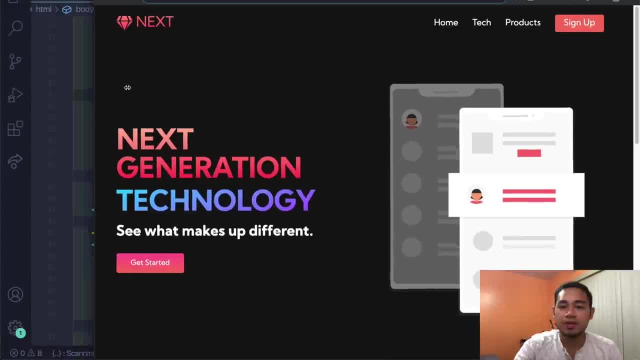 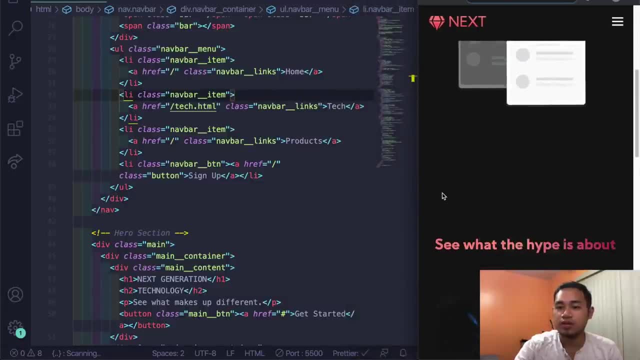 then also if I were to shrink all of this, let me just go up to the top and I'll shrink this And you can see it goes into responsive tablet and then also the mobile, And then I can just scroll down. You can see we have all of our stuff here as well, And then the footer here And then 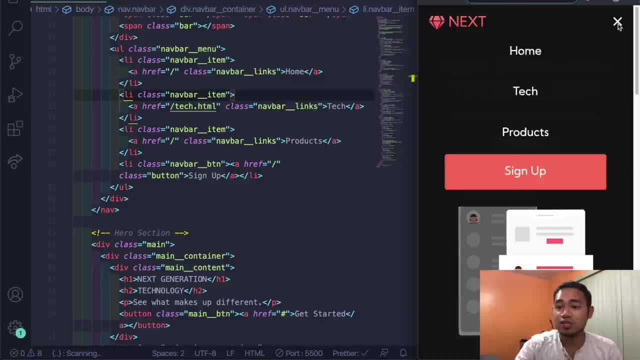 last but not least, the part that uses actual JavaScript is just a couple of lines, but we got a little animation drop down for the menu So you can see there clicking like this. And then, last but not least, the part that uses actual JavaScript is just a couple of lines. 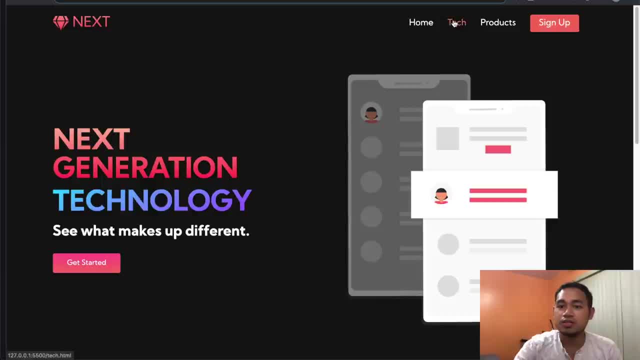 And then also you can go navigate to additional pages and then you can fill in anything you'd like on these pages here, And that's pretty much we're going to make today. So if you want to learn how I did this, then be sure to watch this video all the way to the very end And without further ado. 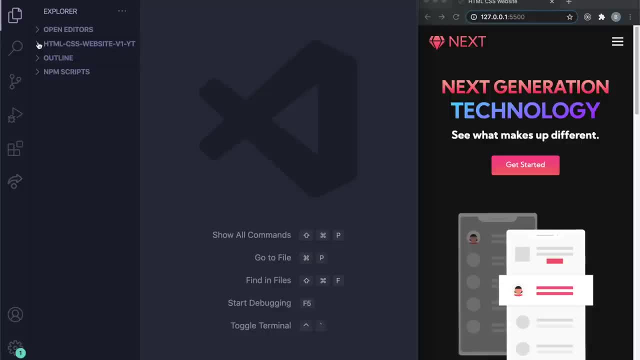 let's hop into my code editor and let me show you how I made this All right. So here I am in my code editor. I'm going to be using VS Code for this tutorial And I already created a folder. So if you have not created one, go ahead and create a folder for your project, And I'm just 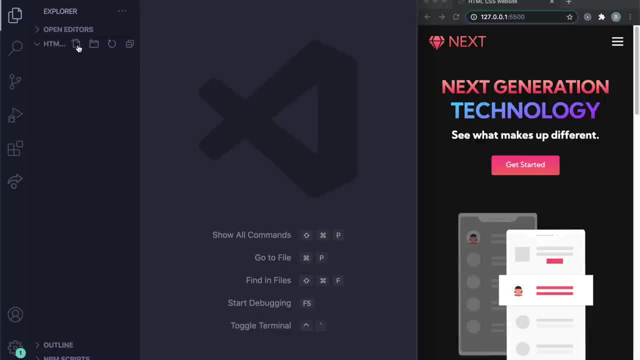 going to click here And then I'm going to go ahead and create a folder for my project And then now I have my icon showing. So I'm going to click on this first icon here And I'm going to create a new file called this, indexhtml. And the next file I'm going to go and create is called 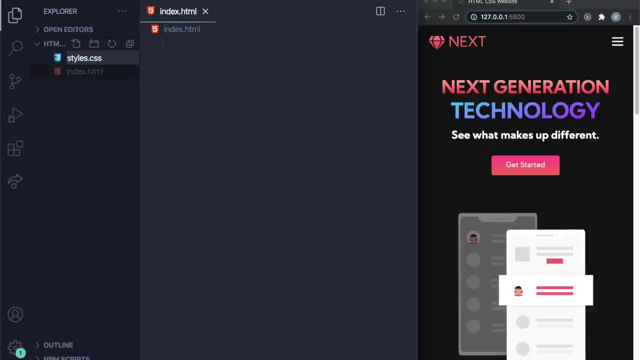 stylescss, And then I'm also going to create an appjs file, So appjs. And then, since we're here already, let's just create a folder, So the second icon, and just type in images, And then last one I'll create is the text. And then I'm going to go ahead and create a folder for my project And 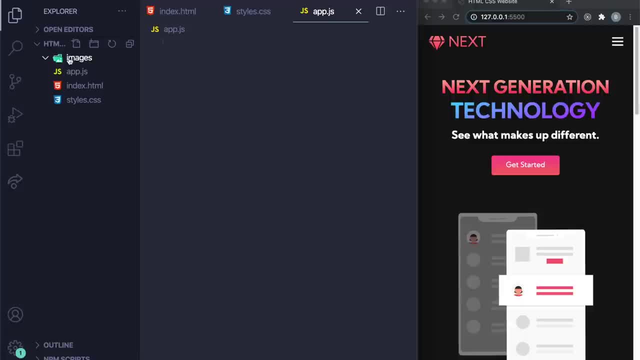 actually let's go outside, Make sure you're in the actual root And then just do techhtml- And this is just to show an example page that we can navigate to- And I'll go into indexhtml And then I'm going to press shift one, make an exclamation mark And then, once I press tab, it'll auto fill. 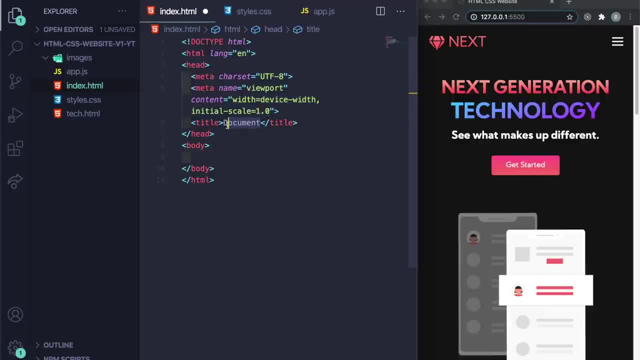 for me. And then boom, we don't have to sit there and type everything out like manually. And then for the tile, let's just say, let's just put like next website Here, And then also under the title, but still inside of this head tag, I'm going to type link. 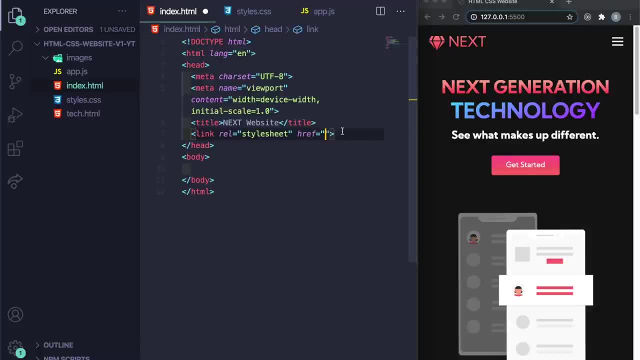 press tab and then automatically types it up for me, And then inside the href I'm going to just add in the stylescss, stylescss, And we can save that by pressing command s on my keyboard. And then in the actual body tag I want to just type in h1 and press, let's say, 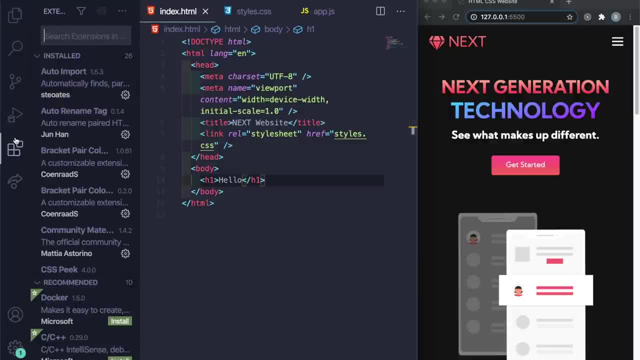 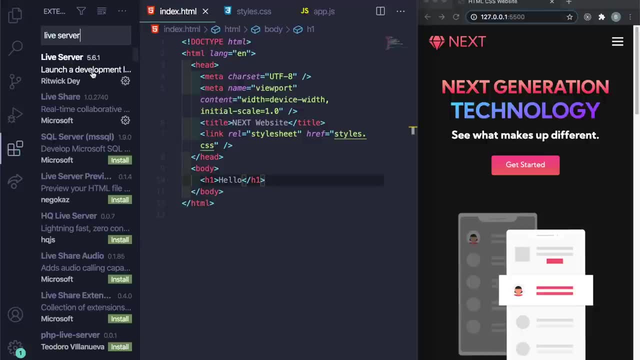 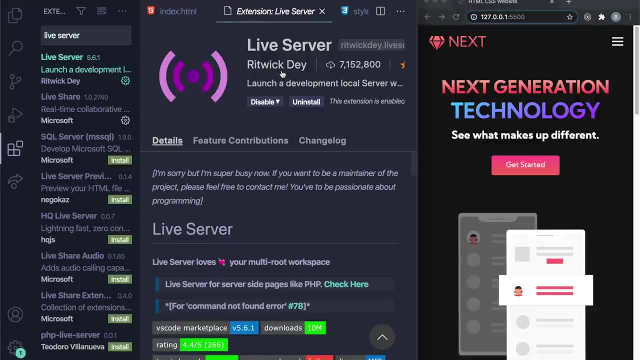 save this. And then also I want to show you some extensions that you need to install. So one is live server, So just go ahead and type in live server And let's see which one we got. This is the one I have right here, live server, and this one by Wigday. And then also, if you don't have, 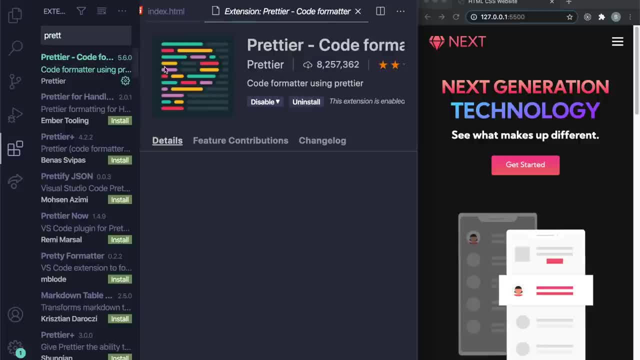 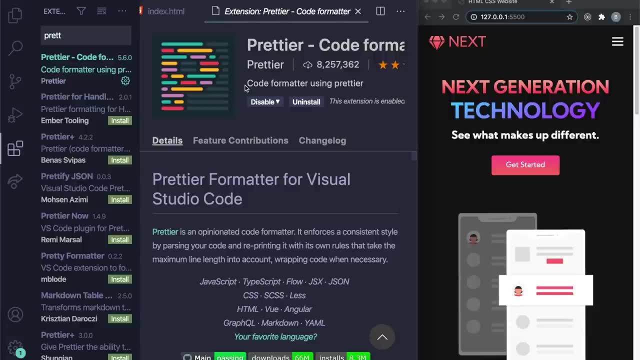 prettier, we just type in right there. This is also another extension I have, So whenever I auto save, it automatically makes my code fit. And then also I want to show you some extensions that I made cleaner. So in case you're wondering, how is that happening and yours isn't? this is one. 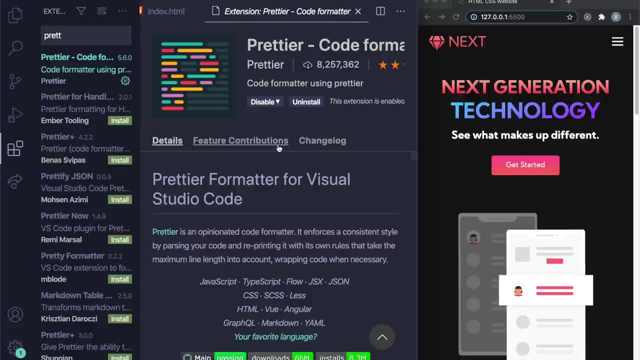 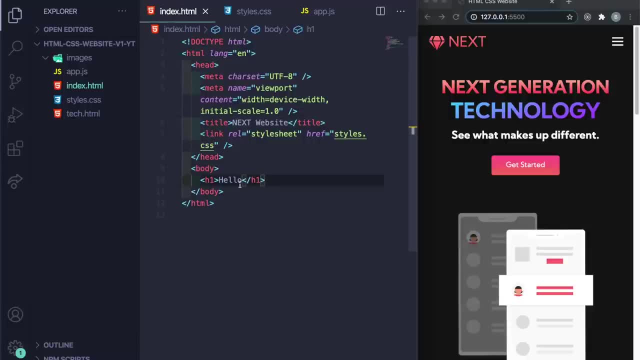 of the extensions I have here, And there's a lot of other customizations you can do as well, but those are just the two ones that you would probably want to have, in case you want to follow along with what I'm doing. So now, before we actually go ahead and load this up, let's go to the stylescss. 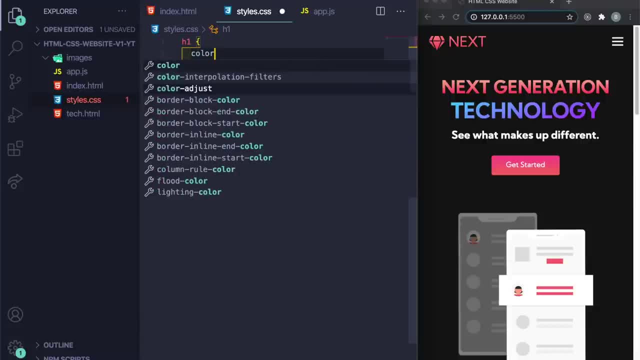 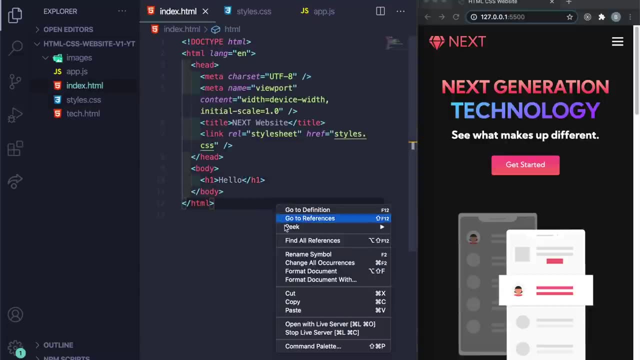 and let's just type h1, curly brace. let's just say color red, just to make sure that everything's working properly. And let's go back to the indexhtml file And then, once you have live server installed, I can just click here: open with live server. 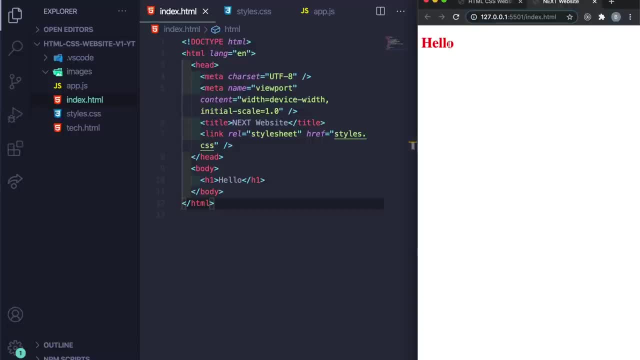 and then this will automatically open up. Perfect, Now we have it right here showing that our website's live. So now I can go ahead and edit this and be like yo, and then perfect, Now everything looks like it's working And notice that once I save it automatically updates. So 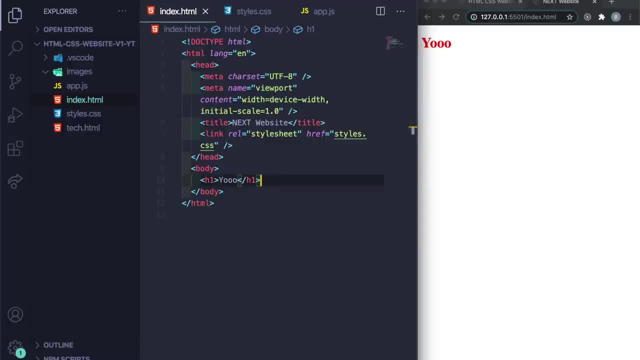 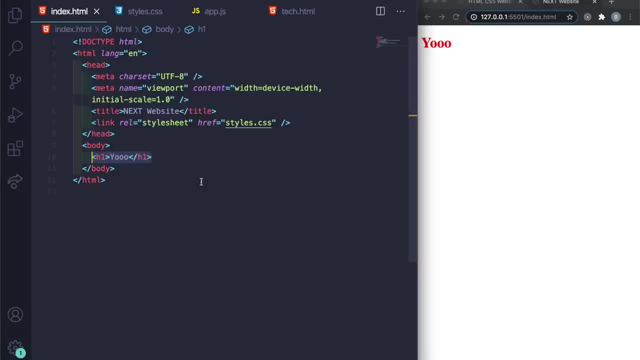 that's pretty cool to have there. And now let's go ahead and actually start adding in our HTML. So the first thing I'm going to do is I'm going to go ahead and add in my HTML. So I'm going to do is actually I'm going to press command B to close out my slide tab. so you can see this better. 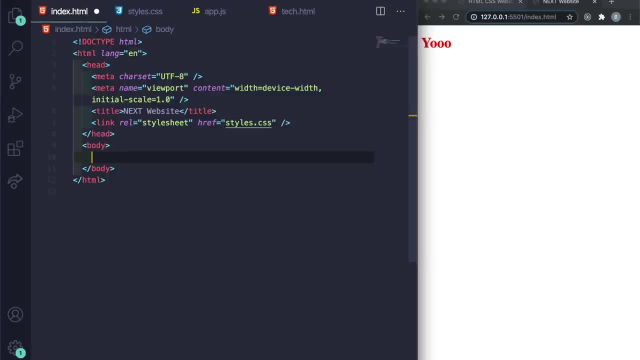 I'm going to erase this h1, and then we're going to create the nav. So I'm just going to create this and let's just do nav, And then I'm going to press dot and then nav bar And once I press tab. 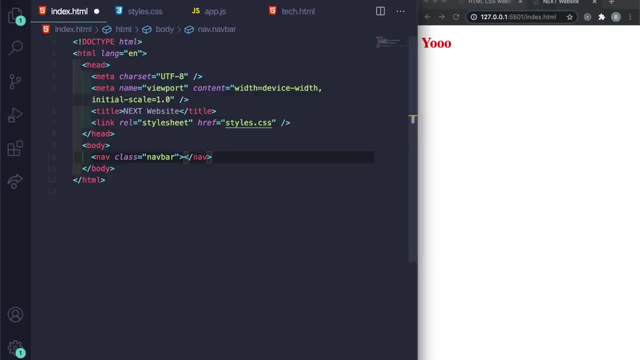 this automatically creates a nav with a class of nav bar, And that's because I have Emmet and it's just perfect like that. And then now under here, let's create a nav bar container. So I'm going to create a div, So for divs you don't have to actually type the word div. So I'm going to create 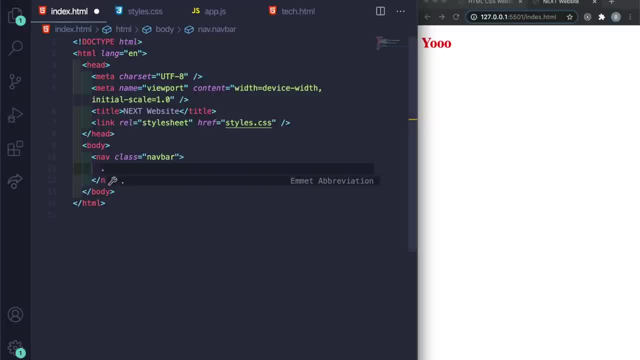 a nav bar container. so you can just type the word div, you just do a dot and then the class you want to name it. So I'm gonna say navbar, underscore, underscore container And I want to press tab. You can see we have a div with the class name navbar, underscore, underscore container, And then 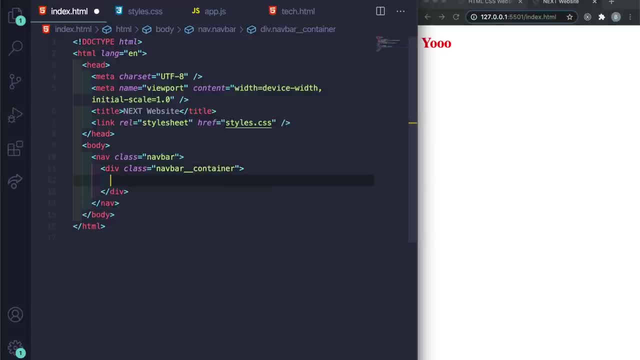 underneath. here I want to create the logo. So ideally you use a page image, but for this example I just hardcore this by typing out the actual words. But here I was going to type in a for the a tag, and then I'm having ID. 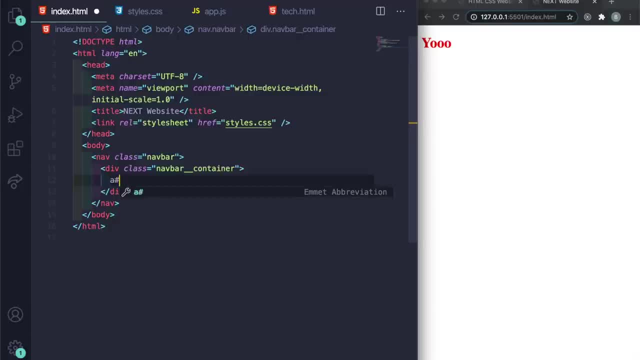 So IDs, you use hashtag, So I'm going to say hashtag and I'm going to say navbar, underscore, underscore logo and then, once I press tab, you'll notice that we have the ID navbar logo and then it has the href. so over here I'm just going to put a slash for that value because we're not linking anywhere yet. 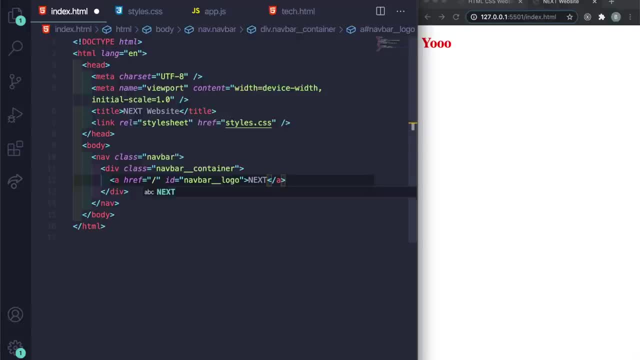 and then in here I'm just going to go ahead and just type in next with the capital letters and then just press save, and now you can see it updates over here. Now, underneath this, a tag, I want to go under it, so press enter and then I'm going to do a div and I'm going to say dot navbar. 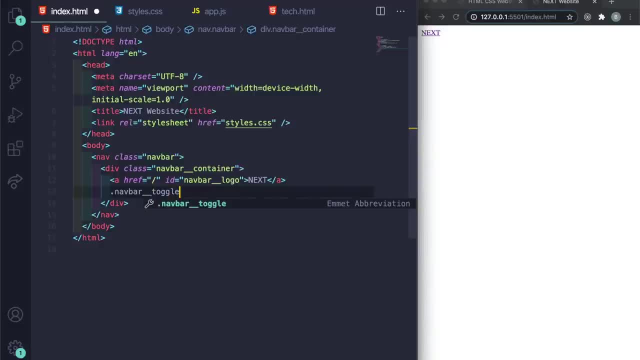 underscore, underscore, toggle. and then I'm going to do hashtag: mobile dash menu. and this is going to be the javascript we're going to be targeting so that whenever we click on the actual icon, it will change from the bars to the x, and I'll just press tab here. and what that did it just? 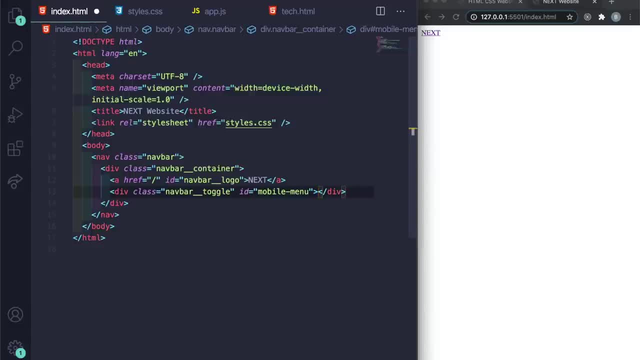 created a class and an id at the same time, and then I'm going to press enter, so now we're inside of this div, and then I'm just going to create a span with the class of bar and do this three times. so I'm just going to say span dot bar. 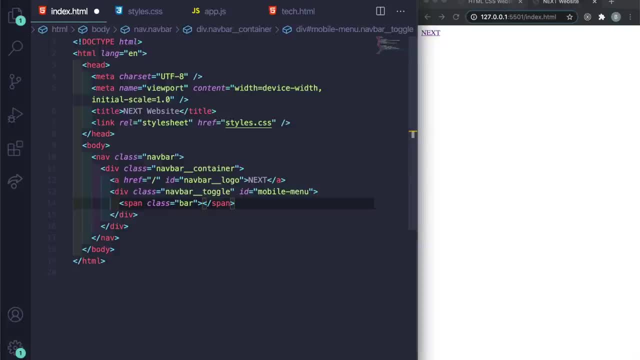 press tab, and this is just me the first bar. and cool little trick you can do: shift, alt and then the down arrow, and then it just copies it down and then do it two more times. so we have three total here. and if that didn't work for you, just simply just copy and paste it three times, like. 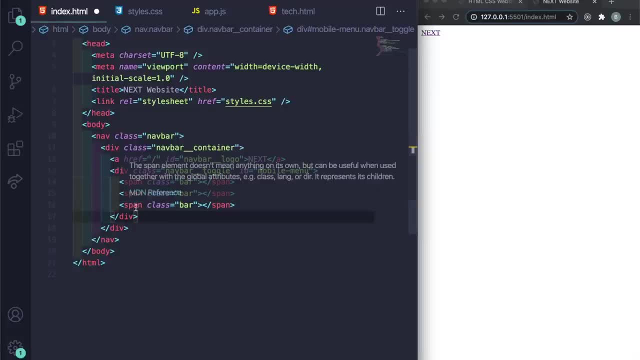 this. and now, outside of this div, right below the span, press enter here. and then I'm going to create a ul with the nav bar menu class name. so I'm going to say ul dot- nav bar- underscore- underscore- menu press tab. so now we're inside of a ul, so I'm going to press enter. and now, inside this ul, I want to create our first. 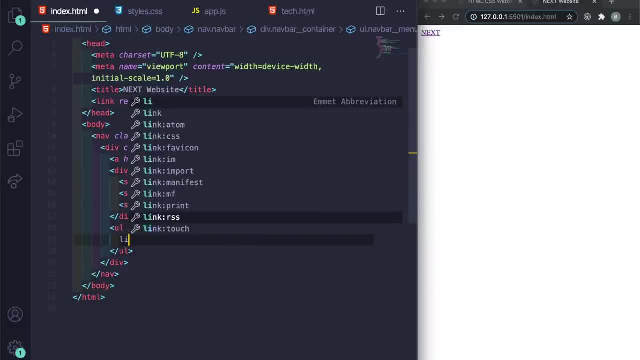 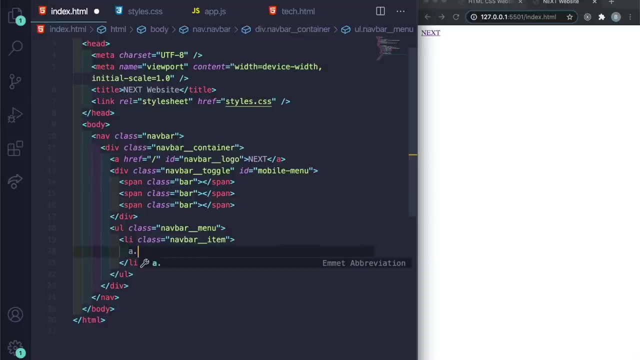 menu item. so this one's going to call it li for the tag, and then the class name is going to be nav bar, underscore, underscore item and I'm going to press tab here, then press enter and now inside this li tag we're going to create the a tag. so I'm going to say a dot and then we'll say nav bar, underscore, underscore links. 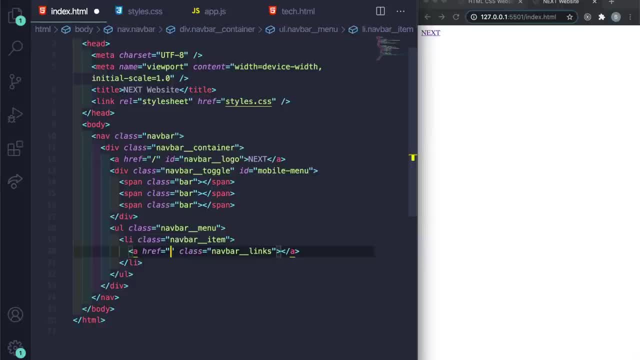 then I'm going to press tab here for the href. let's just put a slash for now and then go inside of this a tag, press, enter here twice, and now I have the space you can see better- and then I'm going to simply have home and then, pretty much, if I save this, it'll. 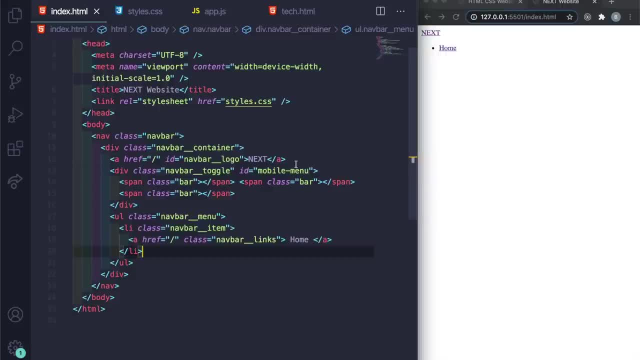 bring it back on the same line here. but now you can see we have essentially a a tag with home. when I click it it just reloads the page because we're going to the slash, and now what we can do is actually just copy and paste this. so I'm just going to take the li tag with the a tag press. 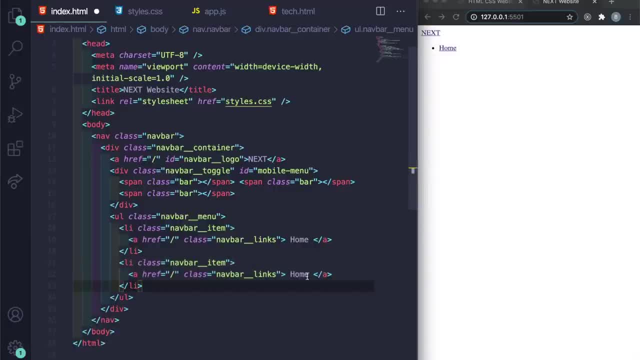 enter under paste it once, and then we can change this one to: let's do tech, and then here I'm gonna put tech dot html and press save. so now what this is going to do. since we have a tech dot html page, we just simply click it and now you can see in the actual address bar that it has the tag that html, and there's. 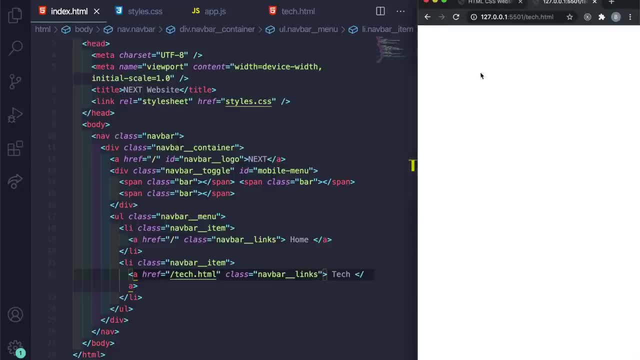 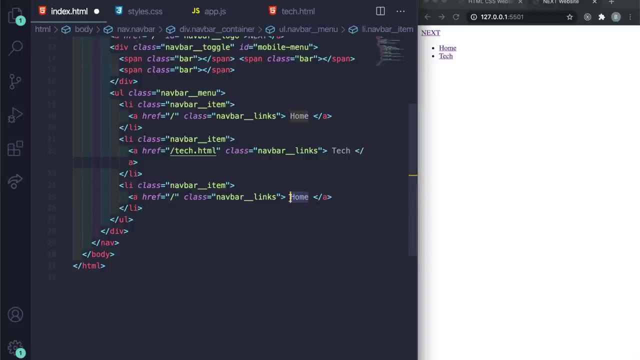 nothing showing because we currently have nothing on the actual tag, that html page, and then let's go back here, and then let's simply go under the li that we just copied. let me scroll up here, but just paste this again, and let's just change this to: let's do a tag with home, and then let's just 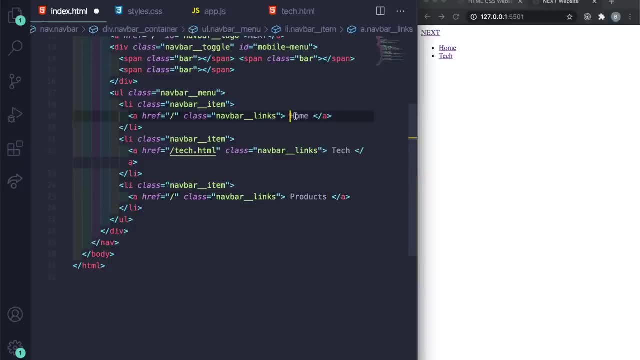 do products. and for this, for my thing, you don't, the spaces doesn't really do anything, but I'm gonna, for my reason- mine's like saving with spaces, but yours probably doesn't have that- and then, underneath this l, I'm gonna do command v again, so pasting it one more time, and except for the last, 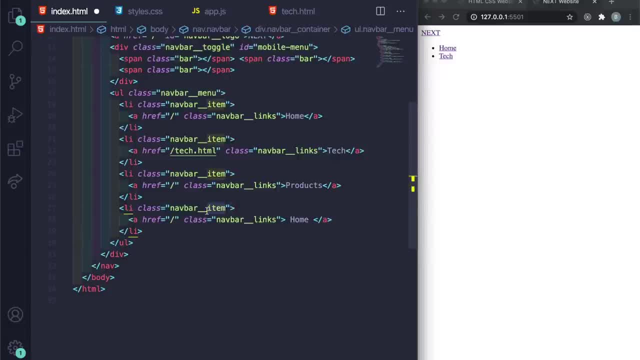 one. I'm going to change this from navbar item to navbar btn and then also navbar, and I'm just going to put this as: take that class completely out and just straight up say button. and then here let's erase this word home, let's just say sign up, so we can save that there. and now we have our central nav menu. prior to styling. so now let's. 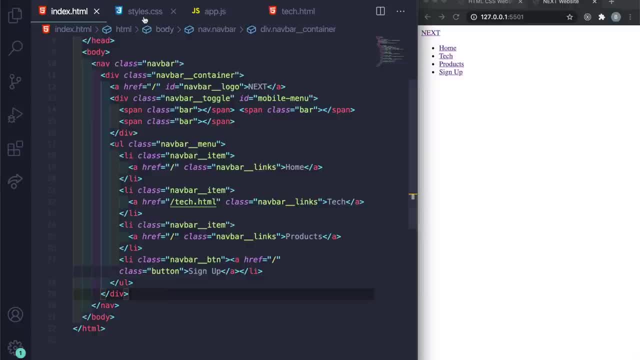 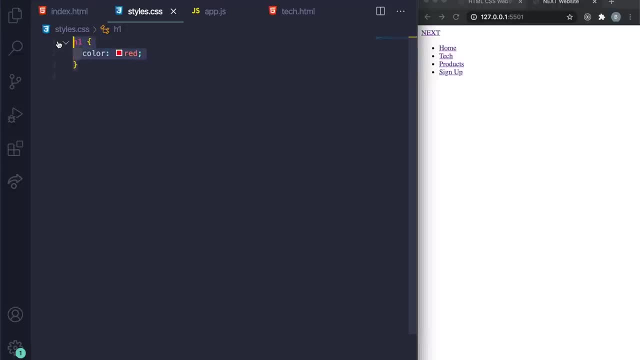 actually go into stylescss. so I'm gonna command b here and let's go to stylescss here and let me close out the side. you can see better. let's just cross this out, and now let's do the first thing. so I'm gonna have a little. 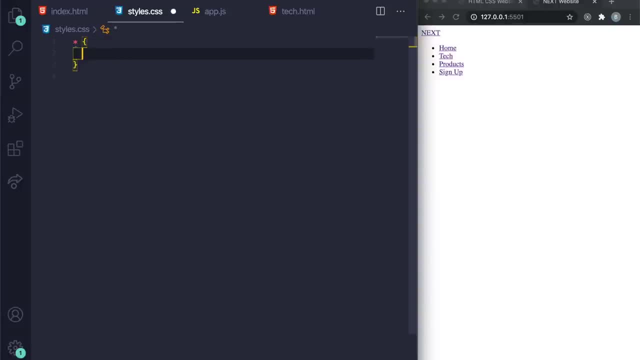 shift 8 symbol, little time symbol, curly braces, enter. and then I'm gonna say: box sizing, border box, and then I'm gonna say margin to be colon zero, padding to be zero, and then I want the font family to be k-u-m-b-h, sans comma, sans serif, and if I 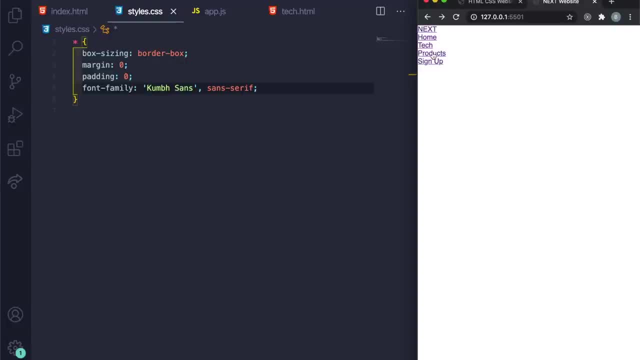 save this. right now we can see that our change, our text has changed, but we will have to import this from google fonts. but I'll do that in a little bit. for now I'm just going to finish up the actual navbar. so now let's target the actual navbar class. so dot navbar, curly brace I want to set. 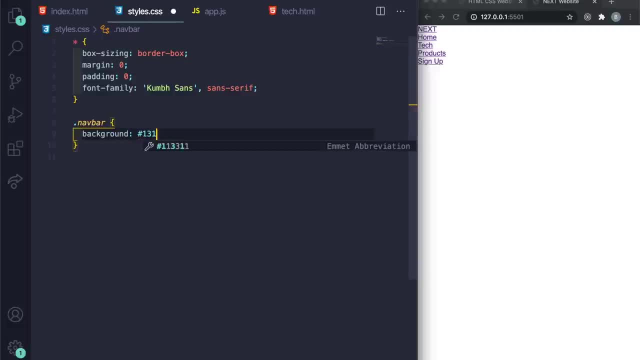 the background to hashtag one, three, one three, one three, and then I want to set the height equal to 80 pixels. then I'm going to say display flex, and what this is going to do is going to be a little bit for the text we're going to create. a line that's going to do is make it like this. now let's just 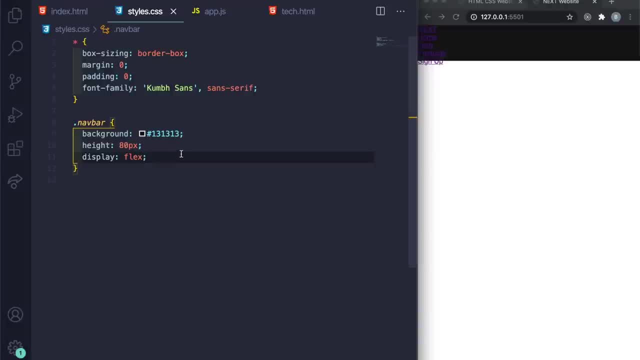 create the line. so this is going to be a little bit of a redefining, and then I'm just going to give this a name. it's going to be like this with this circle. so that's going to look like this. so I'm going to give it a little bit of a different name on it. so let's say: define collection. 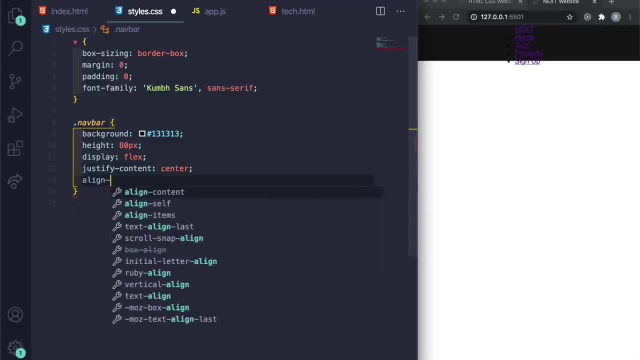 you want to do that, because you know I'm going to do all of these. like you can go over there and type a number or anything you want to put in there and do. that's going to bring a little bit older than this, because I'm going to save this now. you can't really see it yet, but let me just go ahead. 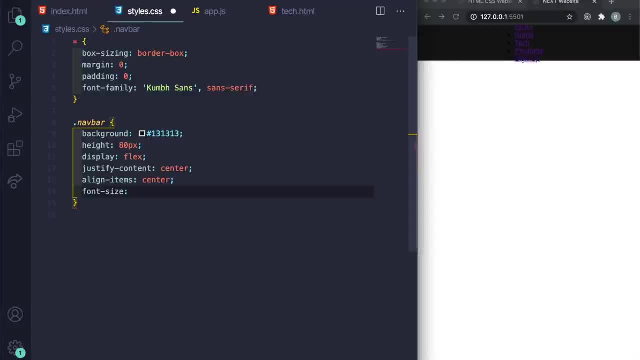 and just do justify content center, so now you can see. it moves it over here and then align dash items. essentially one ram is equivalent to 16 pixels by default, but if you were to change the initial value then obviously you can change that. but for now i'm going to do 1.2 ram. so now you can see. 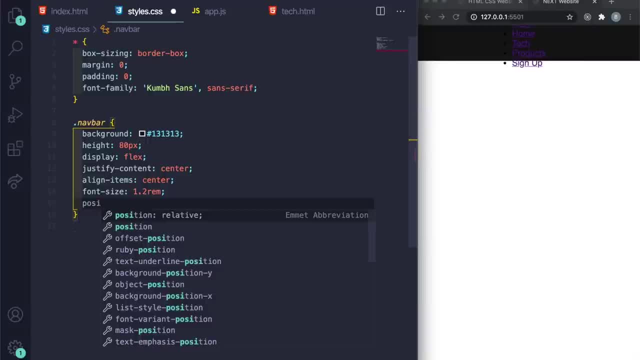 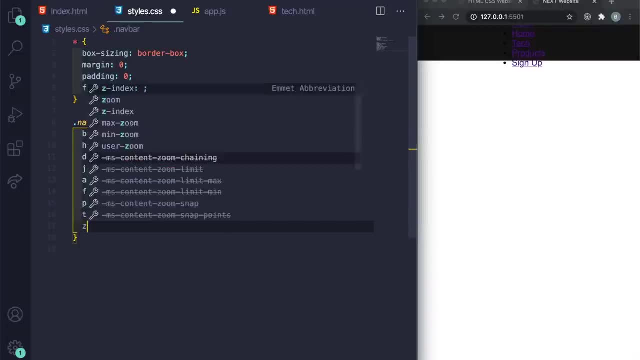 the increase in set size, and then position- let's do just keep it sticky- and then the top. i just want to have a zero. and then the z index, which essentially is- think of this in like three dimensions, in terms of like stacking, and i want it just to be 999, which is just an outrageous 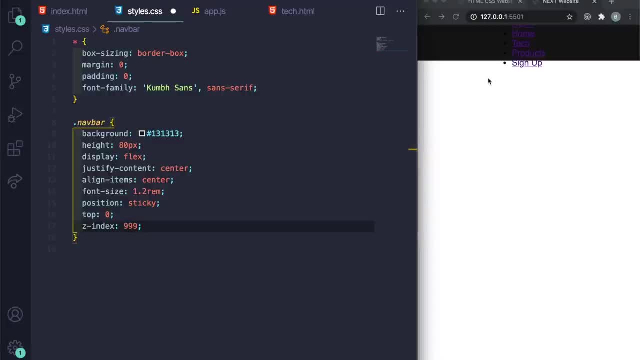 number. but that's to ensure that no matter where i am on my site, wherever i scroll, it will always be above every other part on the website's content. that way it's not blocking, it's not being covered by anything, and then we'll just save here and now. let's press enter and let's do nav bar underscore. 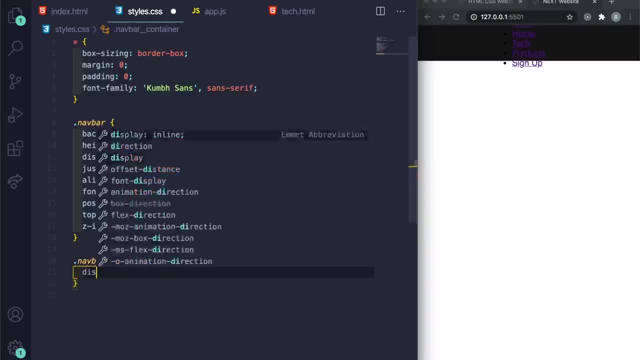 underscore container and i'm just going to say display flex here. so now you can see it moved it to the side and then let's do justify content. i'm going to do space between, so then you won't see how to see yet because it's kind of on its mobile, but once we'll. 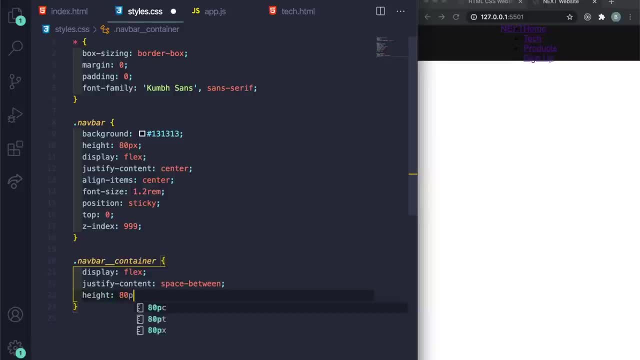 finish this, you'll be able to see everything. let's set the height, let's do 80 pixels here, let's put the z index- just to make it above everything- to one, and let's do width to be 100 and let's make the max width so i don't want it to go past 1300 pixels. 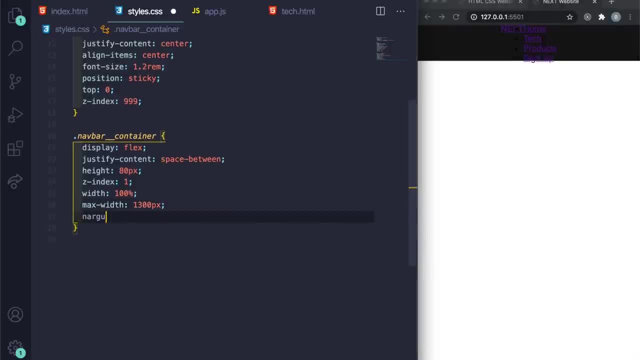 and then let's do margin and let's do right here pretty much colon. and so the shortcut is: if you just do margin instead of doing like margin top or margin right or left, etc. if you do margin the first value is essentially the top and then the second value is right, then bottom and then essentially left. but i want only: 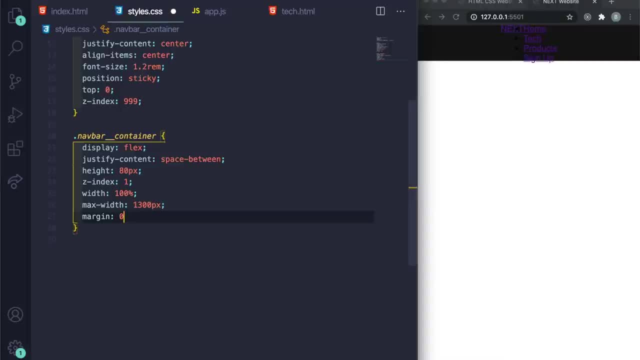 only the top and bottom to be zero. so if you only do two, the first top, the first one does top and bottom and then the second one will do the essentially right and left. so i'm gonna say auto here and then i want to do the same for padding. so i'm gonna say padding and then i want 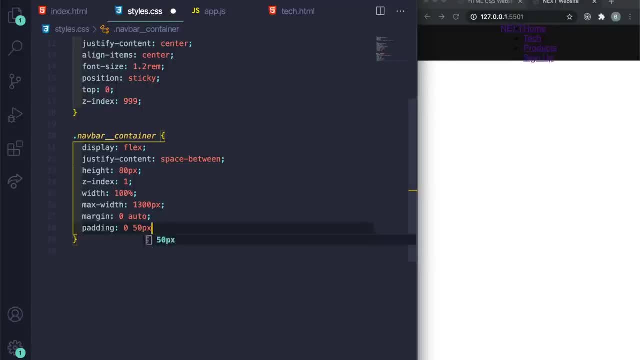 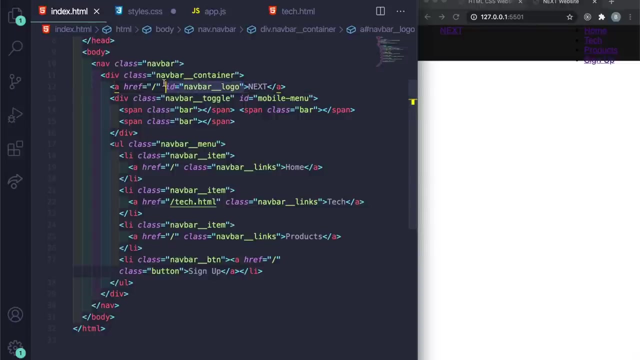 the top and bottom to be zero, and then i want the right and left to be 50 pixels, same here. so now we see some space action going on here, and then let's go ahead and target the navbar logo, and if you remember, that was an id which is: let's see where i put it right here. this one, the next, so 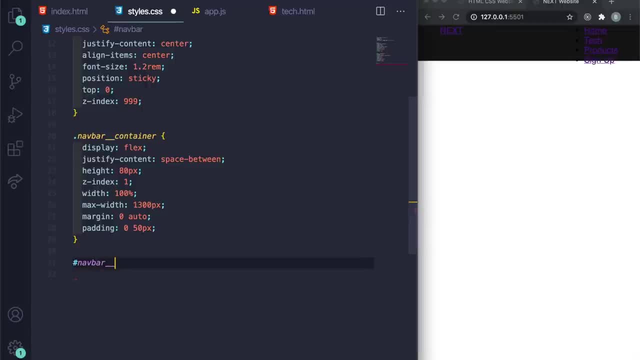 i'm going to do a hashtag, since it's an id, and do navbar underscore, underscore the logo, and then let's do the background, let's set the color, and this is just in case because we have a linear gradient. but in case it failed, well, at least we'll have something, so let's do ff8177. 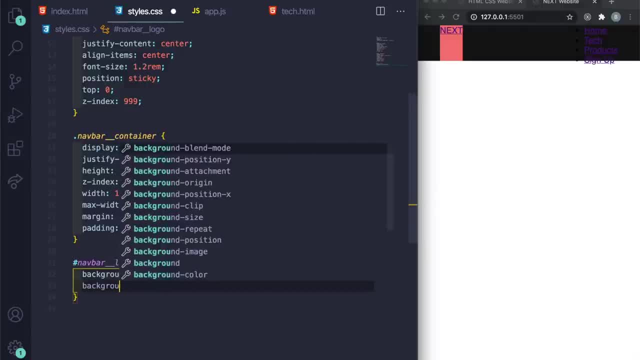 and then let's do background dash image. this is how i got that effect. where the actual logo was a different color, i want to say linear and i have it already auto complete here. so let's press tab, so linear gradient. and then inside here i'm going to say to top. so essentially it's going: 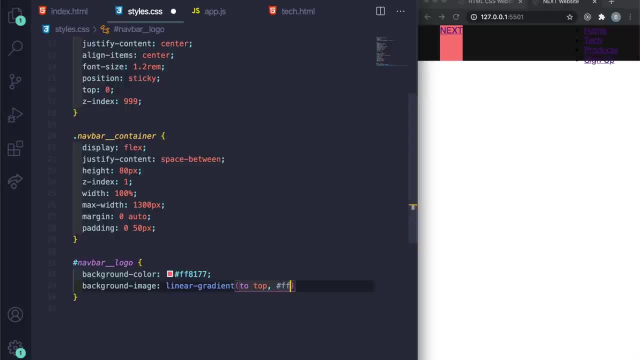 to the top direction, and then i'm going to say hashtag ff0844- that's the color, and then zero percent comma, and then i'm going to say hashtag ffb199 and then a hundred percent, and then i'm going to do a semicolon after this and let's save that there. so now you can see that it's. 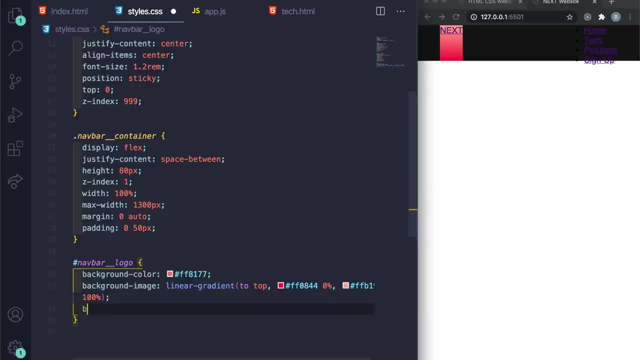 a little gradient effect on the background color. now i want to do background dash size to be a hundred percent, and then i'm going to do dash webkit, dash background clip. i want this to be text and then let me save that there. and then also i want the dash mods, dash background. 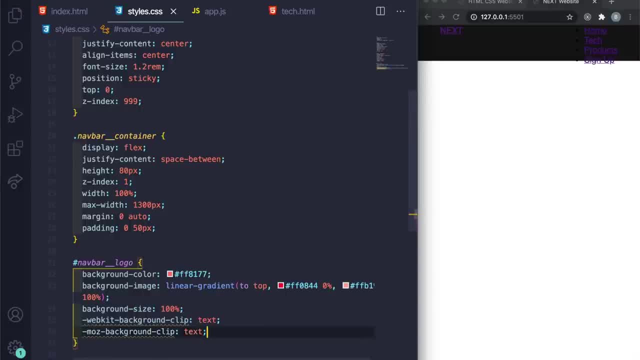 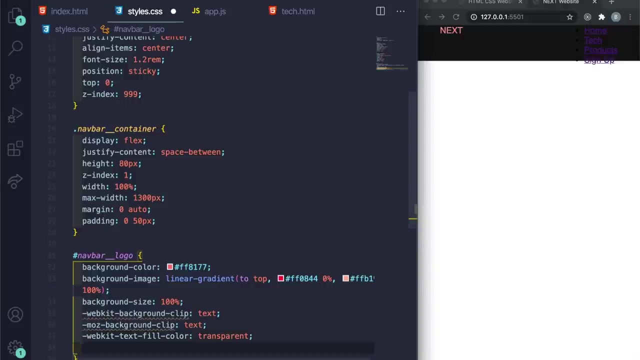 clip. i want that to be text as well, and then under here i'm going to do webkit dash text: dash fill, dash color to be transparent. so now you can see it shows up, and then samby dash mods dash text: dash fill, dash color to be transparent as well. 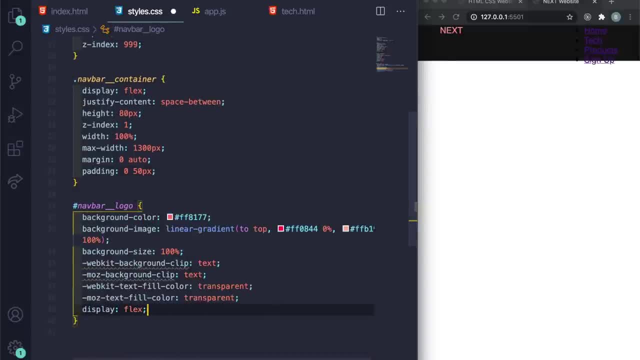 and then under there, i'm just going to say display flex, and we're going to add an actual icon from font awesome. so this is where it's going to make it even, but right now, since we don't have it, it won't really make sense. but you'll be able to see this. 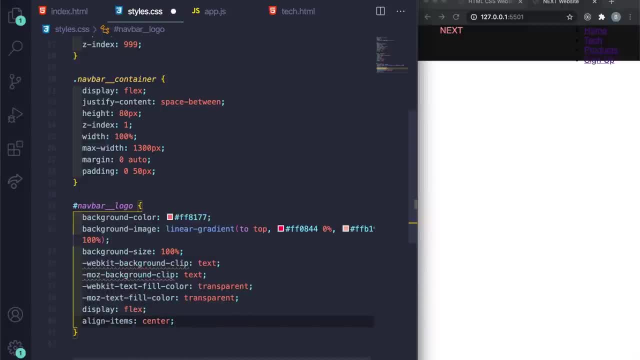 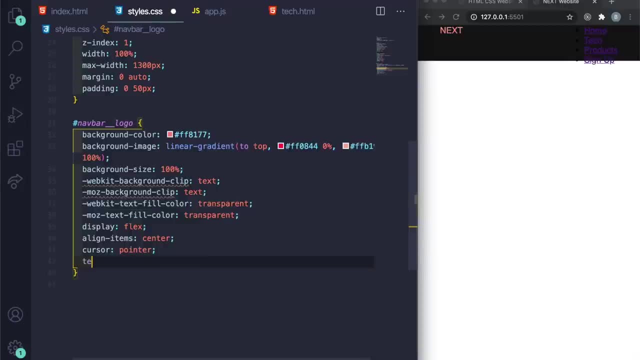 after let's do align items. to be center cursor. i want it to be the pointer, so it has a little hand symbol when i hover over it. and then let's do text decoration to be none. i should see text decoration get rid of the underlines. it's an a tag, and then let's do. 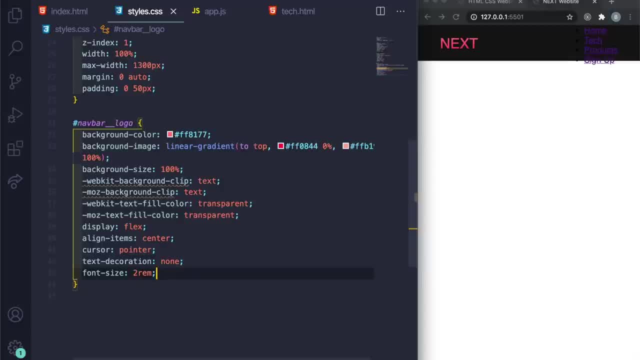 a font size of two rem so you can see you got a little cursor when i hover. and then underneath this we're gonna have the actual icon. so let's just- i'm gonna add it right now. let's just say the class is going to be called fa-gem and it's gonna be curly braces, and i just want the margin. 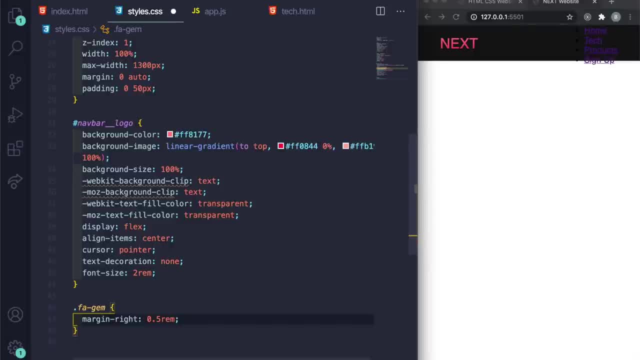 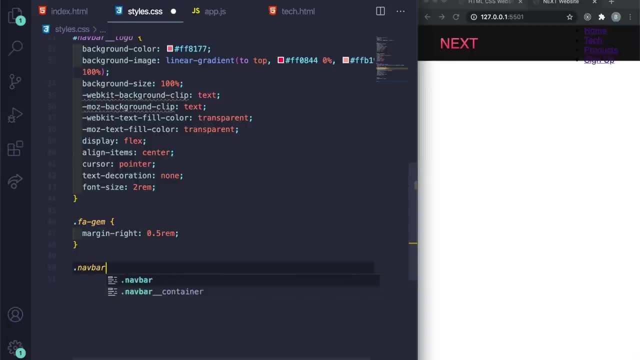 dash right to be 0.5 ram. so we haven't added this yet. but once we go and add it it'll automatically be updated with the css and the under. here let's do dot nav bar, underscore. underscore menu: curly brace, here i'm gonna say display flex. 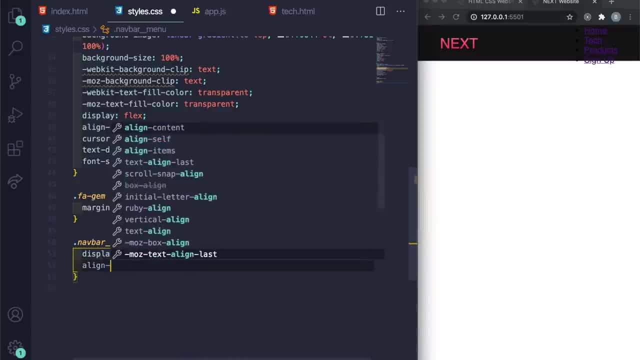 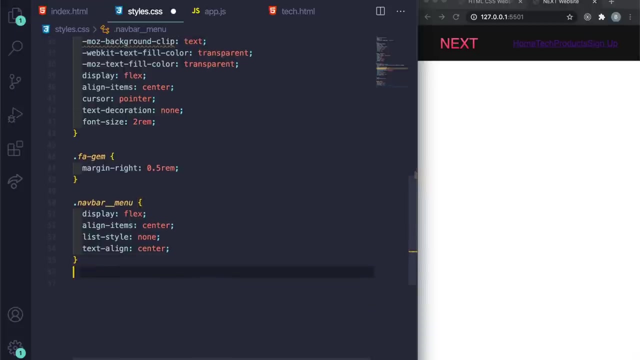 and then i'm gonna say align items to be center. then i'm gonna do list style: i want that to be none and then i want text align to be center. so now you can see our little nav menu items changed, and then let's do dot nav bar underscore. underscore item. 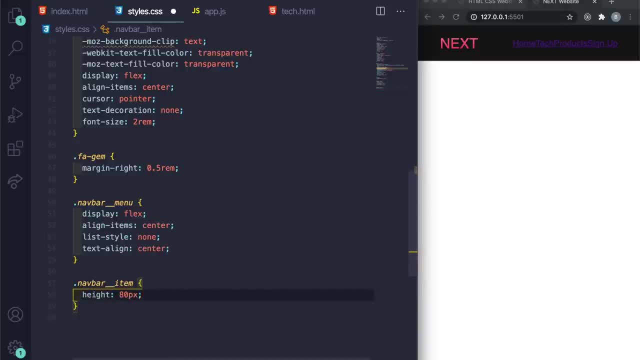 so let's do a height of 80 pixels and then under that let's go ahead and target the nav bar links. let's just do dot nav bar, underscore, underscore links and then curly brace here and let's change the color. let's make that to white, so hashtag fff and let me see if you can see that. and then let's do under right here: let's: 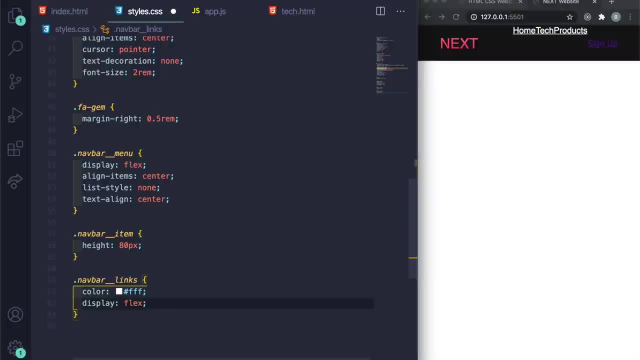 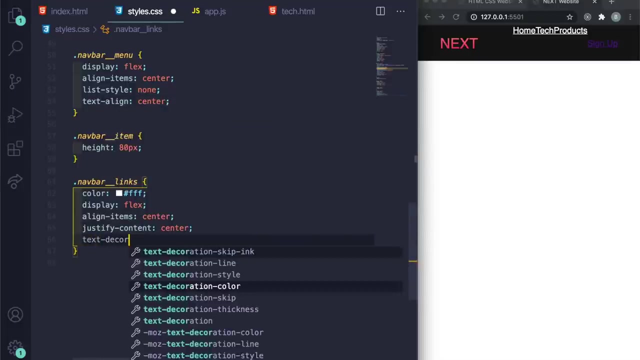 do display, flex, align dash items to be centered, and then let's do justify content. i want that one to be center and then let's do text decoration. let's put that as none and then let's do padding. i want that top and bottom to be zero and then the left right to be one rem, and then let's set the height equal to. 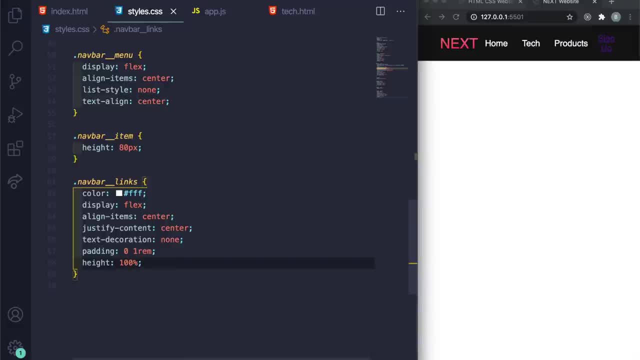 100 percent. so now you can see it's starting to look a little better. and now let's target the button now. so navbar, underscore, underscore btn and curly brace here, and i want this to say: display flex. then i want justify: content to be centered, then i want align. 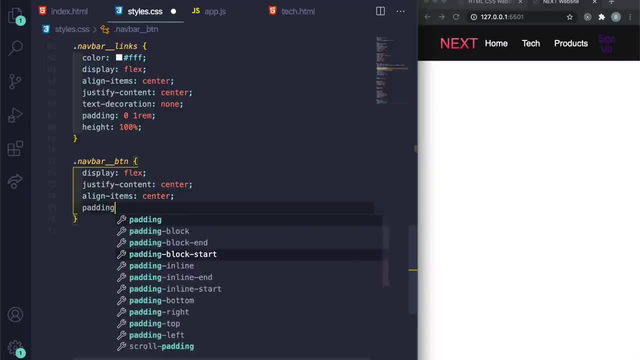 items to be centered. and then let's do padding zero and then one rem, and then let's do width to be a hundred percent. and they didn't do much yet. but let's go ahead and now target the actual dot class, dot button. and now let's do display, let's do flex, justify content center, let's do 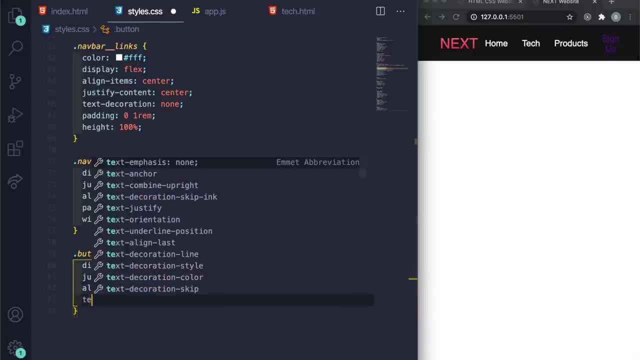 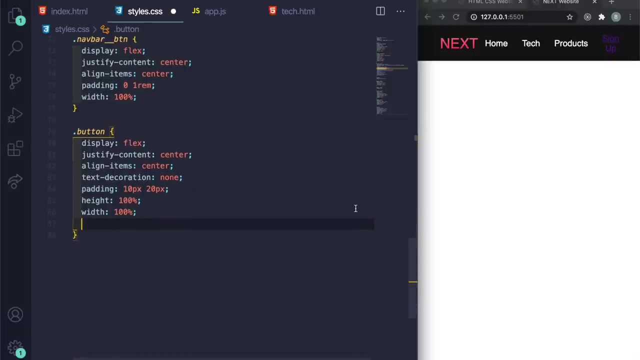 align items center text decoration to be none, and then let's do padding: 10 pixels by 20 pixels, let's set the heights to a hundred percent, the width to a hundred percent and let me just scroll up really quick- and let's do border to be none, outline to be none and then border dash radius. 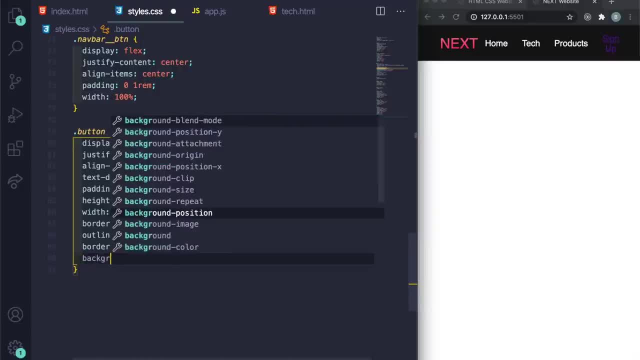 to be four pixels, and then i want the background to be hashtag f, seven, seven, zero, six, two, and then i want the color of the text to be just hashtag fff, which is simply white. and now you can see we have some button action going on here, and then, when i scroll it out, we have it like this and: 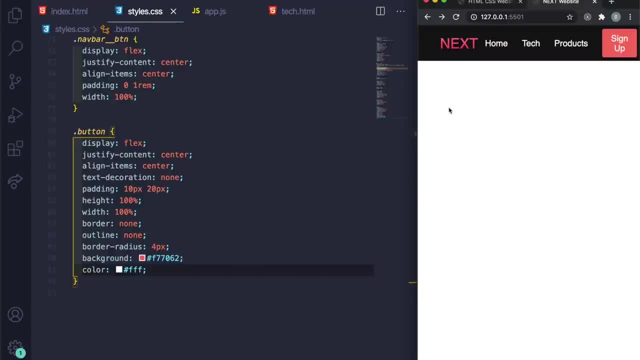 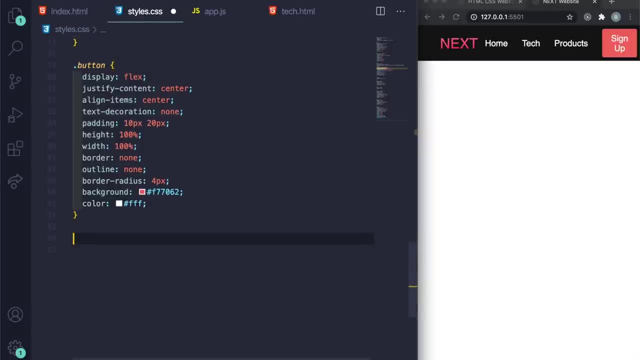 whenever we shrink it, the that's going to disappear because the hamburger menu is going to pop up. but that's what we got going on right now. and now let's finish up our nav menus. let's just do dot button and to do a hover effect, you do a colon and then say the word hover and then curly. 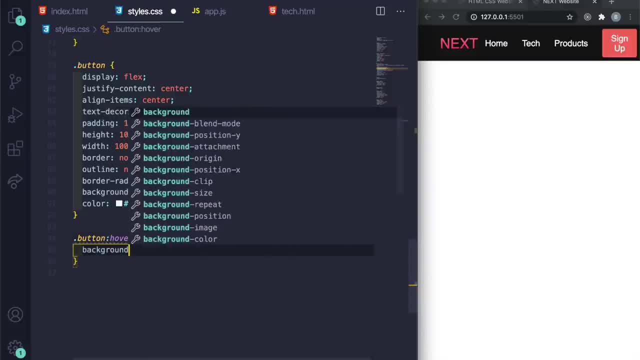 brace under, and then simply let's just say background, let's do hashtag four, eight, three, seven, ff, and then transition. so instead of being it like instantly, i want it to be delayed. so i'm gonna say all 0.3 seconds. and then let's just say ease and it's like i misspelled transition, so transition here. 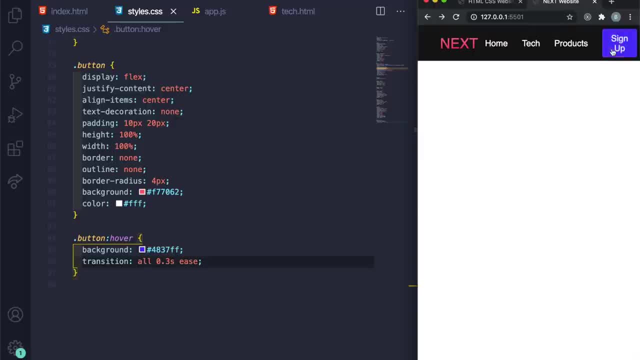 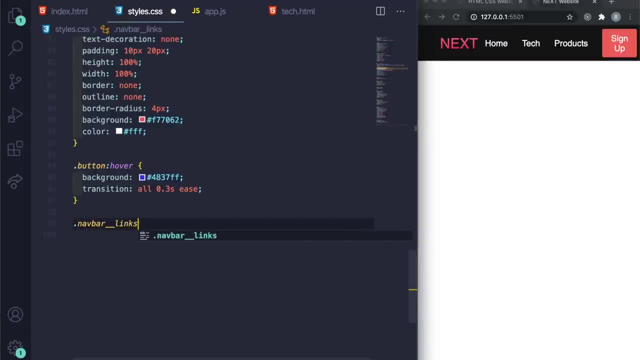 save. so now, you see, we hover over it. we got something going and now let's do the last hover. so basically i'm gonna do the last one here and then i'm gonna hover over. so let's do this, and then i'm gonna set the color equal to hashtag f77, zero, six, two, and then transition is just going to be. 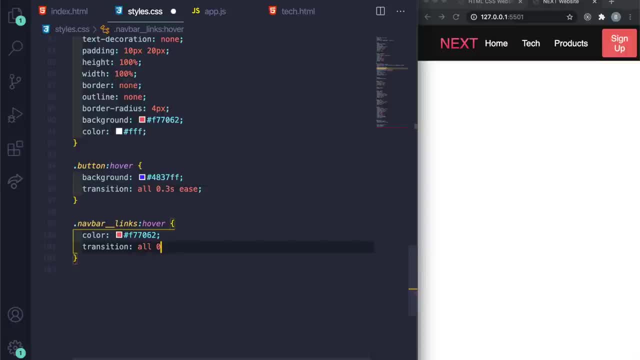 the same exact thing: all 0.3 s e's. so now if i hover over the nav links, we got cool orangeyish looking effect right there. now let's do the actual mobile responsive, tablet responsive part, which is media query. so essentially it's just a massive table of responsiveness that we have here in the 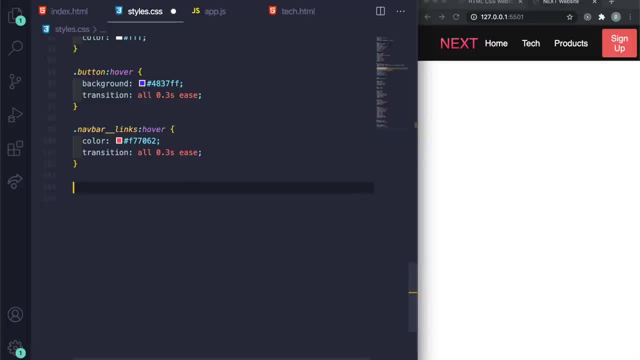 digital calendar for this project. you can see that we have a whole site of media queries here in the for that. you just type in at media and then say screen and, and then parentheses and then max dash width and essentially right. when this hits 960 pixels is when i want to trigger these classes. 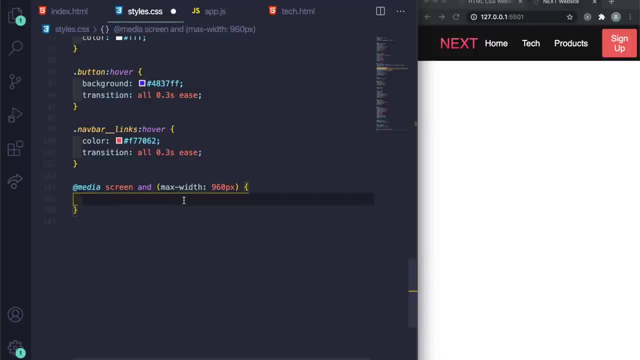 so first thing i want to do is do the nav bar. so let's just say dot nav bar, underscore, underscore container. and then here i'm going to say display flex, justify content to be space between. and then for the heights, let's set that equal to 80 pixels. z index: 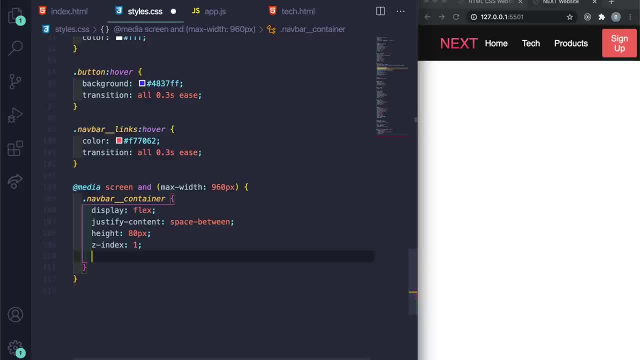 to be one, let's do the width to be a hundred percent. max width, let's do 1300 pixels and then padding: let's set that equal to zero. so underneath here let's do max width. let's do 1300 pixels and then padding: let's set that equal to zero. so underneath here let's do. 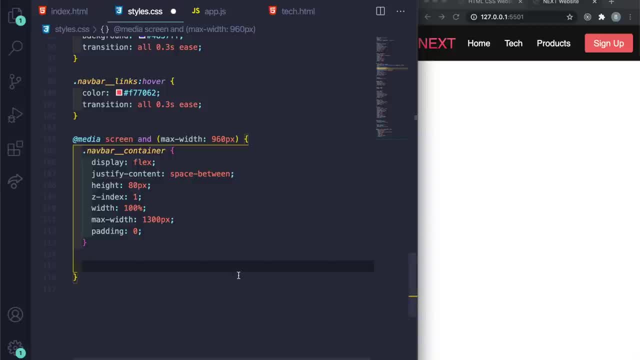 max width: let's do 1300 pixels. and then padding: let's set that equal to zero. so underneath here the nav bar menu. so let me just simply go and say: dot. nav bar, underscore, underscore menu. curly brace, let's do. display grid, let's do grid. templates, columns. 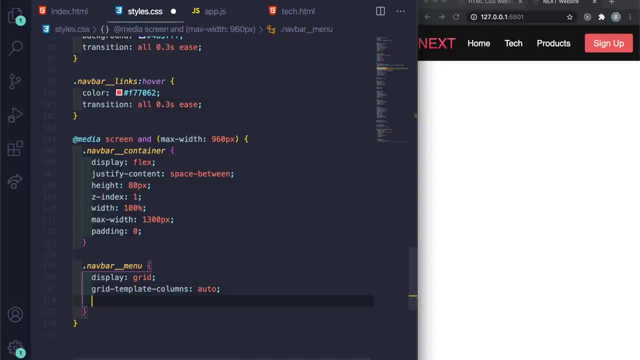 i want to set that value to auto, and then let's set the margin equal to zero, let's set the width equal to 100 percent, and then let's do position, and then let's do position absolute, and let's set the top, and i'll absolute. and let's set the top and i'll. 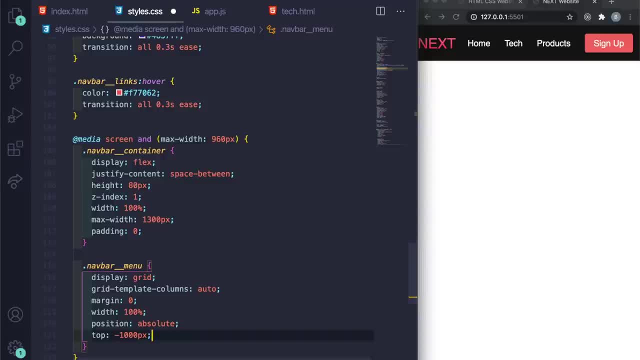 absolute and let's set the top and i'll say equal to minus, say equal to minus, say equal to minus 1000 pixels. so if you saw in the previous 1000 pixels, so if you saw in the previous 1000 pixels, so if you saw in the previous one, 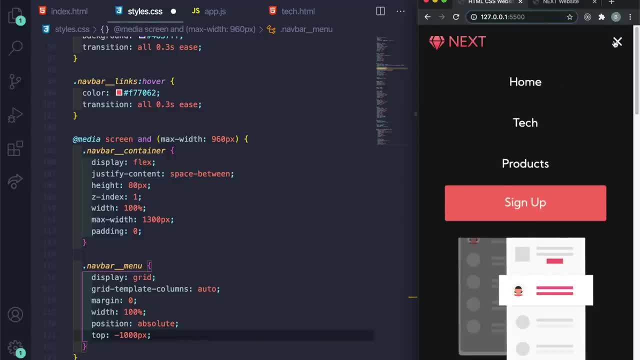 one one. essentially the animation is coming from. essentially the animation is coming from, essentially the animation is coming from the top, the top, the top, so the top. i said to negative a thousand. so so the top. i said to negative a thousand. so so the top. i said to negative a thousand. so just ensure that it's never going to be. 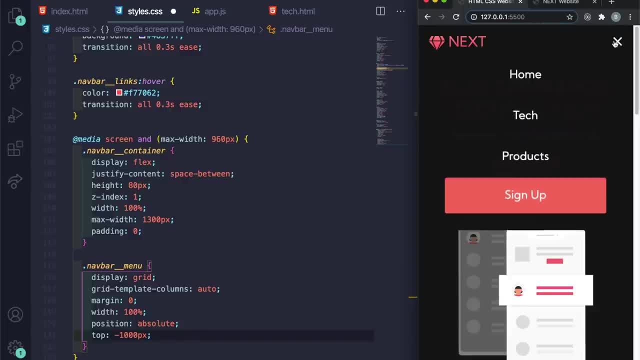 just ensure that it's never going to be, just ensure that it's never going to be seen, and then, whenever i click it seen, and then, whenever i click it seen, and then, whenever i click, it essentially sets the top back to, essentially sets the top back to. 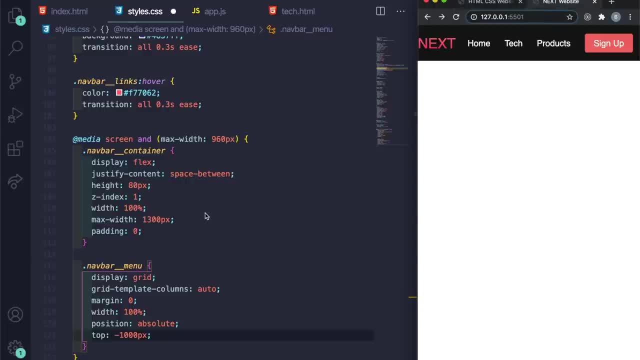 essentially sets the top back to a value, to where we can see it. so a value to where we can see it. so a value to where we can see it. so here, that's what we're doing right now. here, that's what we're doing right now. 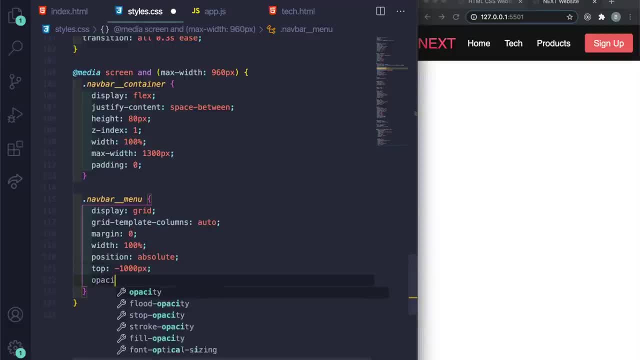 here. that's what we're doing right now: this code, this code, this code, and then under let's do opacity to like, and then under let's do opacity to like, and then under let's do opacity to like to one to one to one, let's transition. 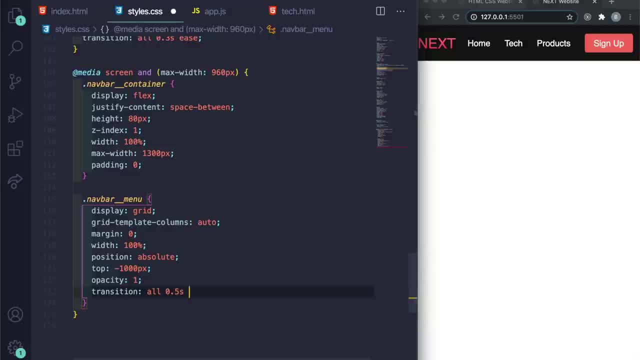 let's transition, let's transition. let's set that equal to all 0.5. let's set that equal to all 0.5. let's set that equal to all 0.5. s east actually. let's set the opacity to s east. actually. let's set the opacity to. 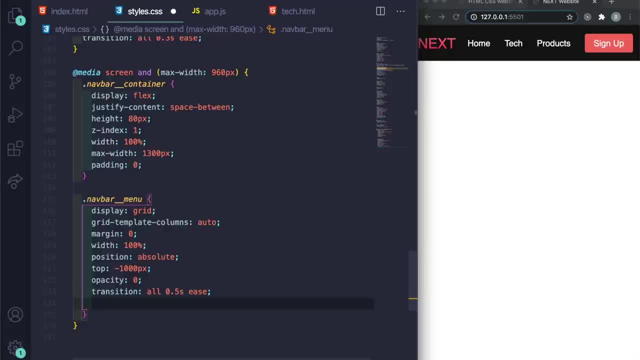 s east. actually, let's set the opacity to zero, zero, zero, because i don't want to be seen, and then because i don't want to be seen, and then because i don't want to be seen, and then let's do the heights. let's do the heights. 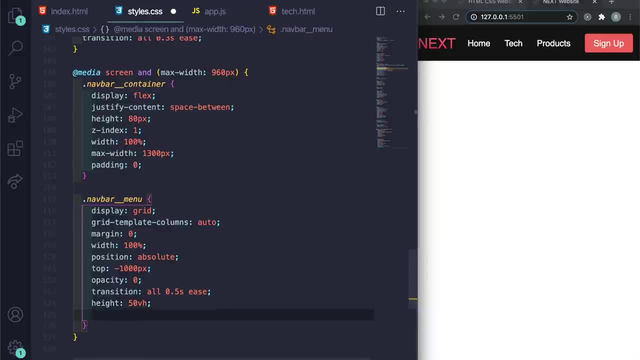 let's do the heights of 50 v h, of 50 v h, of 50 v h, so that means viewport height, and then so that means viewport height, and then, so that means viewport height, and then z index: you have to set it to negative. z index: you have to set it to negative. 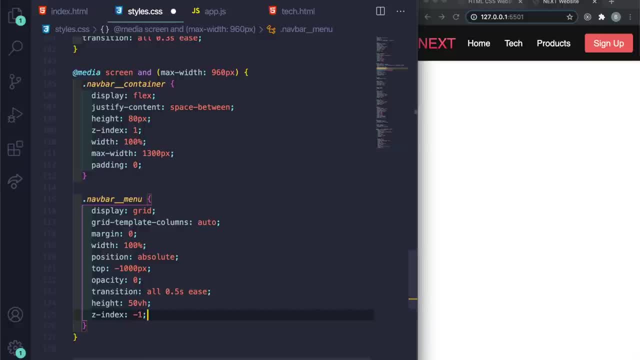 z index, you have to set it to negative one, just so that we actually be able to one, just so that we actually be able to one, just so that we actually be able to click on the icon to trigger this. click on the icon to trigger this. click on the icon to trigger this. so now you can see that nothing is. 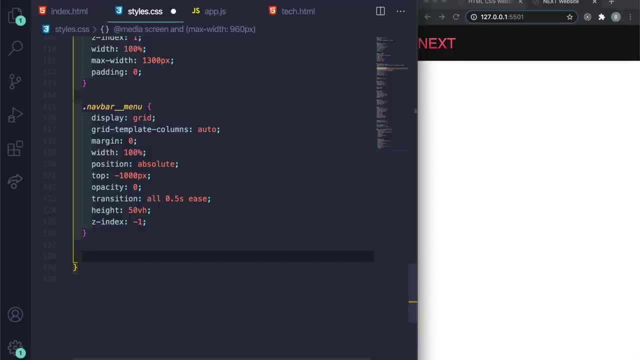 so now you can see that nothing is. so now you can see that nothing is showing, showing, showing. so now we're going to have the navbar. so now we're going to have the navbar. so now we're going to have the navbar. menu- active class menu- active class. 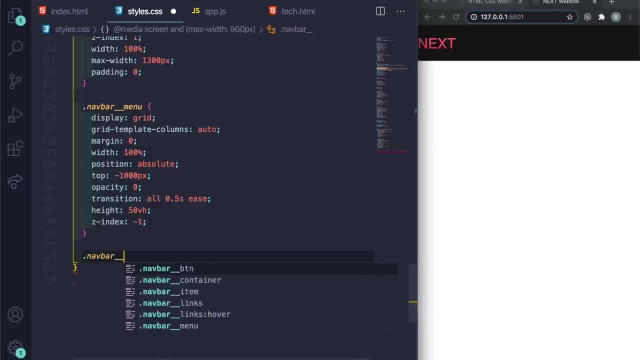 menu active class. so dot navbar underscore- underscore. so dot. navbar underscore underscore. so dot navbar underscore underscore- menu dot active. so this is going to be menu dot active. so this is going to be menu dot active. so this is going to be the javascript that's going to trigger. 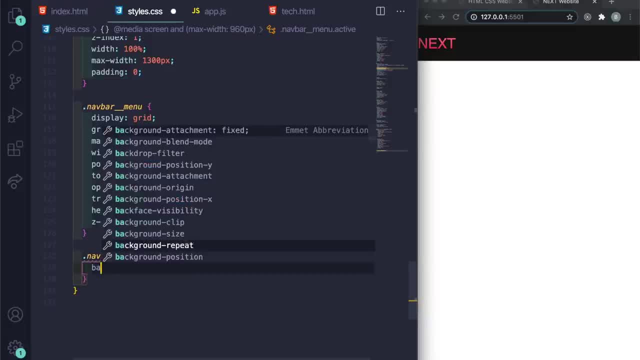 the javascript that's going to trigger, the javascript that's going to trigger this, this, this and essentially, whenever we click it, and essentially whenever we click it and essentially whenever we click it. this one, i want this to trigger, so i. this one, i want this to trigger, so i. 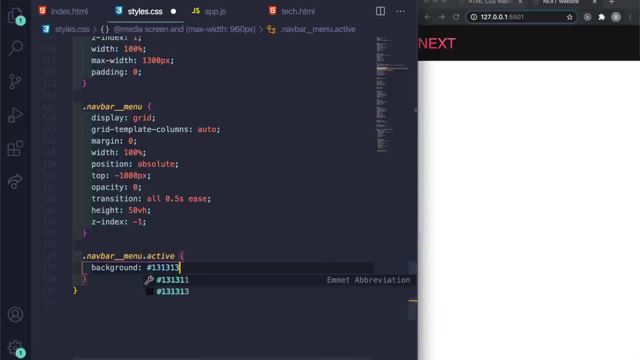 this one. i want this to trigger, so i want to set the background equal to this one. i want to set the background equal to this one. i want to set the background equal to hashtag, hashtag, hashtag. one, three, one, three, one, three, and then i. one, three, one, three, one, three, and then i. 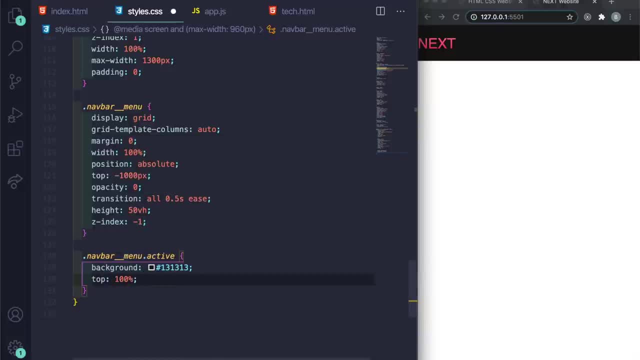 one, three, one, three, one, three. and then i want to set the top equal to 100, want to set the top equal to 100, want to set the top equal to 100. so this value, right here, is going to. so this value, right here, is going to. 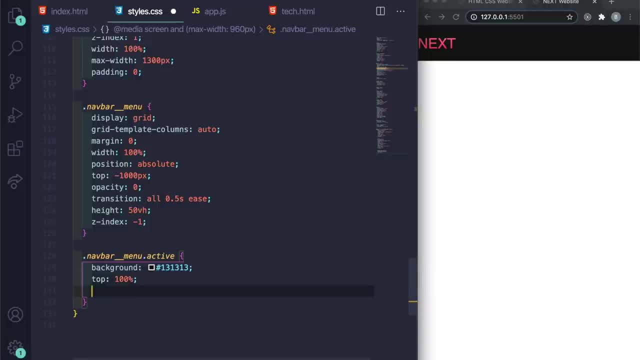 so this value right here is going to essentially show, essentially show, essentially show the entire active menu, the entire active menu, the entire active menu. and then let's set the opacity to one, and then let's set the opacity to one, and then let's set the opacity to one so we can actually see it. 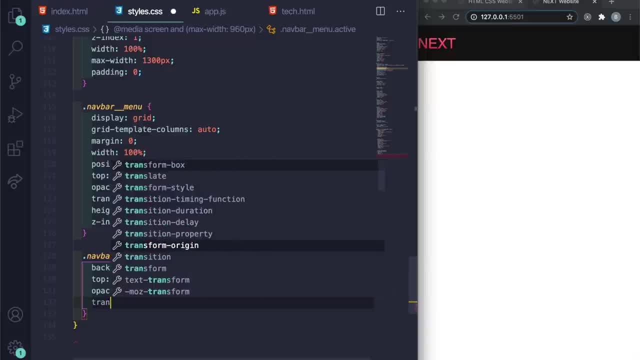 so we can actually see it, so we can actually see it, and then let's do transition, let's see, and then let's do transition, let's see, and then let's do transition, let's see, transition, transition, transition and that's going to be all 0.5. 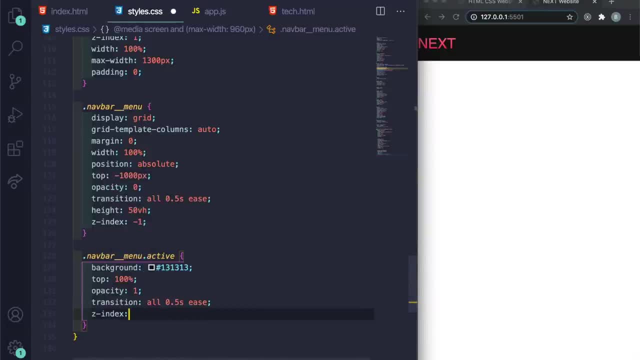 and that's going to be all 0.5, and that's going to be all 0.5 as ease, as ease, as ease, and then let's do z index to be 99, and then let's do z index to be 99, and then let's do z index to be 99, and then set the height again to 50 vh. 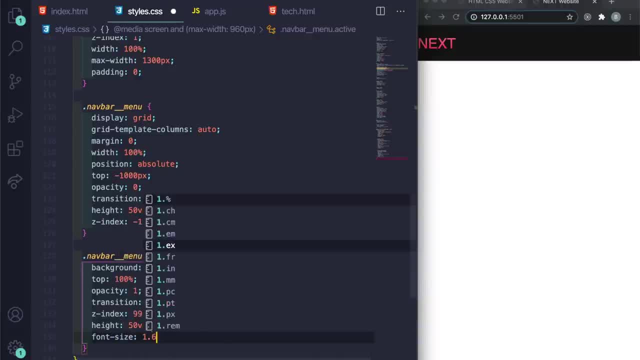 and then set the height again to 50 vh, and then set the height again to 50 vh, and then font size, and then font size, and then font size will be 1.6 ram. so right now you can't see anything yet. so right now you can't see anything yet. 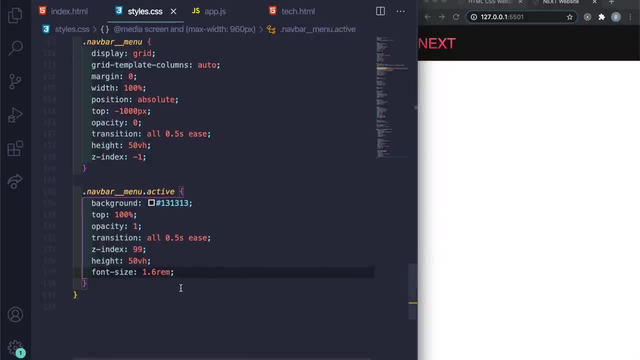 so right now you can't see anything yet because we still have to actually, because we still have to actually, because we still have to actually edit the menu bars now. so let's go edit the menu bars now. so let's go edit the menu bars now. so let's go underneath the navbar menu active. 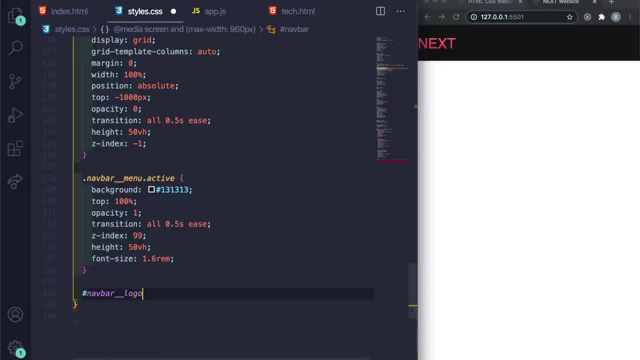 underneath the navbar menu: active. underneath the navbar menu: active. and let's just do hashtag navbar and let's just do hashtag navbar and let's just do hashtag navbar. underscore- underscore logo. underscore- underscore logo. underscore- underscore logo. let's set the padding dash left to be. let's set the padding dash left to be. 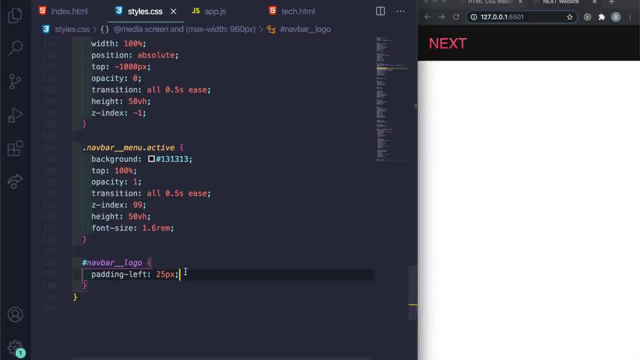 let's set the padding dash left to be 25 pixels. 25 pixels, 25 pixels, and then you can see it's slightly moved, and then you can see it's slightly moved, and then you can see it's slightly moved over, over, over, and then under here let's do dot navbar. 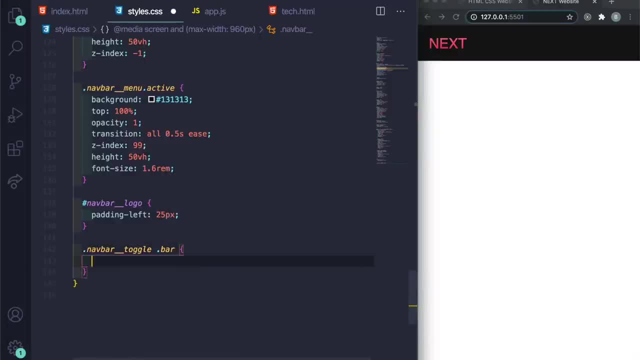 and then under here, let's do dot navbar. and then under here, let's do dot navbar- underscore, underscore, underscore, underscore, underscore, underscore- toggle- dot bar. toggle, dot bar. so now we're targeting the actual bars. so now we're targeting the actual bars. so now we're targeting the actual bars now. so let's say width. 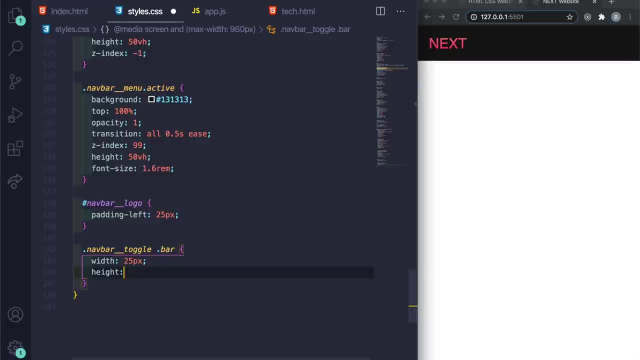 now. so let's say width now. so let's say width, i want it to be 25 pixels. heights, i want it to be 25 pixels. heights, i want it to be 25 pixels. heights to be three pixels, to be three pixels, to be three pixels margin, i want that to be five pixels. 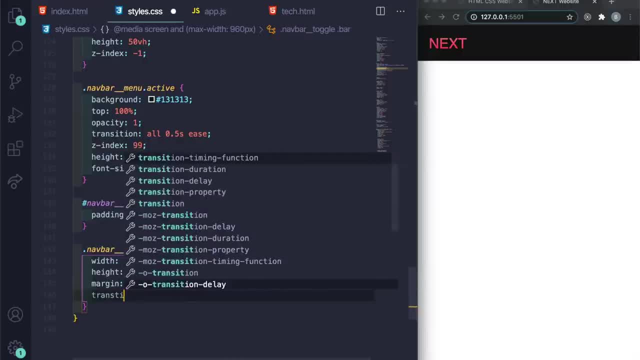 margin: i want that to be five pixels. margin: i want that to be five pixels. auto, auto, auto and let's do transition, let's do and let's do transition, let's do and let's do transition, let's do all 0.3, all 0.3. 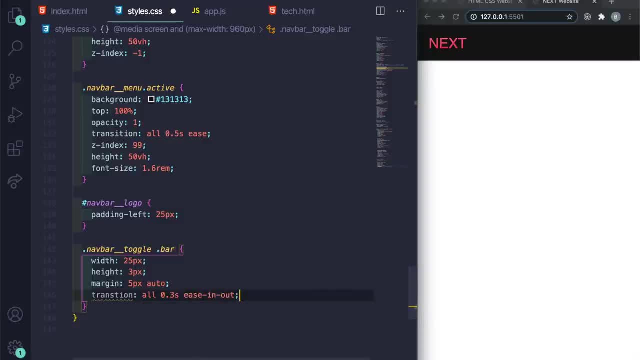 all 0.3 s s s ease dash in, dash out, ease dash in, dash out, ease dash in dash out, and i misspell transition again. so make and i misspell transition again, so make and i misspell transition again. so make sure i fix that. 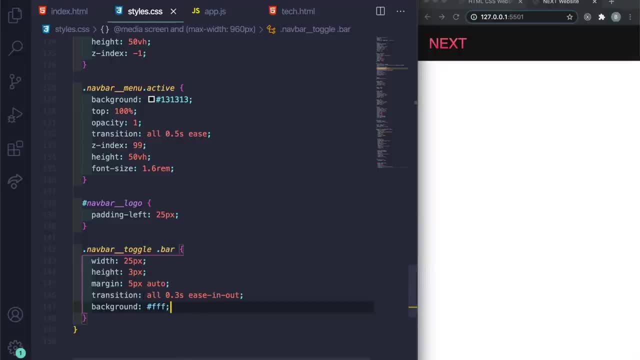 sure i fix that, sure i fix that. and then let's just set the background, and then let's just set the background, and then let's just set the background. equal to hashtag ff, which is white, equal to hashtag ff, which is white, equal to hashtag ff, which is white. and now we should have 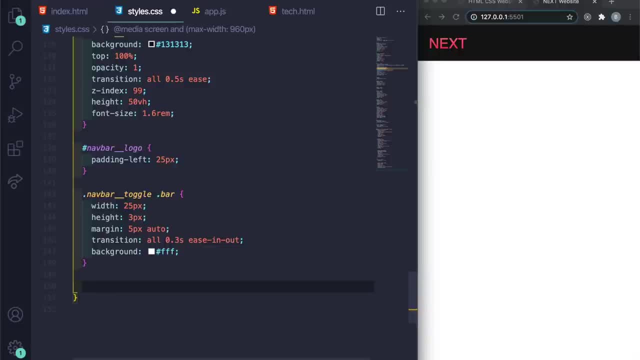 and now we should have, and now we should have this done here, and then let's simply add this done here, and then let's simply add this done here, and then let's simply add the navbar item: so dot. navbar underscore. the navbar item: so dot. navbar underscore. 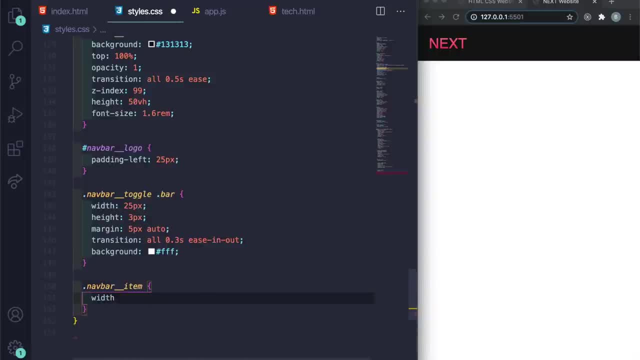 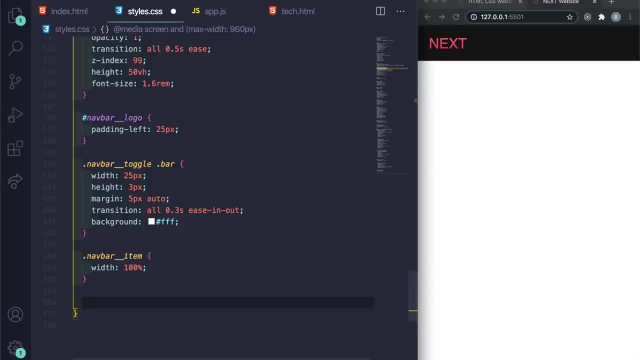 the navbar item. so dot navbar underscore. item: item item. let's set the width to, let's set the width to, let's set the width to 100 percent, 100 percent, 100 percent. and then, underneath this, and then underneath this, and then underneath this, let's do dot nav bar underscore. 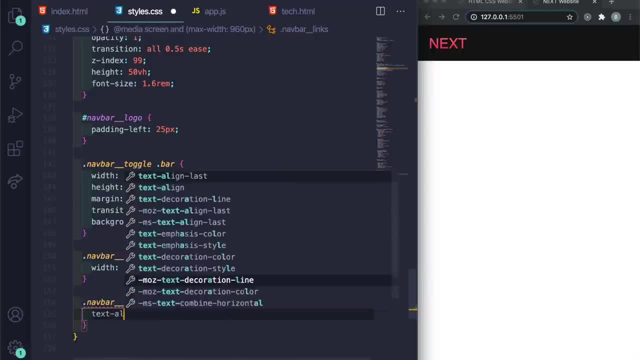 let's do dot nav bar underscore. let's do dot nav bar underscore. underscore links. underscore links. underscore links. i'm going to set the text align to be. i'm going to set the text align to be. i'm going to set the text align to be centered. 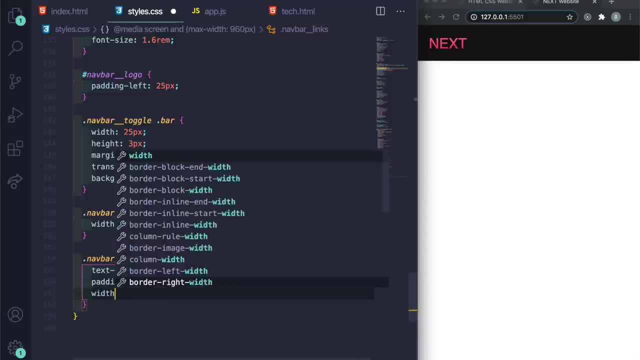 centered, centered. want the padding to be 2rem, want the padding to be 2rem, want the padding to be 2rem, the width to be a hundred percent, the width to be a hundred percent, the width to be a hundred percent and then the display to be. 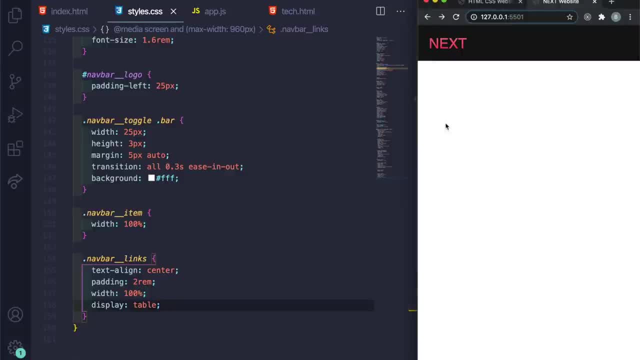 and then the display to be, and then the display to be: table, table, table. so right now looks like, let's see. so right now looks like, let's see. so right now looks like, let's see, yeah, the bars are showing up right now. so, yeah, the bars are showing up right now. so 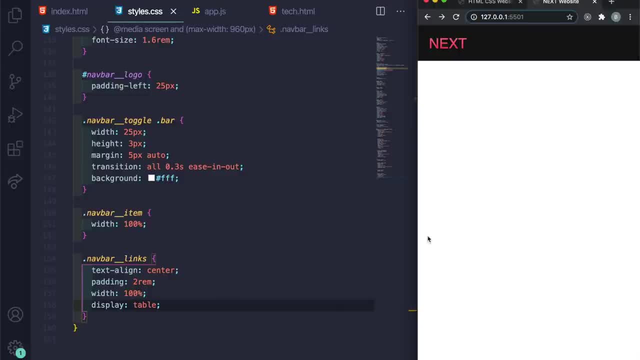 yeah, the bars are showing up right now. so let me see, let me see, let me see, make sure i have everything. oh yeah, so make sure i have everything. oh yeah, so make sure i have everything. oh yeah. so let's add this right here, so we can. 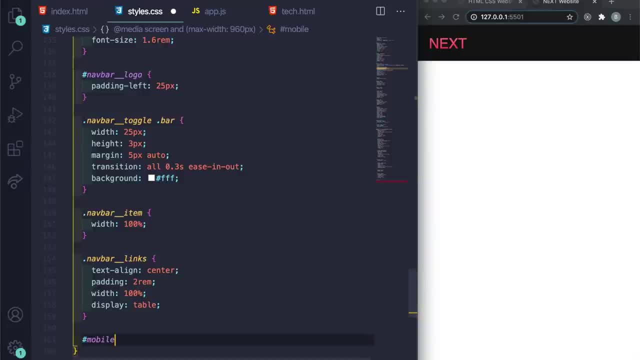 let's add this right here so we can. let's add this right here so we can actually see what's going on. let's do actually see what's going on. let's do actually see what's going on. let's do hashtag so id mobile. hashtag so id mobile. 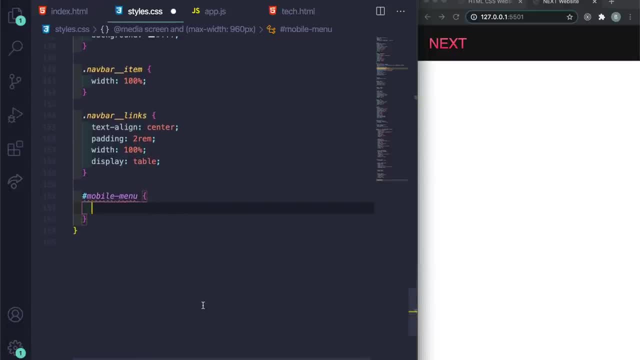 hashtag, so id: mobile dash menu, dash menu, dash menu. and then here i'm going to say position. and then here i'm going to say position. and then here i'm going to say position: absolute, absolute, absolute, top. i want it to be 20 percent, top, i want it to be 20 percent. 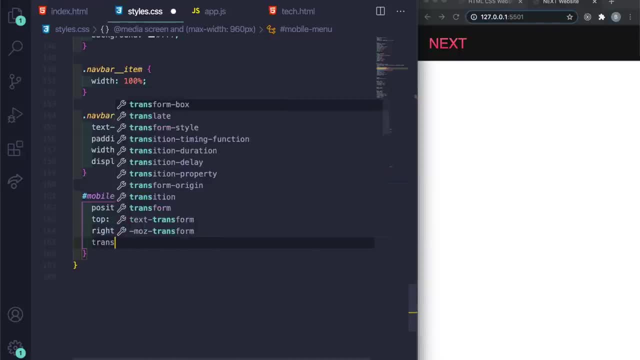 top. i want it to be 20 percent, right? i want it to be five percent, right, i want it to be five percent. and then i want to transform, and then i want to transform, and then i want to transform translates, translates, translates: five percent comma twenty percent. 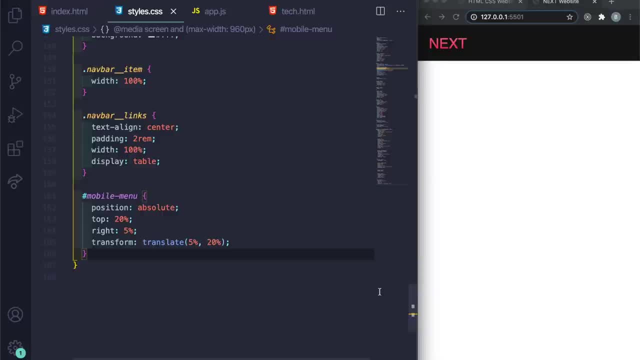 five percent comma twenty percent. five percent comma twenty percent, and save that there, and save that there, and save that there, and then it looks like i need to actually, and then it looks like i need to actually, and then it looks like i need to actually add the um. 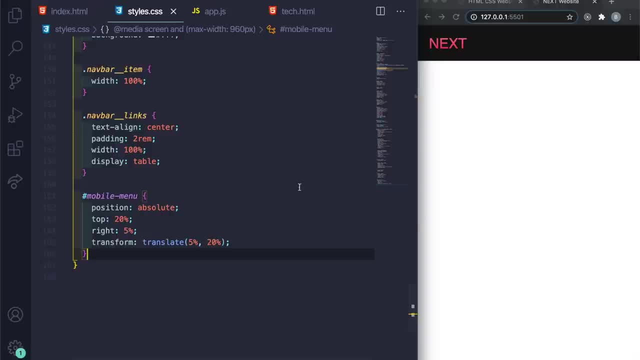 add the um. add the um, let's see what else do we got. so never links. so never links. so never links. let's do navbar btns, let's do dot. let's do navbar btns, let's do dot. let's do navbar btns, let's do dot. navbar underscore, underscore, btn. 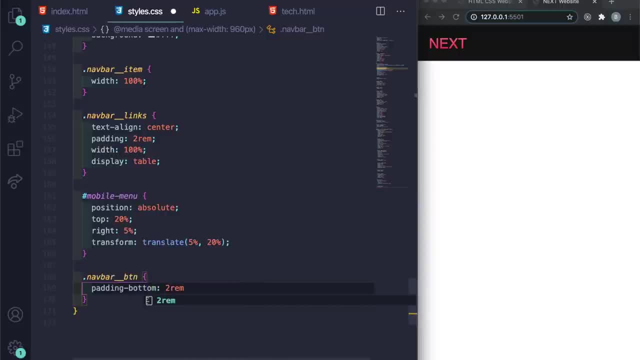 navbar- underscore- underscore btn. navbar- underscore- underscore btn. let's do padding dash bottom to be two. let's do padding dash bottom to be two. let's do padding dash bottom to be two. rem, rem, rem, and then for the button, and then for the button, and then for the button. let's see: 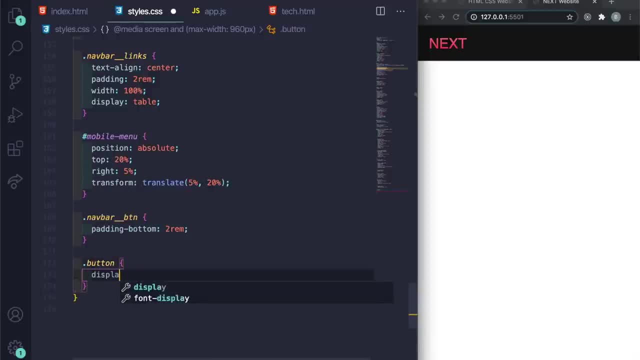 let's see, let's see dot button, dot button, dot button. let's display, let's display, let's display flex, flex, flex, and let's do justify content to be, and let's do justify content to be, and let's do justify content to be centered, centered, centered. and then let's see if i can actually 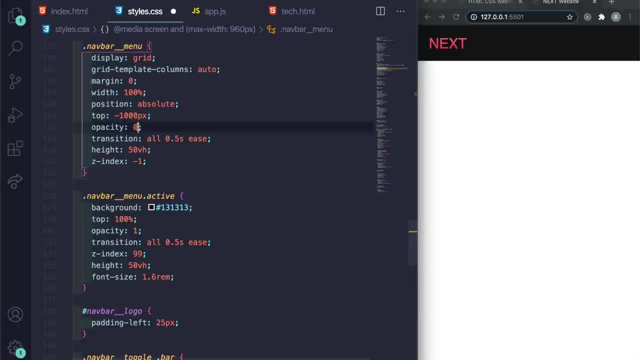 and then let's see if i can actually, and then let's see if i can actually make this uh visible one sec. make this uh visible one sec. make this uh visible one sec. let me just take this out. let me just take this out. let me just take this out, so now you can see what we've been. 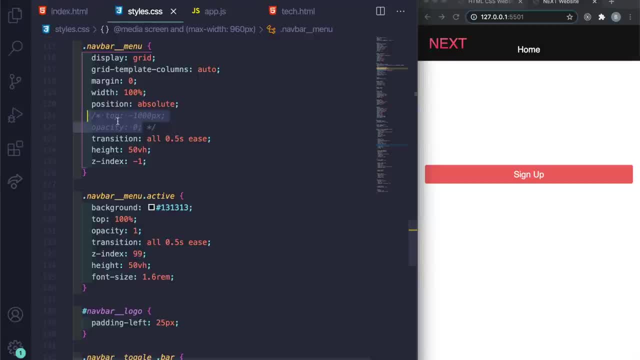 so now you can see what we've been. so now you can see what we've been editing so far, editing so far, editing so far, and it's essentially just the mobile menu and it's essentially just the mobile menu and it's essentially just the mobile menu. so right now i actually put this: 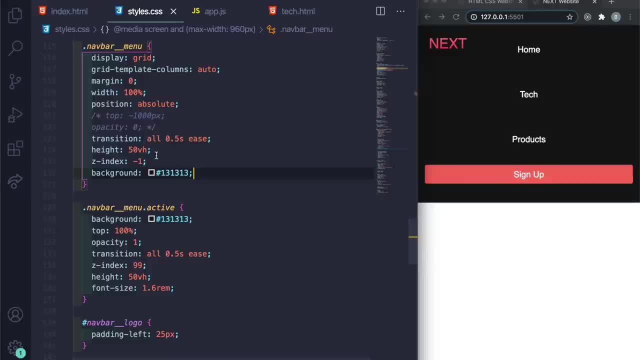 so right now i actually put this. so right now i actually put this background on here. now you can see it much cleaner now. you can see it much cleaner. now you can see it much cleaner and i'll go back and re-comment that out and i'll go back and re-comment that out. and i'll go back and re-comment that out later. but pretty much let's go back to later, but pretty much let's go back to later. but pretty much let's go back to the bottom and let's go back to our the bottom and let's go back to our. 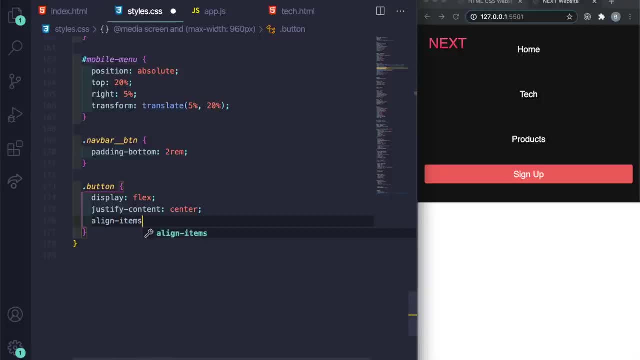 the bottom and let's go back to our button now. button now, button now. and let's do a line items to be center and let's do a line items to be center and let's do a line items to be center. let's set the width to 80. 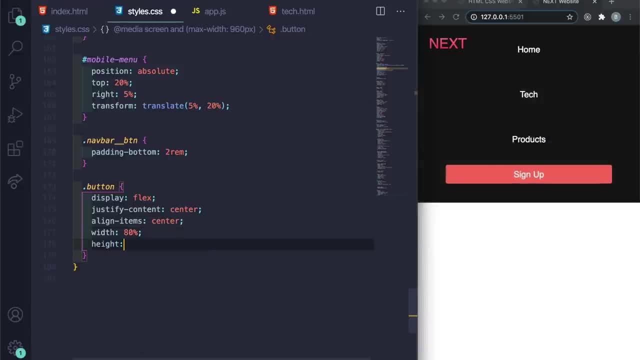 let's set the width to 80. let's set the width to 80. so i shrink the button there. so i shrink the button there, so i shrink the button there. let's do the height to be eight pixels. let's do the height to be eight pixels. 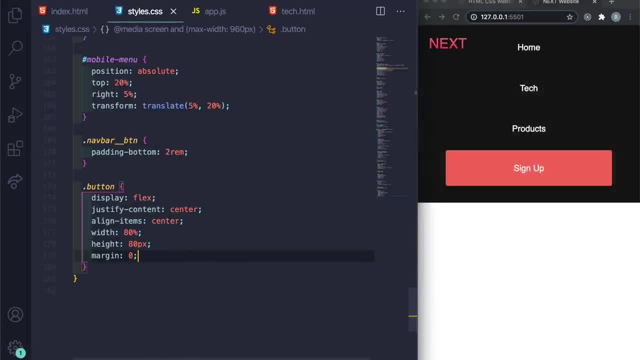 let's do the height to be eight pixels here, and then let's set the margin to be here, and then let's set the margin to be here, and then let's set the margin to be zero, zero, zero. all right, so here's what we got going on. 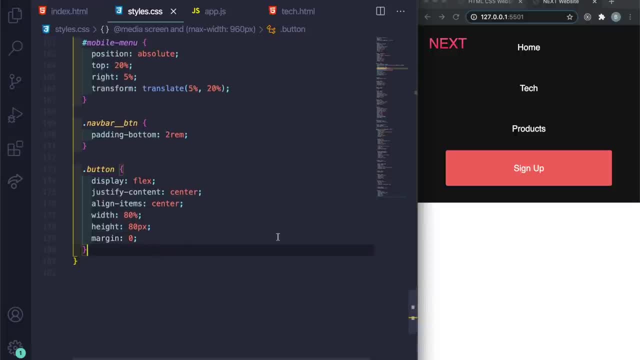 all right. so here's what we got going on, all right, so here's what we got going on right now. and then let's see you got the right now. and then let's see you got the right now. and then let's see you got the mobile menu. 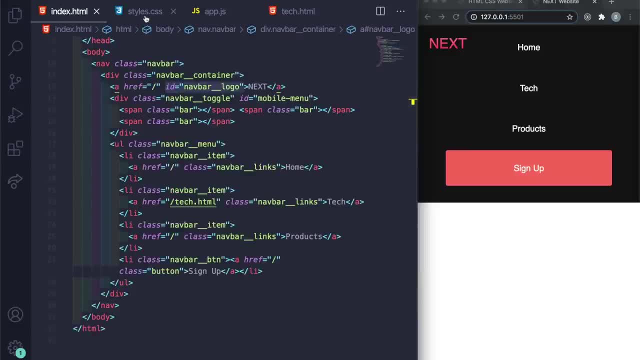 mobile menu. mobile menu, and let me make sure i got all my and let me make sure i got all my and let me make sure i got all my classes. just one second classes, just one second classes, just one second. yeah, i should be fine here. yeah, so now, 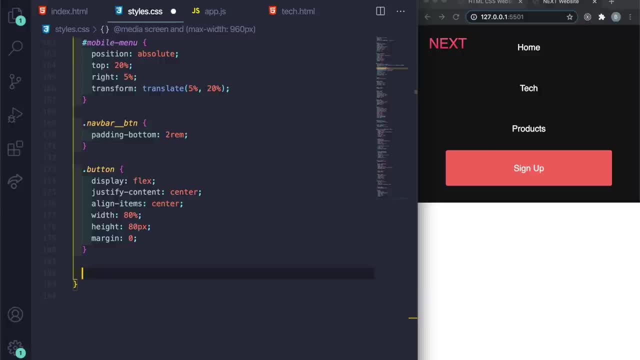 yeah, i should be fine here, yeah, so now. yeah, i should be fine here, yeah. so now let's go underneath this, let's go underneath this, let's go underneath this, and then let's hear the toggle. so now. and then let's hear the toggle. so now. 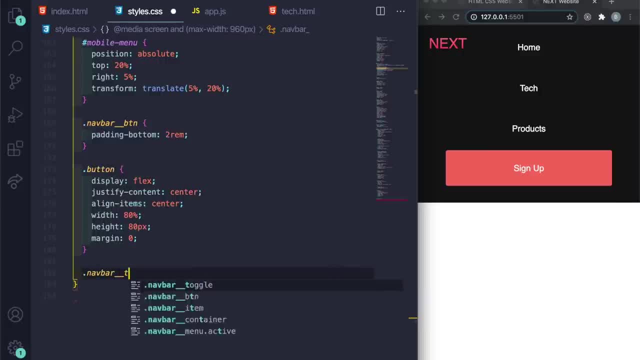 and then let's hear the toggle. so now let's do dot nav, let's do dot nav, let's do dot nav bar- underscore- underscore- toggle bar- underscore- underscore- toggle bar- underscore- underscore- toggle. and then space dot bar, and then space dot bar, and then space dot bar, and then here i'm going to say display to 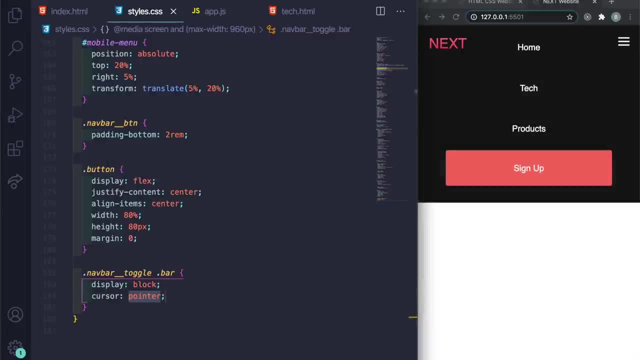 and then here i'm going to say display to, and then here i'm going to say display to be block, and then cursor to be pointer be block, and then cursor to be pointer be block, and then cursor to be pointer. and now we can see we got our little. 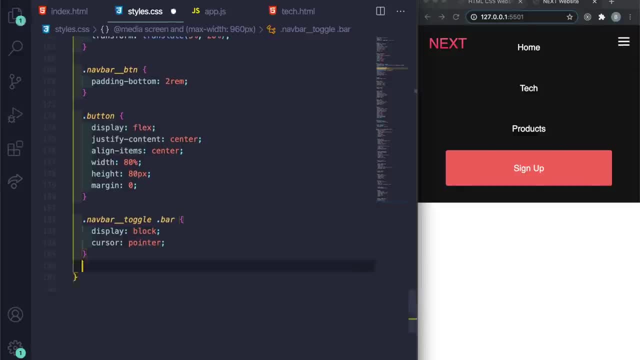 and now we can see we got our little, and now we can see we got our little. more action here, more action here, more action here. so now let's go underneath this, so now let's go underneath this, so now let's go underneath this. and here's the little effect, to where it. 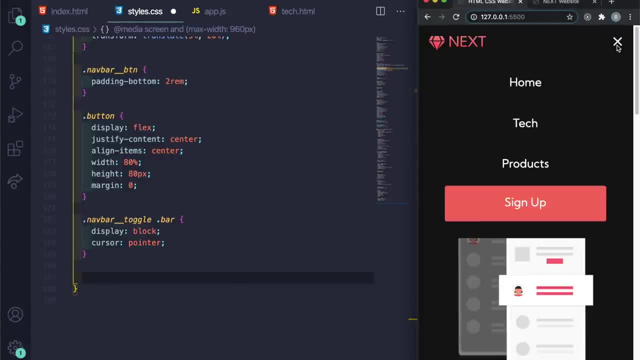 and here's the little effect to where it. and here's the little effect to where it actually actually. actually, we got a little animation effect, so we, we got a little animation effect, so we, we got a little animation effect, so we saw back on the original site. 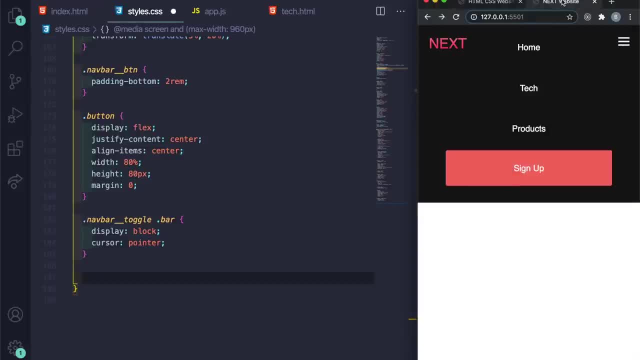 saw back on the original site. saw back on the original site. it like animates it. so this is the way i it like animates it. so this is the way i did this. so pretty much did this. so pretty much did this. so pretty much, what you do is you just do the id. so i 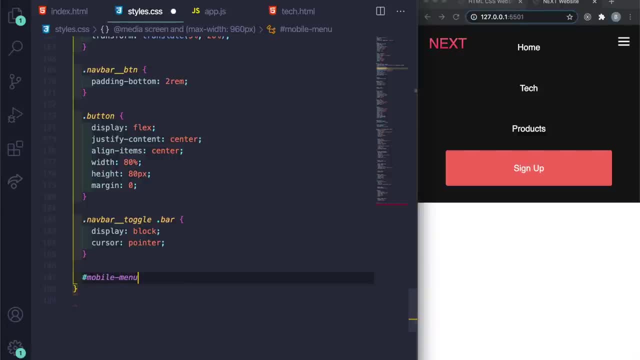 what you do is you just do the id, so i. what you do is you just do the id so i: hashtag mobile dash menu. hashtag mobile dash menu. hashtag mobile dash menu. and then you say dot is dash active and then you say dot is dash active and then you say dot is dash active, which is going to be a javascript. 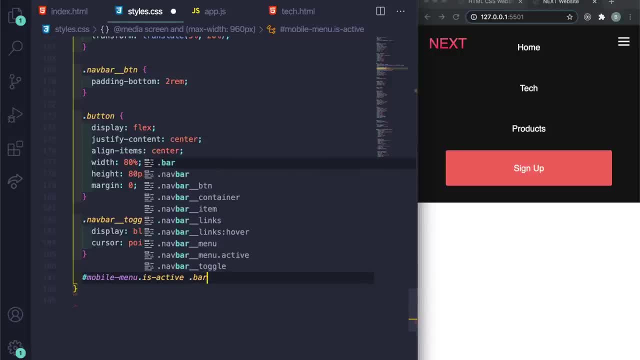 which is going to be a javascript, which is going to be a javascript. we're going to add this in javascript. we're going to add this in javascript. we're going to add this in javascript, and then space dot bar, and then space dot bar, and then space dot bar, and then. 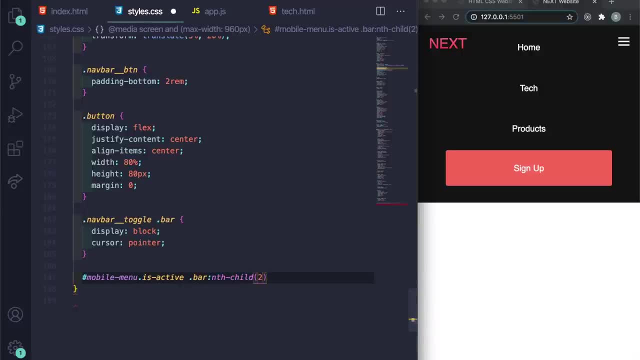 and then, and then colon nth dash child of the second, so, and then colon nth dash child of the second, so, and then colon nth dash child of the second. so this essentially targets the second child, this essentially targets the second child, this essentially targets the second child, and then i just want the opacity to be. and then i just want the opacity to be, and then i just want the opacity to be zero. so i just don't want it to be zero, so i just don't want it to be zero, so i just don't want it to be visible at all. 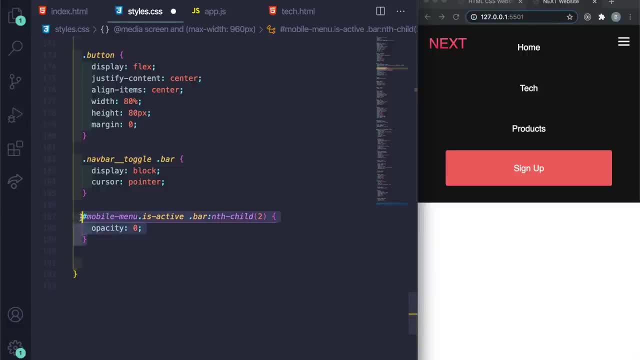 visible at all. visible at all. and then let me just go and copy, and, and then let me just go and copy, and, and then let me just go and copy and paste this again. paste this again, paste this again. so command c, command, victory v. so command c, command, victory v. 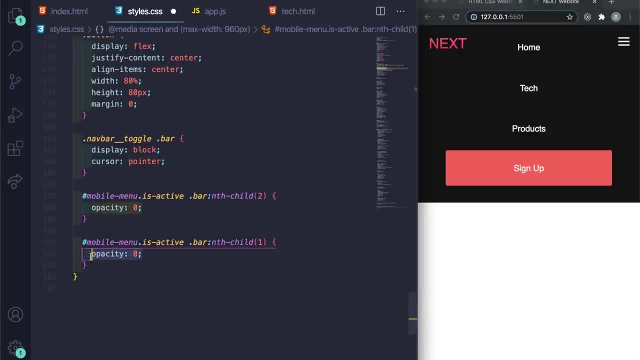 so command c, command victory v, and i want to target now the top bar, so, and i want to target now the top bar, so, and i want to target now the top bar, so i'm going to say one and then i'm inside. i'm going to say one and then i'm inside. 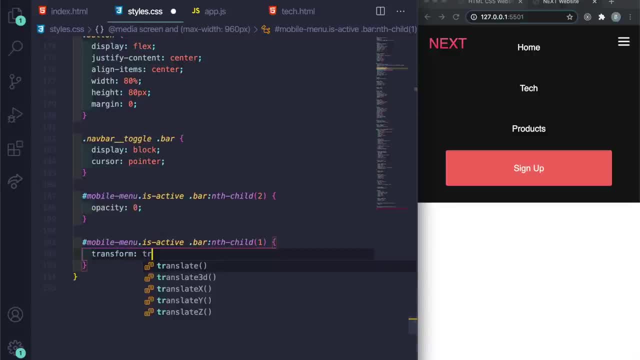 i'm going to say one, and then i'm inside: erase opacity. i'm going to say transform, erase opacity. i'm going to say transform, erase opacity. i'm going to say: transform set equal to translate. set equal to translate. set equal to translate. so translate y. i want that to be eight. 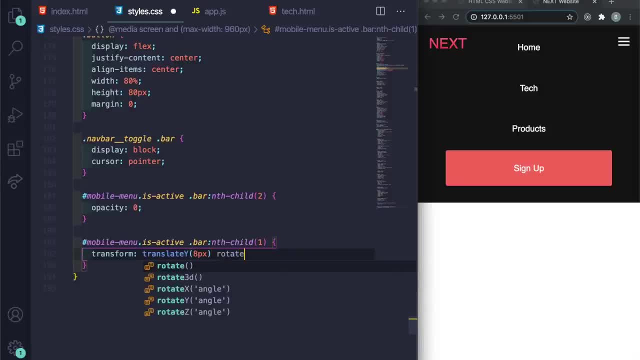 so translate y. i want that to be eight. so translate y. i want that to be eight pixels, pixels, pixels. and then i'm going to set rotate to and then i'm going to set rotate to, and then i'm going to set rotate to become 45 degrees. 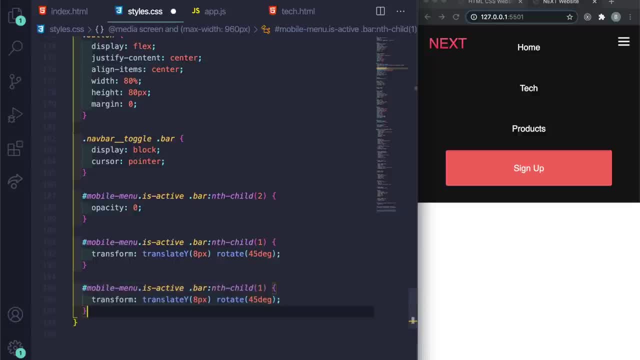 become 45 degrees, become 45 degrees, and then let's copy this again, and then let's copy this again, and then let's copy this again, and then essentially let's change this, and then essentially let's change this, and then essentially let's change this child. so now i'm going to target the um. 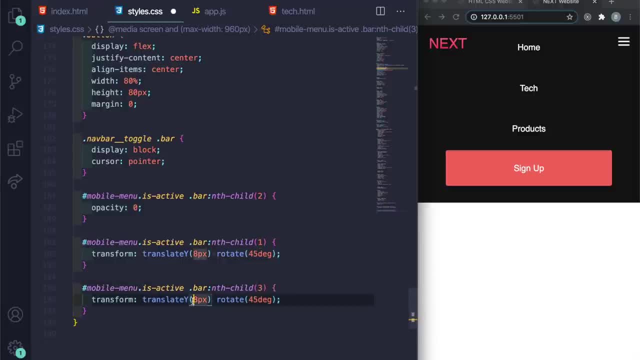 child. so now i'm going to target the um child. so now i'm going to target the um. i'm going to target the third bar now. i'm going to target the third bar now. i'm going to target the third bar now, and then i'm going to change the y to: 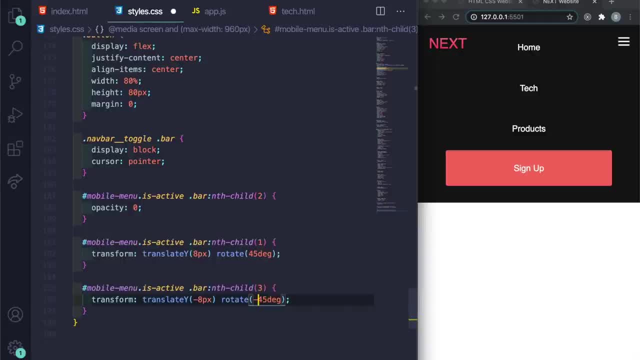 and then i'm going to change the y to: and then i'm going to change the y to: negative 8, negative 8, negative 8, and then negative 45 degrees, and then negative 45 degrees and then negative 45 degrees. so i'll save it now. so right now, when i 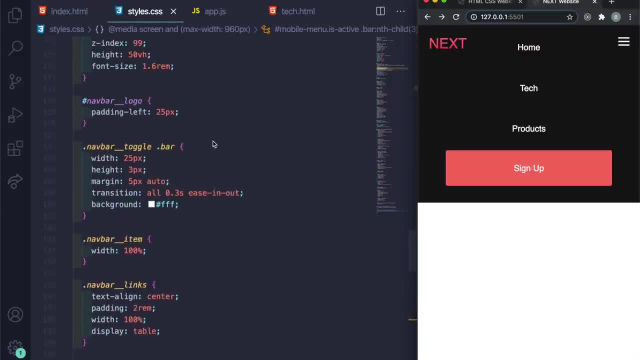 so i'll save it now. so right now, when i so i'll save it now. so right now, when i click it, nothing's happening. click it, nothing's happening. click it, nothing's happening. and also, we have this here, so what i'm. and also we have this here, so what i'm. 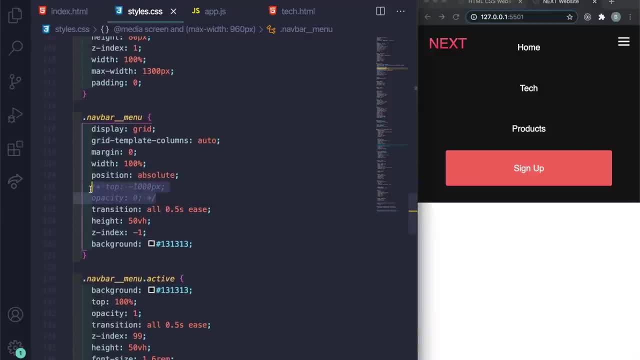 and also we have this here. so what i'm going to do, is actually going to do, is actually going to do, is actually: let me uncomment this out so it. let me uncomment this out, so it. let me uncomment this out: so it disappears, disappears, disappears. and then let's go to our appjs now. so 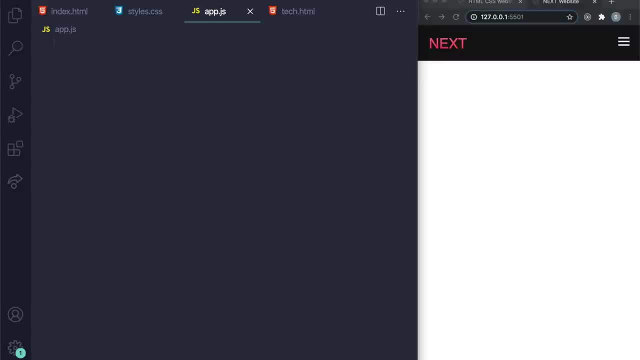 and then let's go to our appjs now. so, and then let's go to our appjs now. so here this is so here this is. so here. this is so simple and super easy, but pretty much simple and super easy, but pretty much simple and super easy, but pretty much what we're going to do is: what we're going to do is what we're going to do is add the effect, the click effect. so it add the effect, the click effect. so it add the effect, the click effect, so it actually animates. so i'm going to say actually animates, so i'm going to say 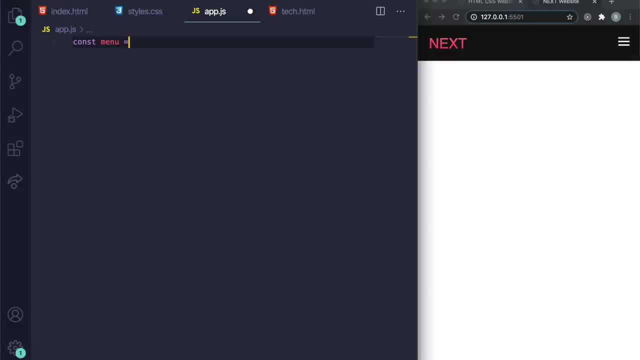 actually animates. so i'm going to say const, and then i'm going to say menu, so const. and then i'm going to say menu, so const, and then i'm going to say menu. so i'm just naming this whatever i want to. i'm just naming this whatever i want to. 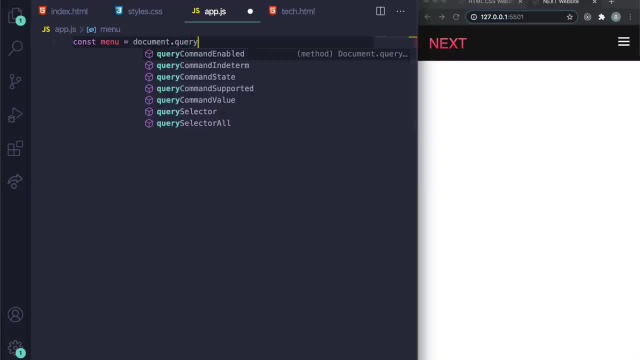 i'm just naming this whatever i want to and i'm going to actually target it. and i'm going to actually target it, and i'm going to actually target it saying document dot query selector. saying document dot query selector. saying document dot query selector, and then the parentheses, and then i have 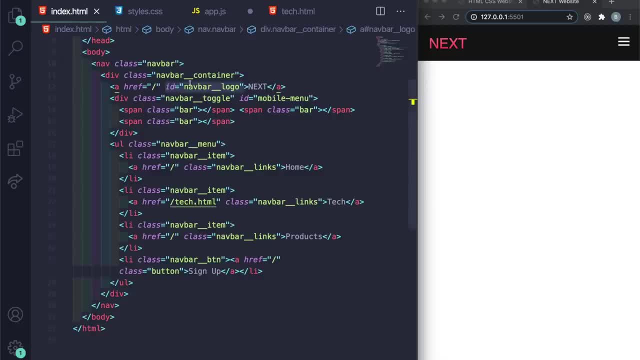 and then the parentheses, and then i have, and then the parentheses, and then i have to do the quotes, to do the quotes, to do the quotes. and what i want to target in the index and what i want to target in the index and what i want to target in the index html is the: 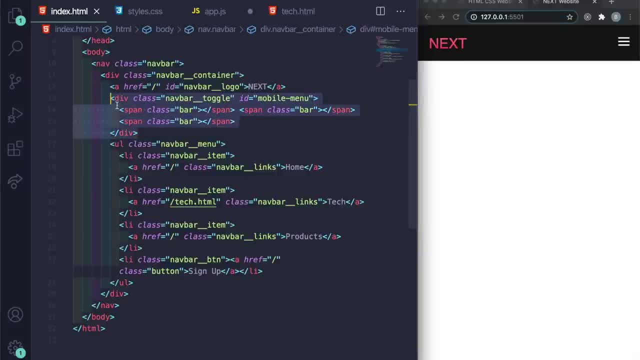 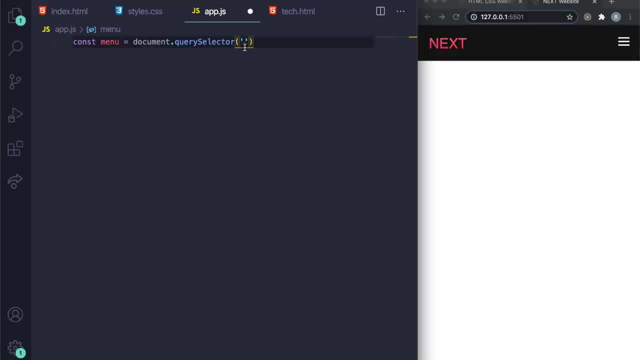 html is the. this is the actual nav, the bars right here, right, and it's wrapped around this div navbar toggle and i put id mobile menu so i can target with javascript. so now i go back here. i'm going to say hashtag for the id mobile dash menu and then underneath 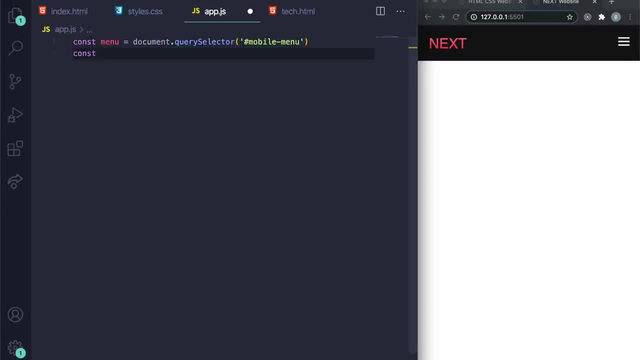 there. i'm going to target another class this time. so i'm going to say cons, menu links with a capital s, i mean a capital l, because they equal to documents. dot- query selector, and then parentheses, quotes, and then say dot- navbar, underscore, underscore- menu, press enter. here you go back. 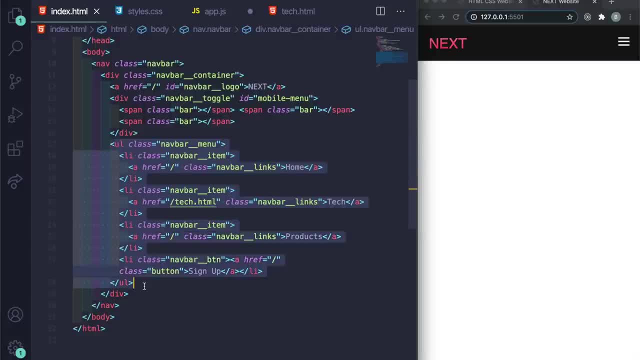 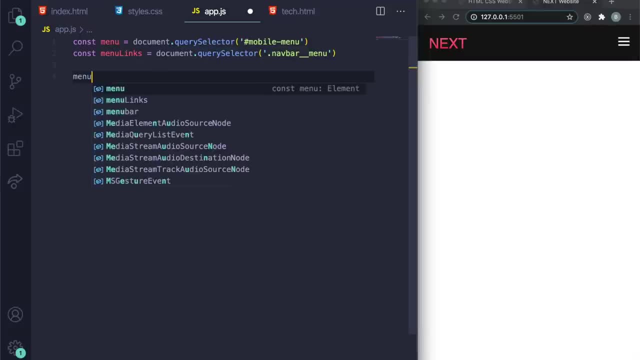 again. now you can see this is the actual ul, this is what we're going to be targeting here, so that we can actually have that trigger too, and to simply target this, we're just going to say menu, which we just created. i'm going to say dot, event, listener, and essentially what we're going to. 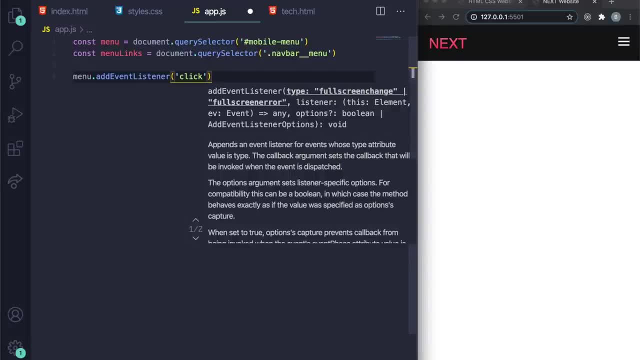 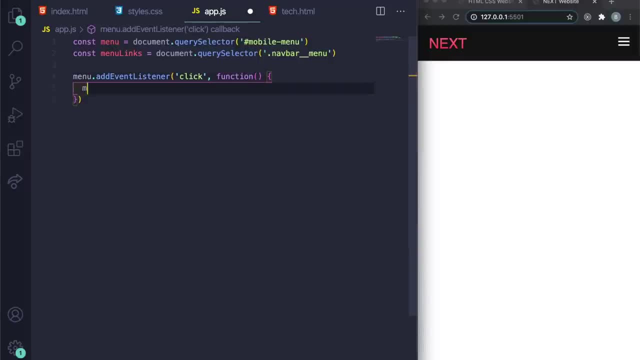 do is we're going to say: dot event listener. and essentially what we're going to do is we're going to do: we have quotes and we're going to listen for a click event. so once we click it, i want a function to run, and what this function is going to do is it's simply going to toggle. so i'm going to say: 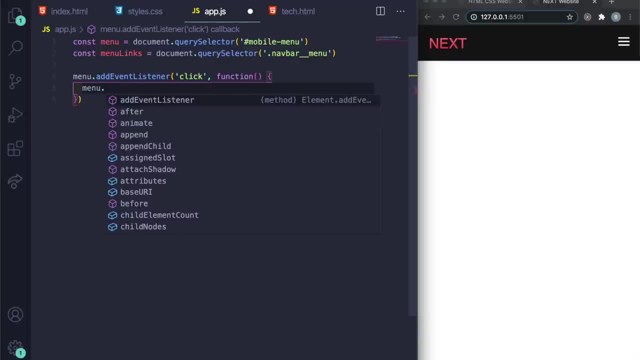 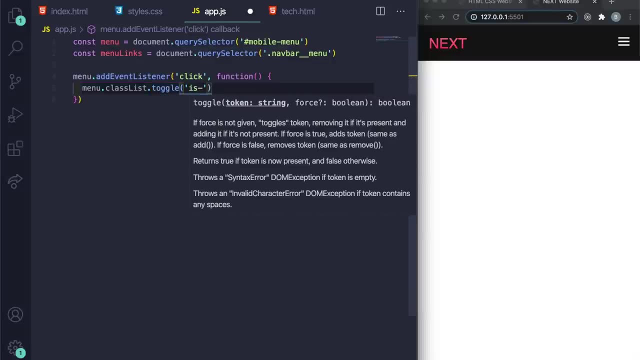 menu dot. it's going to toggle and add a class list. so i want to say menuclasslisttoggle and i want to toggle this one is dash active? and then underneath that i want to do menu links dot, class list. so i want to add this class list dot toggle. 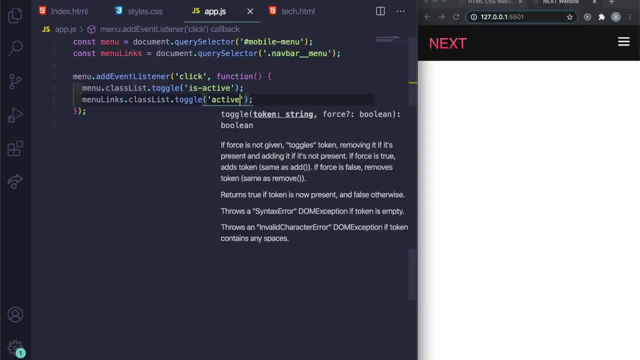 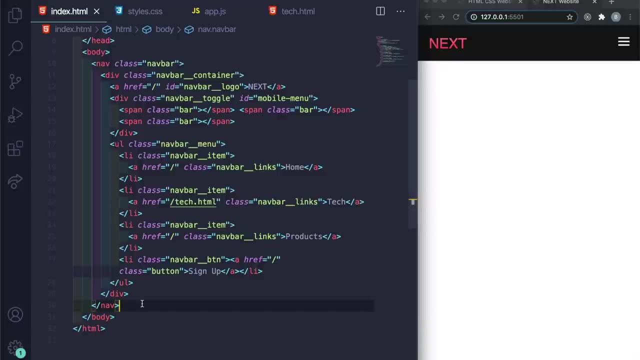 and i'm going to toggle the active class. so we did everything properly, we save, and it looks like something is not working, so let me make sure. oh yeah, the one thing i forgot to do: always make sure you have this: go to the bottom of the nav, right below before the body tag. 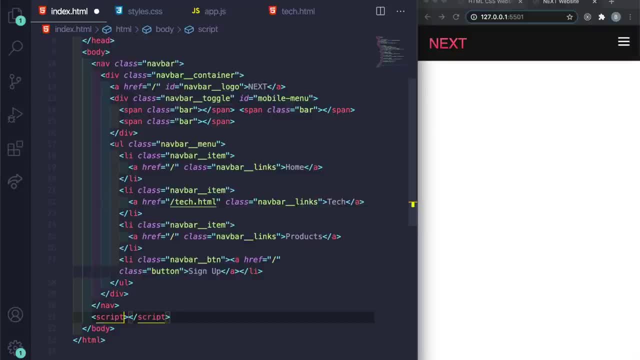 and let's simply do scripts. and i press tab, it automatically has it auto type, and then inside the opening script tag, let's do: src equals to quotes, appjp. yes, save it. so now this should work all right. so perfect. now we have our entire mobile navbar effect. also, when we scroll out here, you can see that everything looks like this. 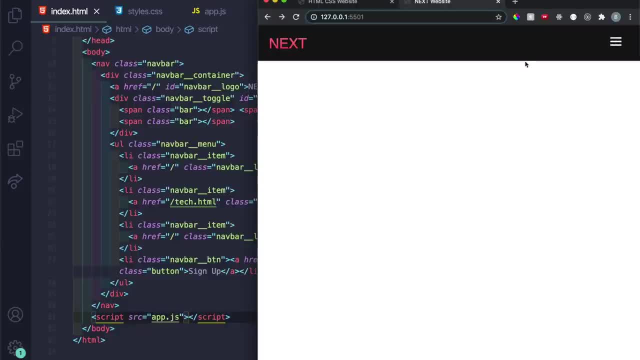 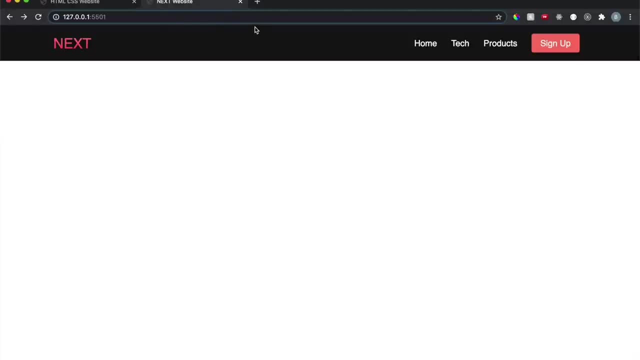 and then again boom, just like that. so there is the navbar. so one last thing i want to do is actually add the font awesome to here, so let me just bring that site up really quick. so here i am on font awesome. so if you've signed up for this site, then you probably already know. but 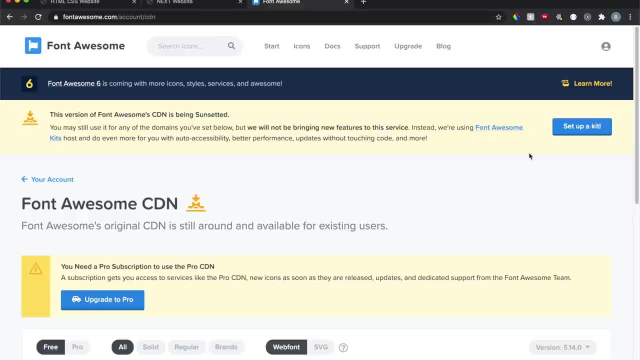 if you don't want to add icons, then don't have to follow this, but this is just in case you wanted to copy it. and also in the footer, this will work out the icons as well, and simply just sign up with an account and then just click on this icon and click on font awesome cdn and it'll lead you right. 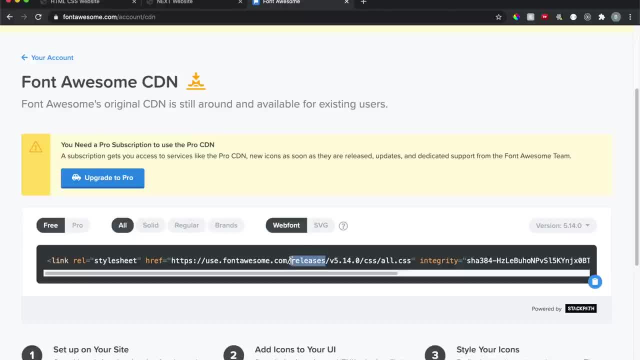 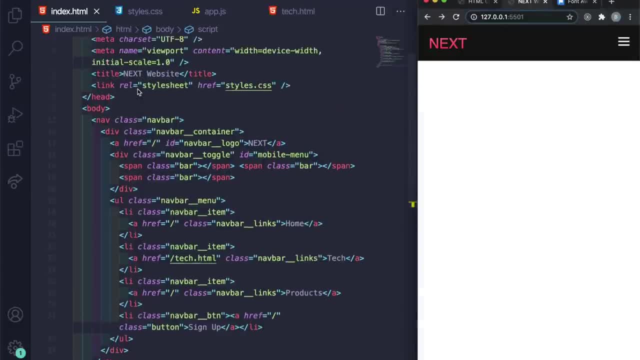 to this page and then, once you have it, you'll have this little cdn here. so i'm just going to copy this, then we just shrink this back over and then i'm going to simply paste this inside the head tag. so let me just do this right under the stylescss. 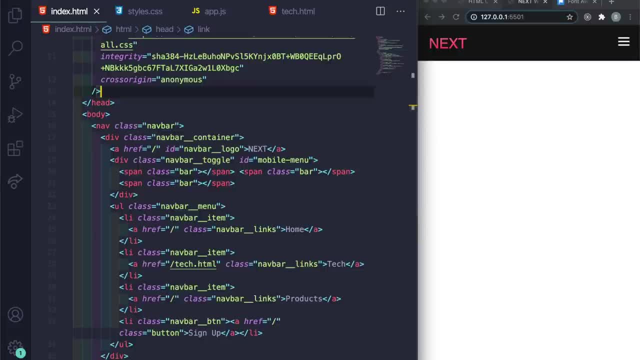 let me save it. and now what we can do is actually add this icon into our logo. so right here, right between the navbar logo and the word next, i'm going to add this icon here. so i'm just going to say opening tag. actually, i'm just going to say: let me space this out so you can see it better. so 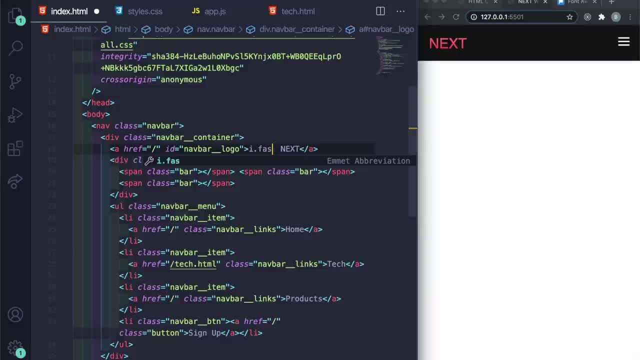 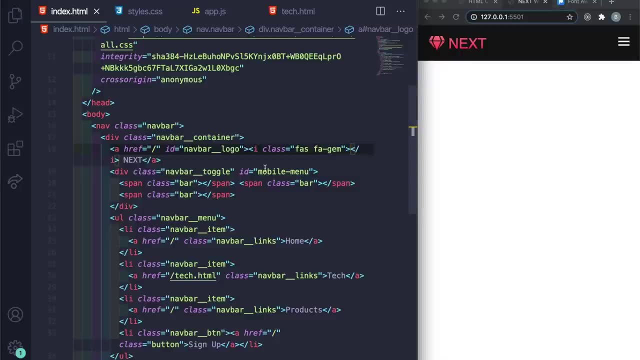 i'm going to say i dot f a s dot f a dot gem press tab, and now you can see that i created this. i tag right here, which essentially is the little diamond icon we got going on and that's right in front of the word next, but it's within the actual a tag. so let me, if i, 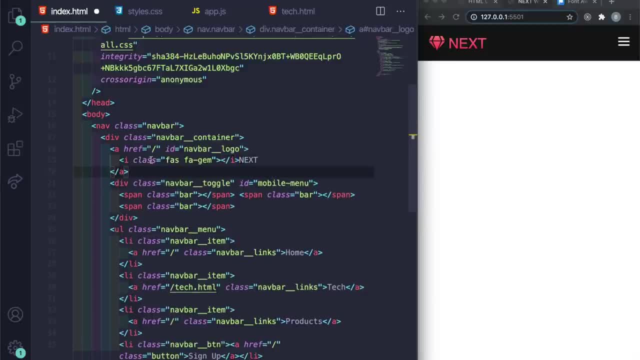 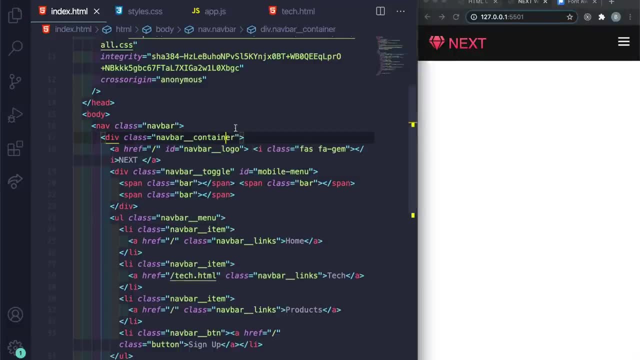 press enter, you can probably see a little better. so you can see like that. so this is essentially how, how it's written like this, and now we have a little icon. so that's good, right there, i'll save it here and now let's go ahead. let me- i'm just going to comment this for you. 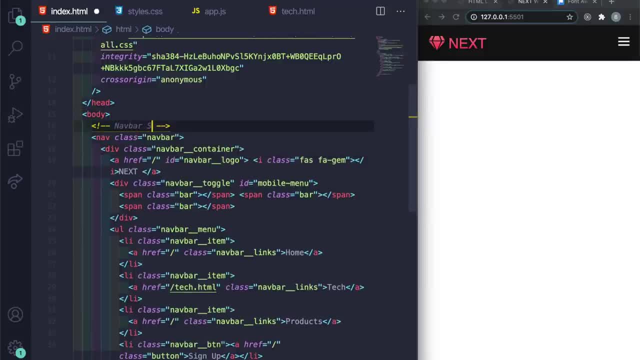 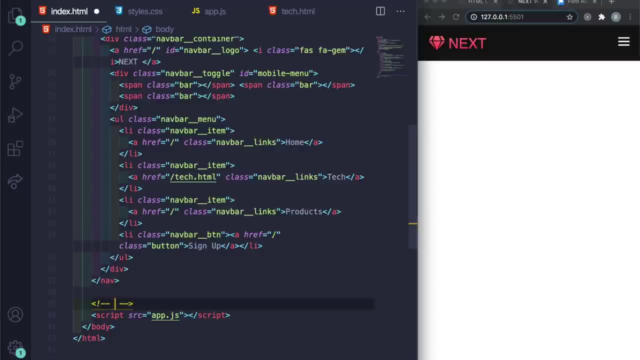 guys to see this. but this isn't. you don't have to copy this. i'm just saying nav bar section here. but this isn't. you don't have to copy this. i'm just saying navbar section here. and now, under underneath this nav, let me press enter and let's create the hero section. so let 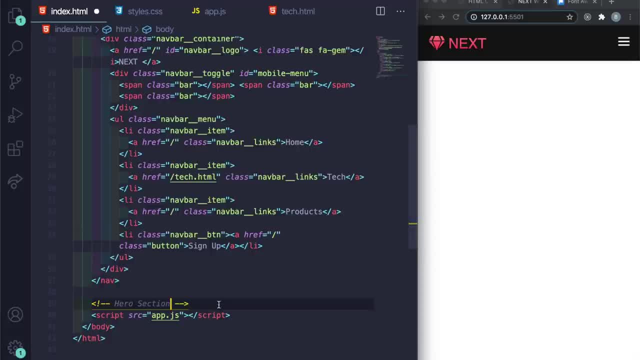 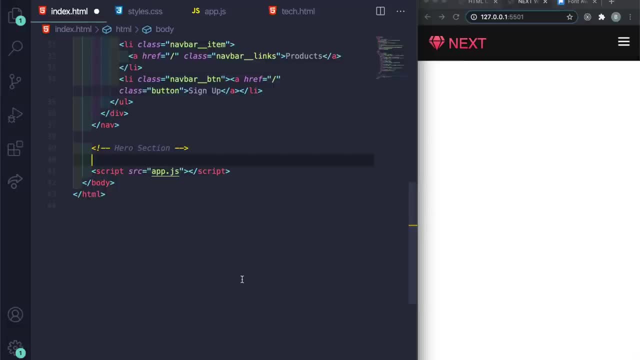 me just say hero section, and let me press, press enter, and now let's go ahead and create the hero section. alright, so now I'm gonna go under here, start adding the HTML here. so first I'm gonna do is dot main. so now we have a div with the 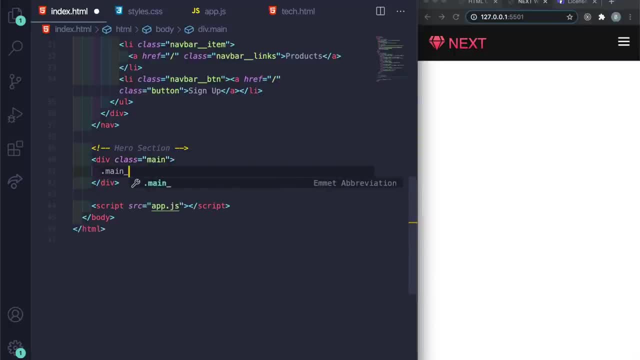 class of main and then say dot main, underscore, underscore container. so now we have a main container and then I'm gonna say dot main, underscore, underscore content and it's going to be essentially our content with our text. so I'm gonna say h1, then press tab, and then I'm just gonna say all caps, next generation. then 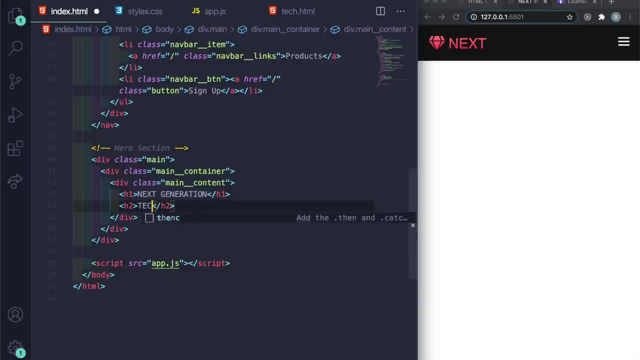 underneath the h1, say h2, and let's just say technology, and underneath this h2 let's just say p-technology tag, and then let's do see what makes us different. and then boom. i think I misspelled. in the original version I think I said: what's that say? I see what. 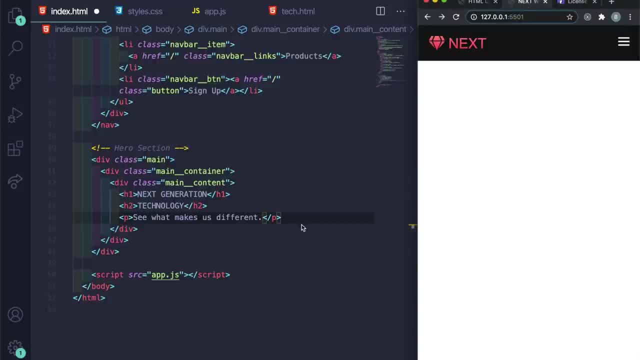 makes up. see what makes up different. eh, it doesn't matter, there's just text here. and then underneath this P tag, let's just say button and then say dot and let's do main underscore, underscore btn. and now we have this main button right here with the class, and then on inside of the button i'm gonna do a and just 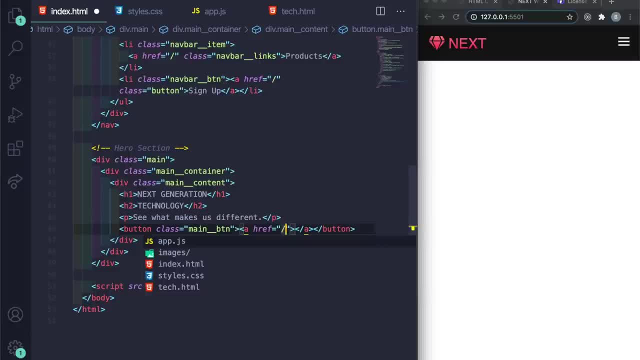 press tab. now we have an a tag and let's put a slash here, and then inside of the a tag i just want to say: get started, save it. and now we have a beautiful looking site, just kidding. so let's go underneath- so here's the button underneath this div- and press enter, and then i'm gonna say: dot. 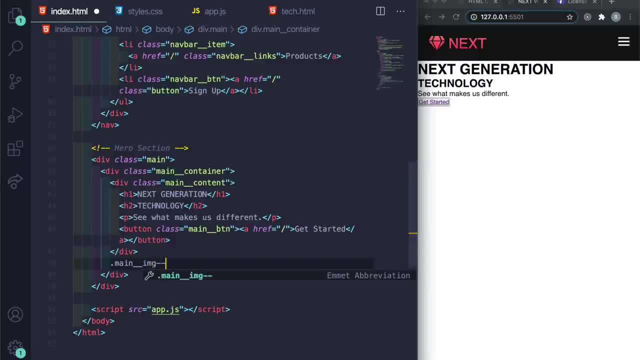 main underscore image img- dash, dash container. and then inside of here i'm just gonna do image, so img, with an id of main underscore, underscore img, press tab and for the src we're gonna do images slash. pick one dot svg and i'll show you where i got these pictures from. 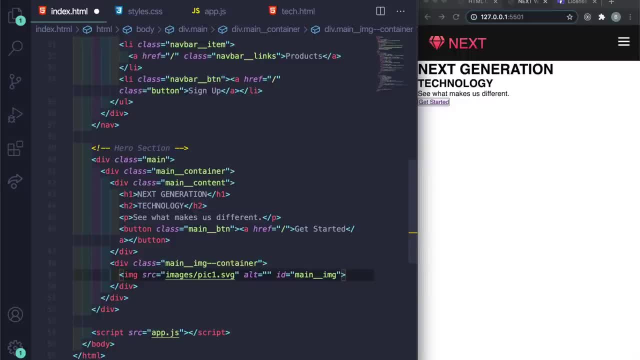 and then for the alt, let's just do: um, what was my picture? i don't even know. let's just do pick, for now it doesn't matter and let's save it. so right now, let me command b. you can see everything. this is pretty much all the html we need to actually add in a picture to the 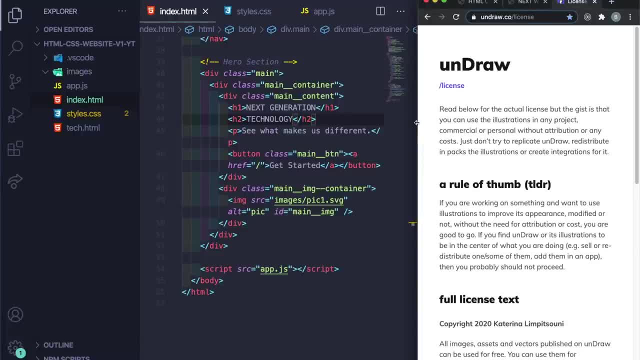 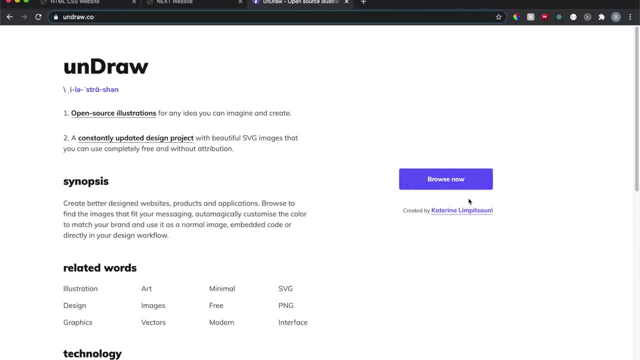 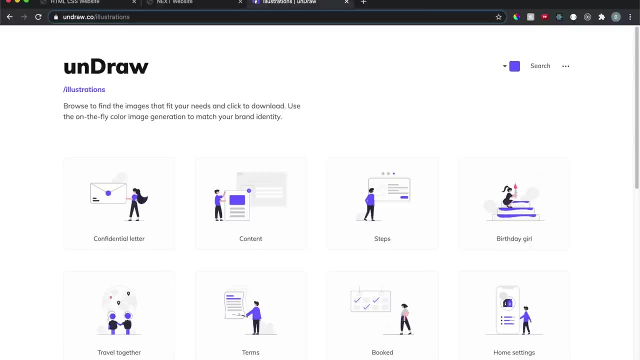 images. so let me show you the site that i got this from. so this site's called androco and essentially these are free illustrations. so when you're on here, you just hit return and then just click on browse now and what you can do is you can actually go ahead and pick a color. so let me see what color. 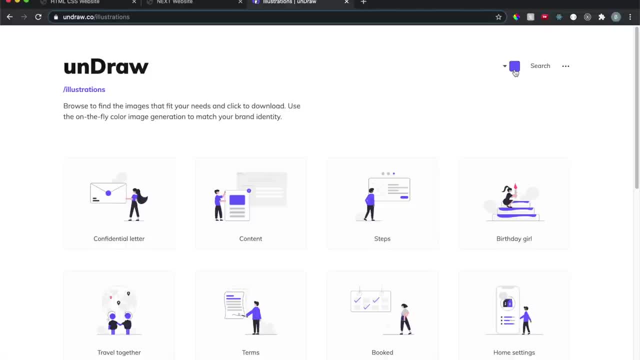 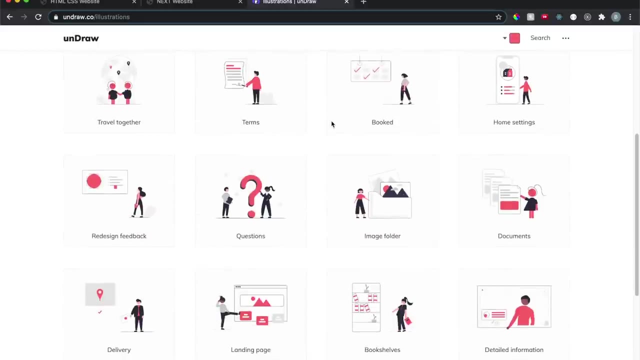 i use for the actual image. so you want to copy my exactly? i just got you. just click on the color and just paste it in. so i got fa6771, just put a hashtag and then you pretty much look like this and then from here you can just scroll in here, click on any of these and then just download svg. 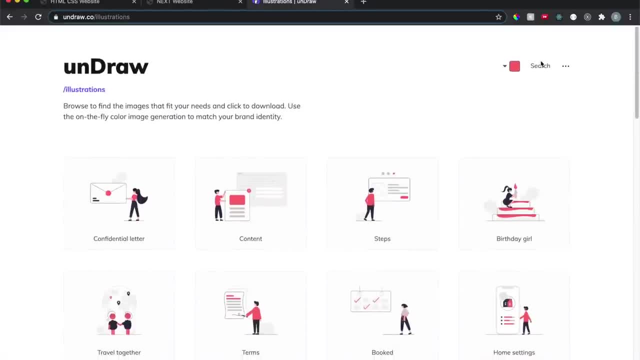 for your project, so go, feel free to pick one. i think i put messages. let me see or just message. you know, just click on it and then you can just copy and paste it in here and you can just copy and paste it in here, and then you can just copy and paste it in here and you can. 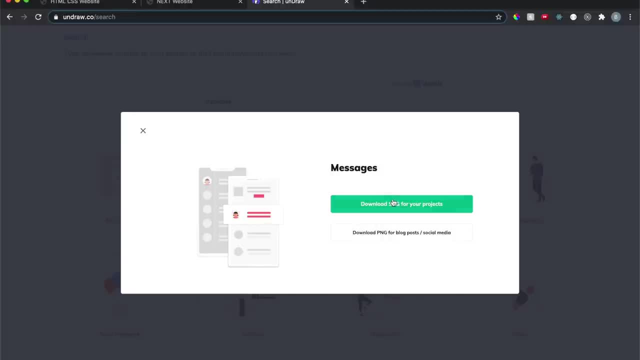 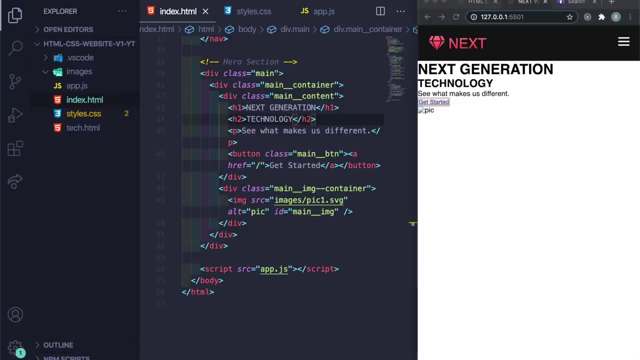 click on here and then i just went ahead and download the svg for my projects and then upload that into my file. so what i'm going to do, i already have it downloaded. so go ahead and download that and let me drag that into my actual project. so give me one second, let me find it, and i'm just 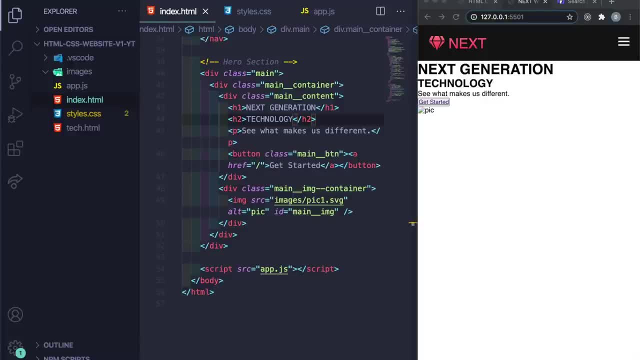 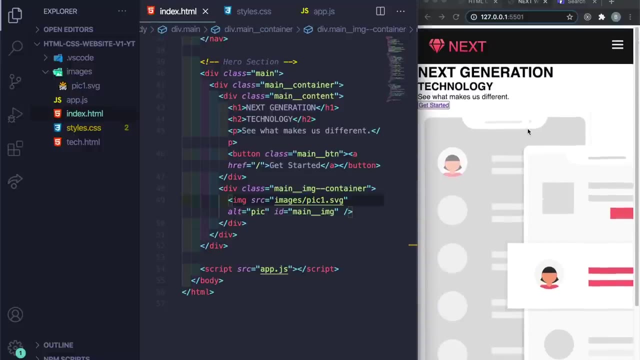 going to drag this over in here into the images folder, and now you can see we have our svg here and i named it: uh, pick dot. i'll just name it, pick one dot- svg. so just make sure you rename it, and then you'll have it here showing up just like this. and now let's go ahead and add. 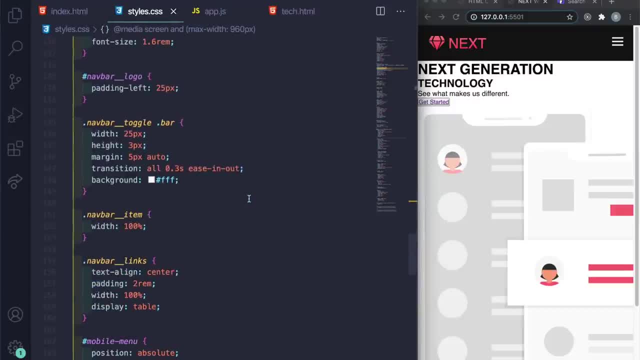 the styles. so go to styles here, and then let me command b so you can see more. and then what i'm going to do is comment. so i'm going to say: let's do hero section, css. and now under here let's just target the main. so let's do main curly brace. let's set the background color equal to hashtag 141414. 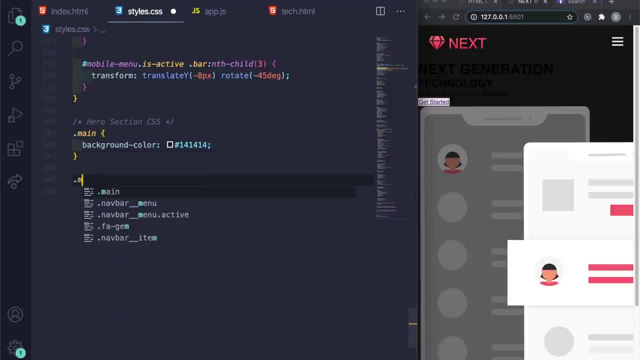 see that there and let's do dot, main, underscore, underscore, container and let's just do display to be grid. let me do grid, template columns and i want it to be 1fr, 1fr, so it's essentially like a 50- 50, even split in terms of the screen space, and let's do align. 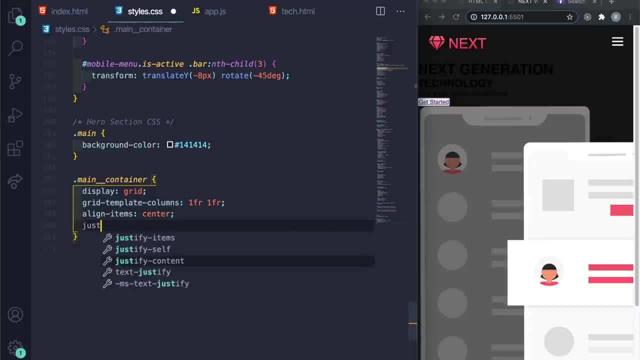 items to be center, let's do justify. let's do self center margin. this is going to essentially center it, so zero auto. and then let's do a height. i want it to be 90 viewport height, so essentially 90 of the screen. and then let's do background color. 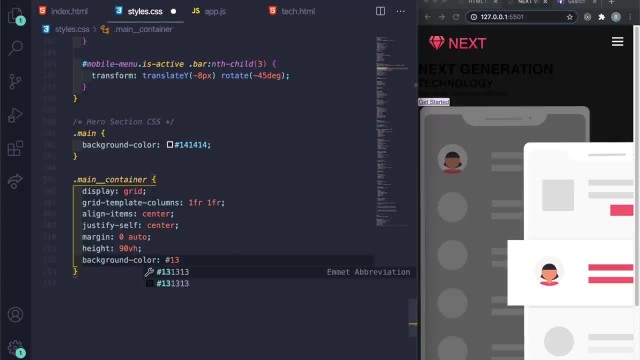 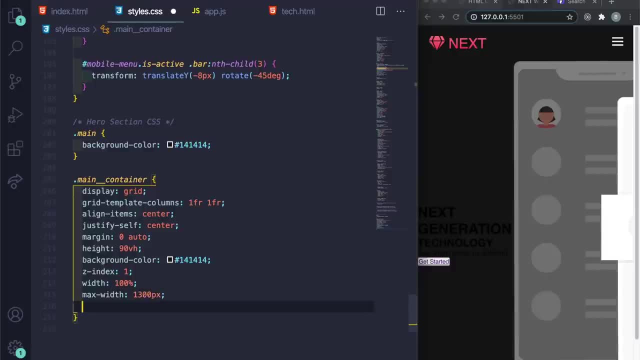 and let's do max width. i want it to be 1300 pixels, and then let's do padding, and i want the top to be zero and bottom to be zero, and then i want the left and right to be 50 pixels each. all right, so now we have the container done, so now let's do the. 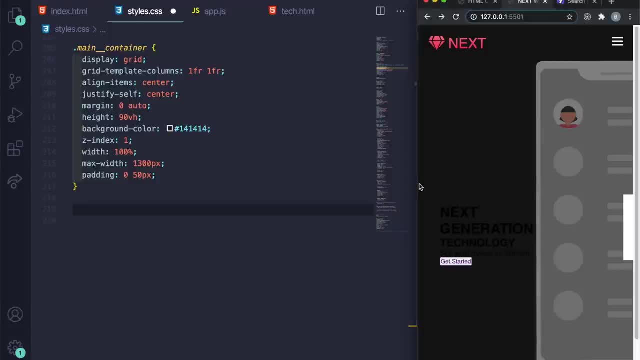 main content. so if i were to actually let me see, i actually brought that out. you can see it's like this. and now let's just do dot main underscore. underscore content h1. and then i'm simply going to say font size is going to be 4rem. background dash color. i want that to be hashtag. 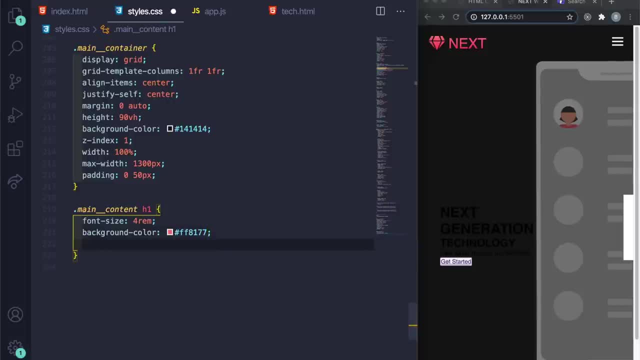 ff8177. and then let's do background dash image to be linear dash gradient to top comma. hashtag f f 0: four, four, zero percent comma. hashtag f f b: one, nine, nine, hundred percent. and then let's do background dash size to become. let's do 100 here and then let's do: 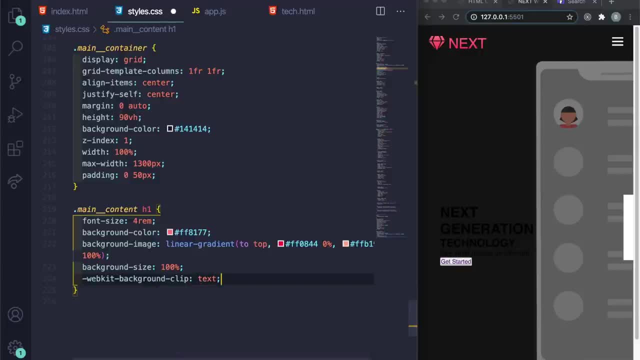 web kit background clip. let's do text. then let's do moz background clip to btex. let's just spell text. and then let's do web kit. uh see, text fill color, and let's just do transparent. and then dash mods, dash text, dash fill, dash color, let's just do transparent as well. 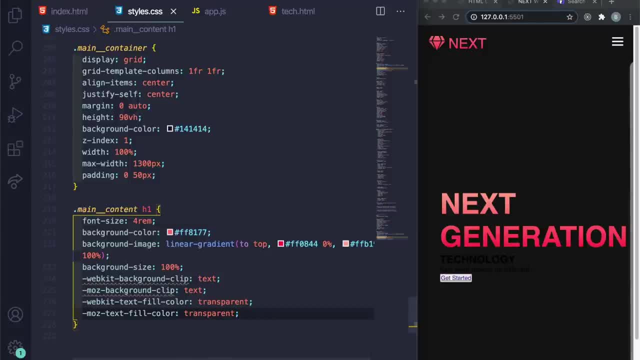 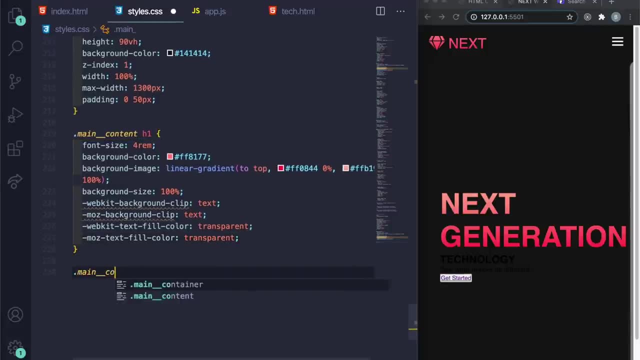 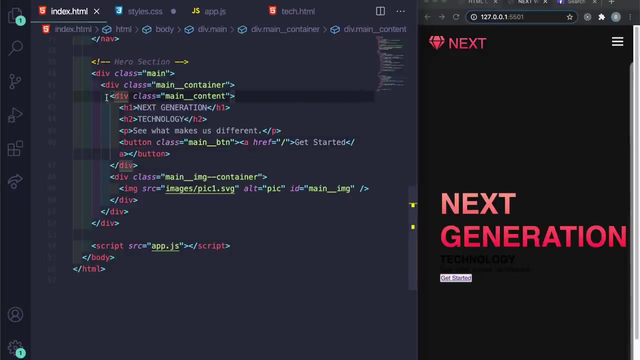 so now we have the text. it's nice and green looking and now let's go ahead and edit the h2. now. so let's just do dot, main underscore, underscore content h2 and notice, in case you're first time confused, like how am i coloring this? essentially, here's the main content. that wraps. 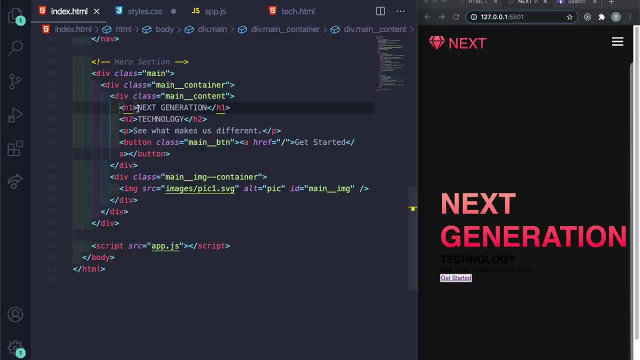 all of this text in here. so i could have just went in here and just like added a class here, custom, like class, you know whatever mean underscore content, you know heading or like yeah, whatever text. but the thing is it's just so much easier and less code, if i just straight up. 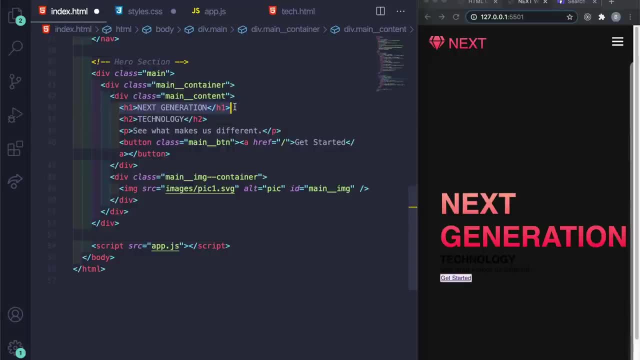 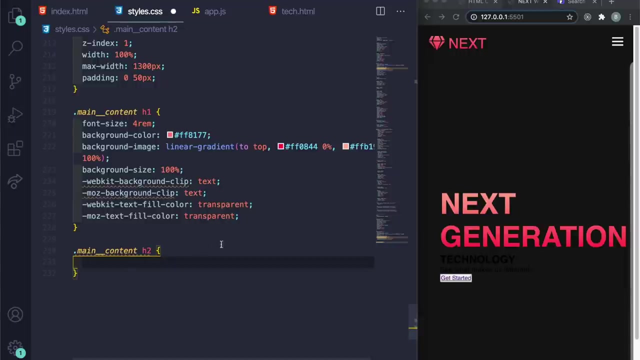 targeted such a the child's in here. so essentially next generation. so it's main content, h1, main content, h2, main content, p button, etc. so essentially, this is what i'm doing here, in case you haven't seen this style, and let's just do pretty much. we're just going to copy and paste this, the only difference. so 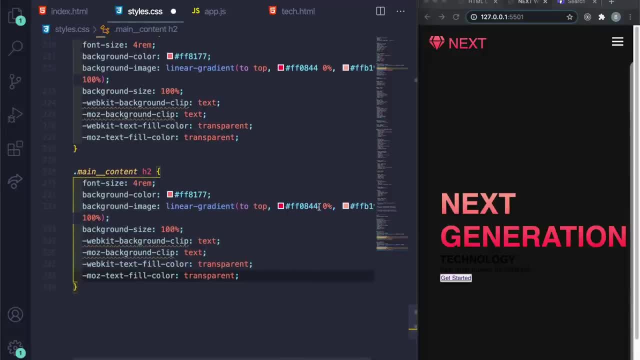 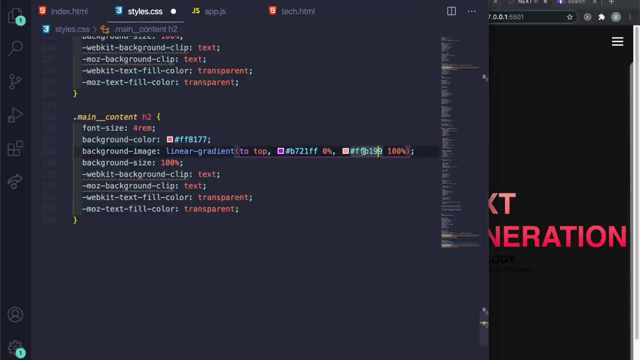 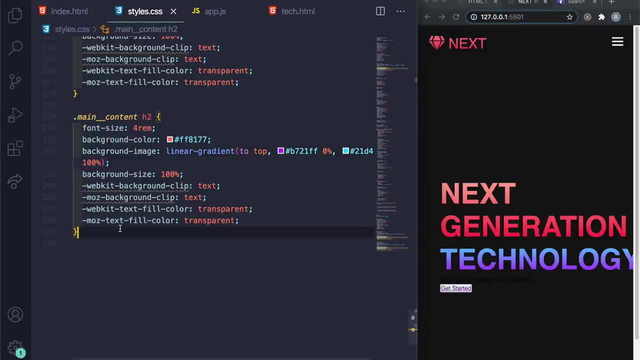 we're going to change the um, the colors. so here let's do, uh, erase this. let's say b721ff, and then for this one looks like i can't even. yeah, i can't see it, but this one let's just do, uh, 21 d4, fd, save it. so now you can see we got some color action going on there. let's press enter. 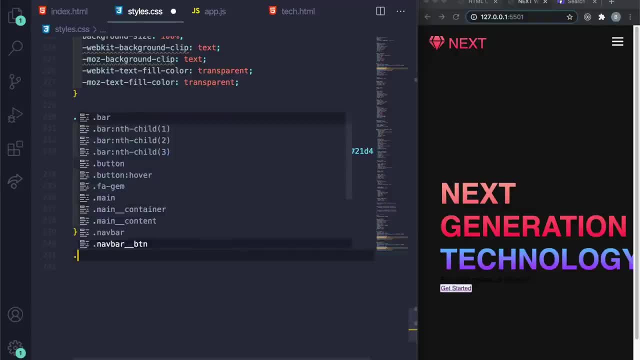 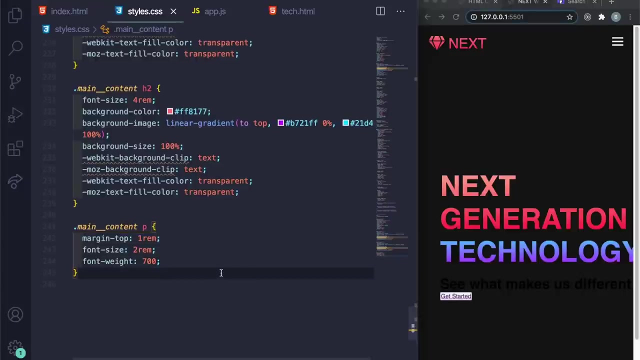 and now let's target the p tag or the paragraph. so let's just do main underscore, underscore content p and let's just do margin, dash top to be one rem, font size to be two rem and font weight to be 700. now we're going to add in um the different font sizes soon, so actually 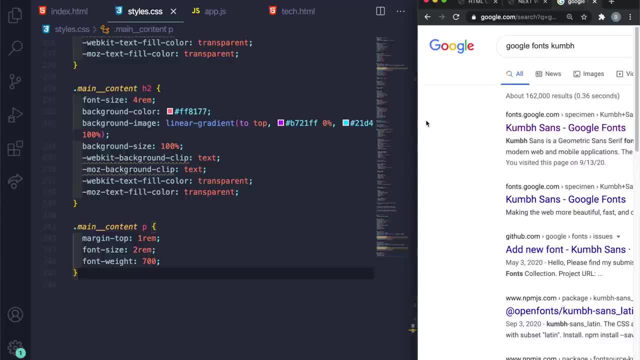 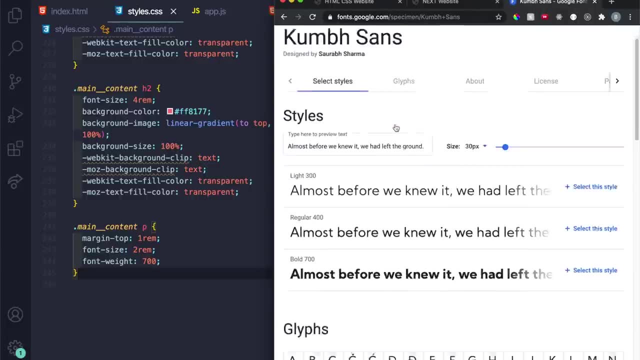 let's just go do that right now. so i went ahead and googled google fonts- k-u-m-b-h, so let me just bring this over. so simply just google this, click on google fonts and now all you need to do is get the regular, so select this style and then also want the bold, and then what you do is you go to 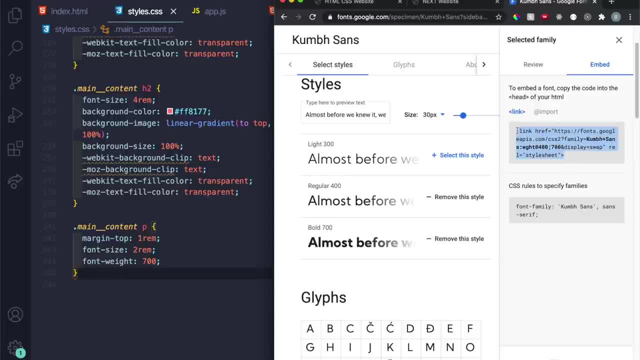 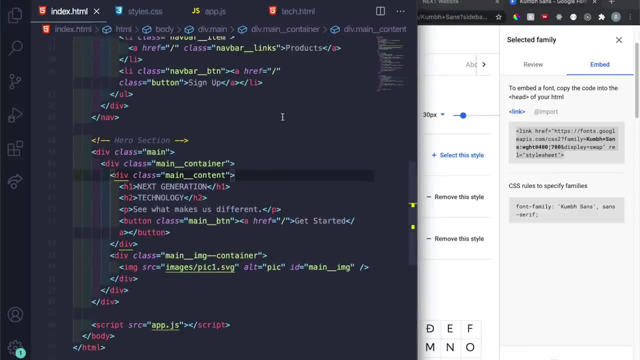 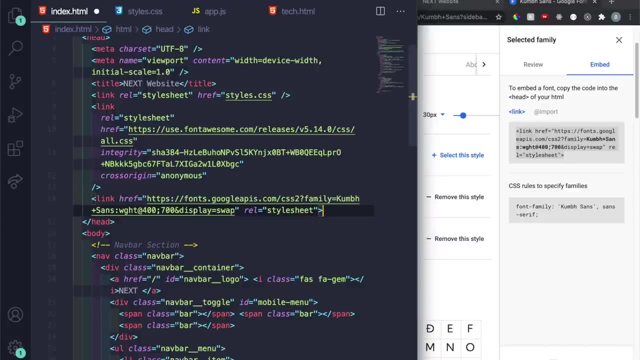 embed and then what you want to do is copy this link tag right here. so i'm going to copy this. go back to our indexhtml file. so now i'm indexed, i'm going to go to the top in the head tag. i'm going to go right underneath the font awesome and just paste this in and just save it there. 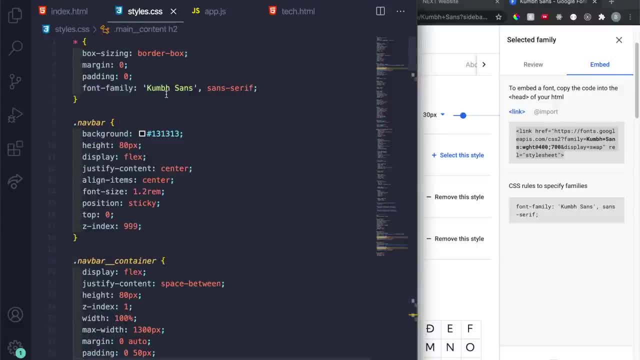 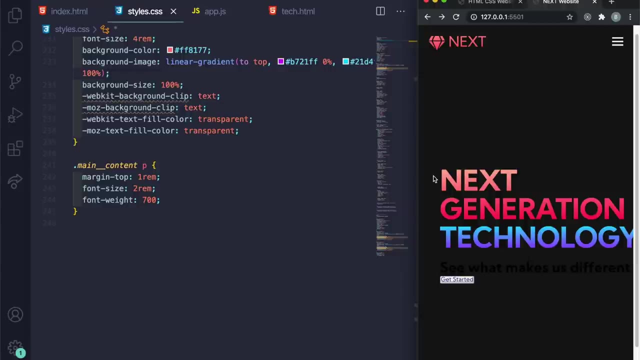 and since we already added that to the top of our, our um css earlier, it should automatically fill out for us. so now, if i simply just go, let me go back to our bottom, go back to our site. you can see it: updates here, and that's essentially how you can add any font. 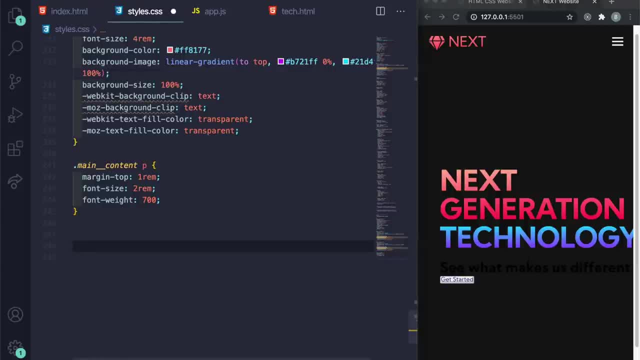 feel free to add whatever you want to. and then let's do the dot main underscore, underscore btn, and then curly brace. here i'm going to say font size to be one rem, background, dash image to be linear gradients to top comma. hashtag f: seven, seven, zero, six, two, zero percent. and then hashtag f e: five, one, nine, six, a hundred percent. 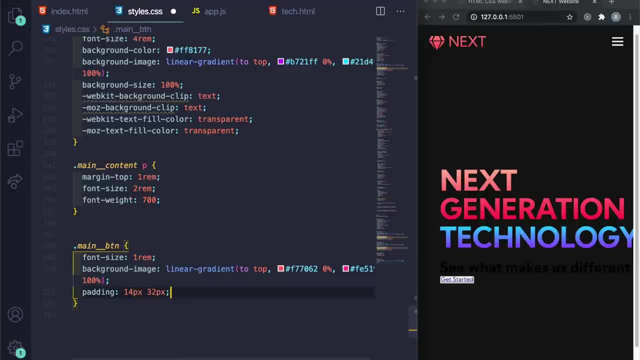 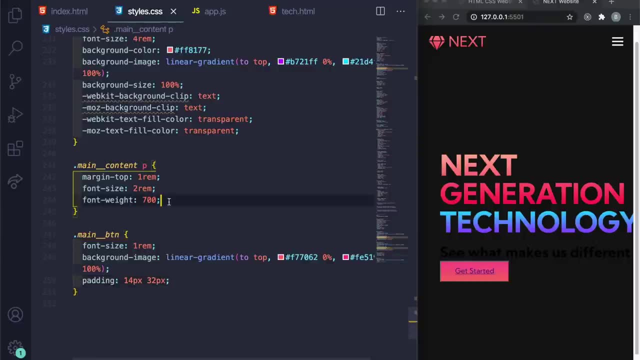 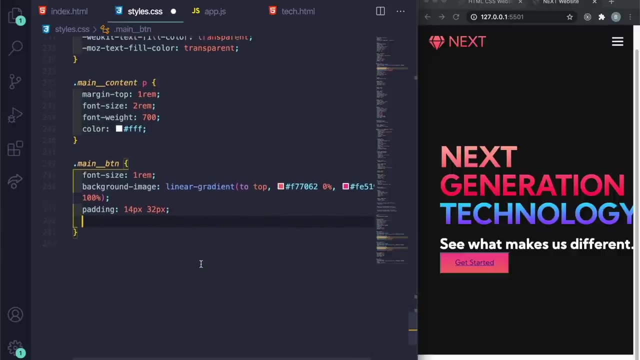 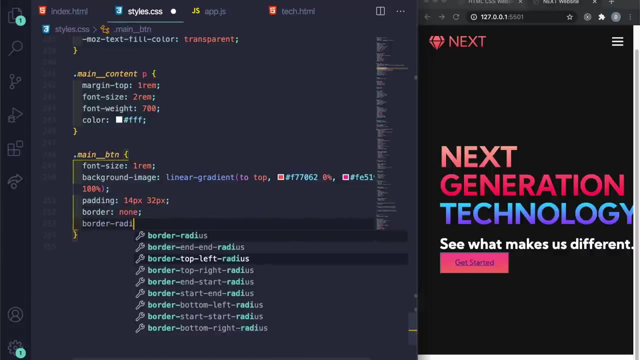 and then let's do padding to be 14 pixels by 32 pixels, so you can see it's starting to go up. and i think i should add actually colored on the p tag to be white, so you can see it all. right, yeah, perfect there. and now for the under padding. let's do border to be none. let's do border dash radius to become. 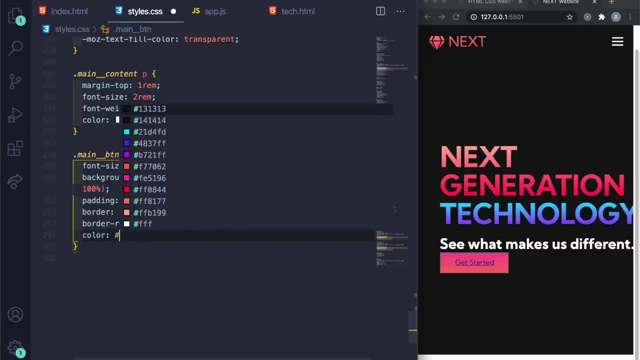 four pixels. let's do color hashtag: fff. let's do margin dash top to become two, rem cursor to be pointer, and then let's do position relative and let's do transition. make sure i spell the transition. let's do just all 0.35 s and let's do outline to be 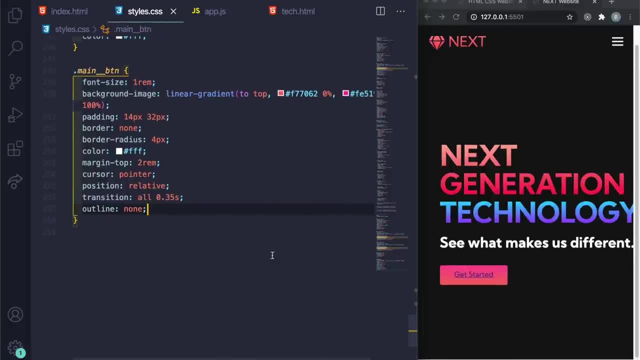 none. so there's our button right there. so now what you do is actually target the a tag inside of the button to get rid of that little underline in the purple text. so i'm going to do a dot. let's do main underscore, underscore btn and then a tag. 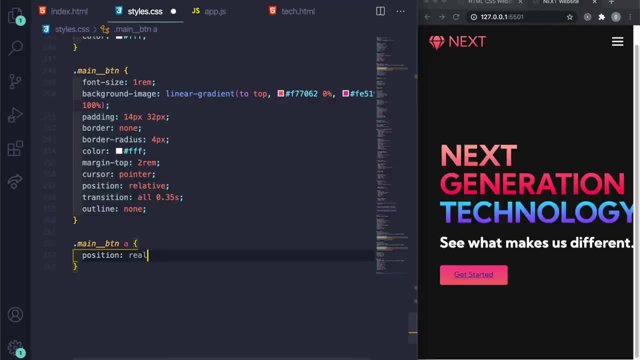 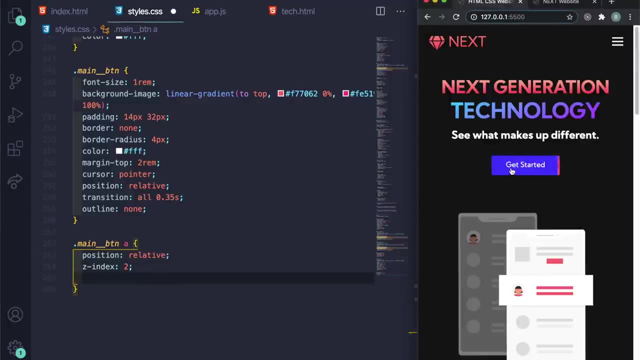 and then we're going to do position relative here and let's just do z index and the reason we're doing this is because of that hover effect. so it's normally not necessary. but since we're doing a little hover effect action we're doing in the previous, let me show you, sure, like that we have to do all these like c index stuff. 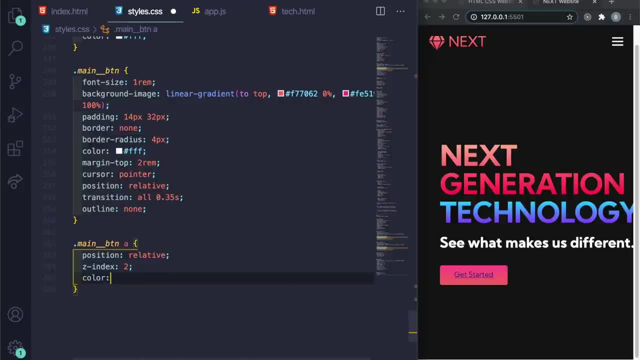 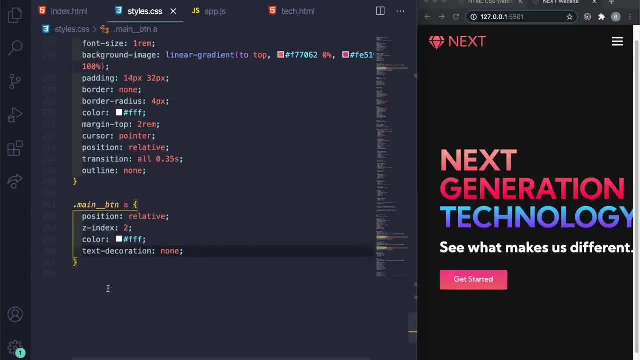 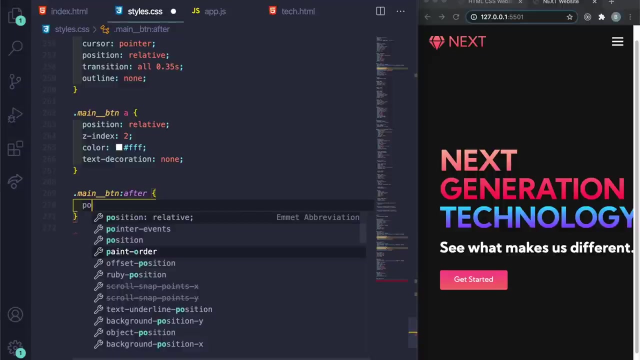 and then let's do color to be hashtag fff, and then text decoration to become none. all right, looking a little cleaner. and let's do dot main underscore, underscore btn, colon after- and this is essentially going to place these values after in the actual. you've seen the html when you inspect the page. let's do position absolutes. 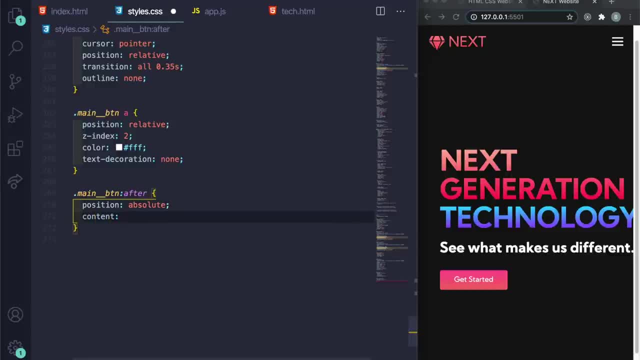 content. you want this to be empty string so that when you actually see the hover effect, like nothing's there except what the color is top, you have to set that to zero for the left. you're going to set that to zero for the left. you're going to set that to zero for the left. you're going to. 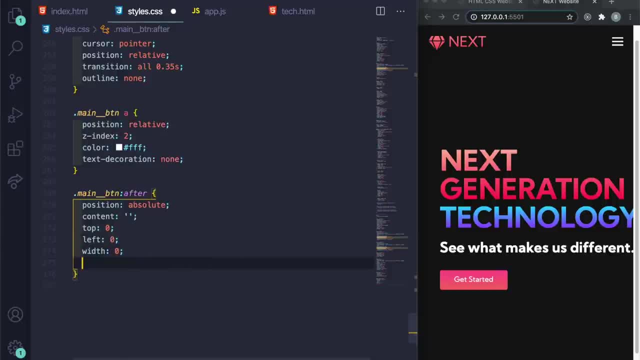 set that to zero. for the width, you're going to set that to zero and then for the height, i'm going to set that to 100, and then background is going to be hashtag 4837 ff and then transition going to be all 0.35 s and then border dash radius is going to be four pixels. 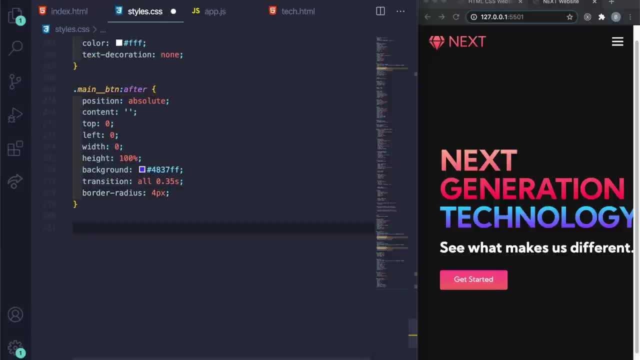 now, underneath this, let's do the hover now. let's do dot main underscore. underscore btn- colon hover and let's do color the hashtag fff. let's do the width to be a hundred percent. actually, my bad, delete the width. let's do um dot main underscore btn. 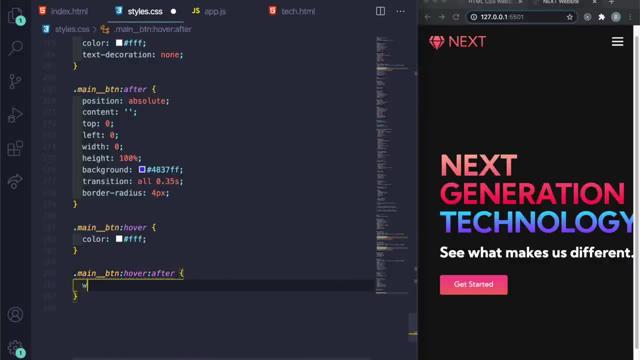 colon hover, colon after, and then let's do width to be a hundred percent and then let's do dot main underscore btn colon hover. and then let's do dot main underscore btn under. it's going to score img dash, dash container and let's simply just do text align to be center. 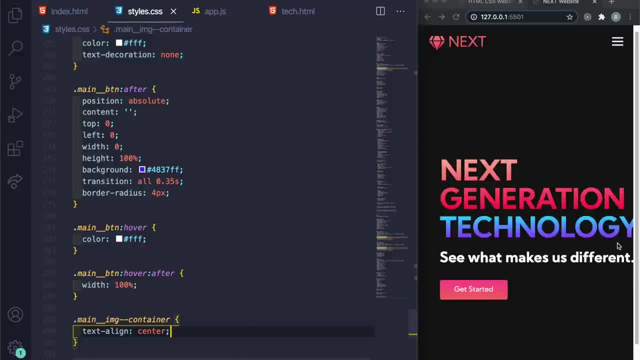 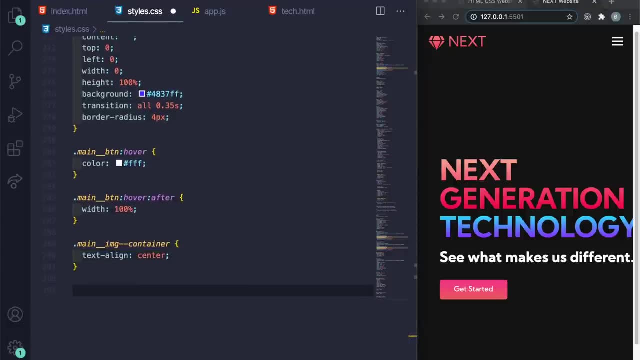 let's see if this actually pulls off. so now we have a little hover animation going on, awesome, cool, cool. and now let's finish off this before we go to our load responsiveness. let's just do hashtag mean that i'm just going to score img and let's just do heights to be. 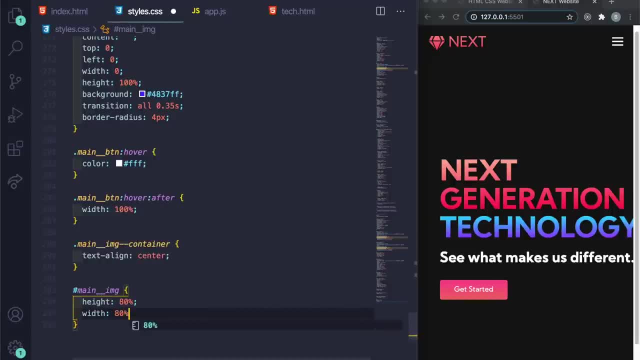 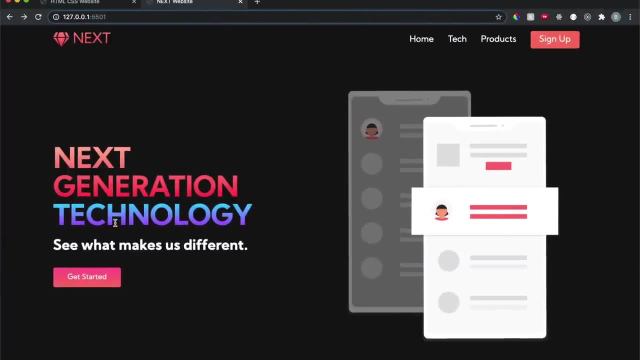 80% and then the width to be 80. so let me scroll this out to see what i got going on right now. so it's pretty much the first part, but it's not more responsive, so let's go and finish this up. so right now you can. 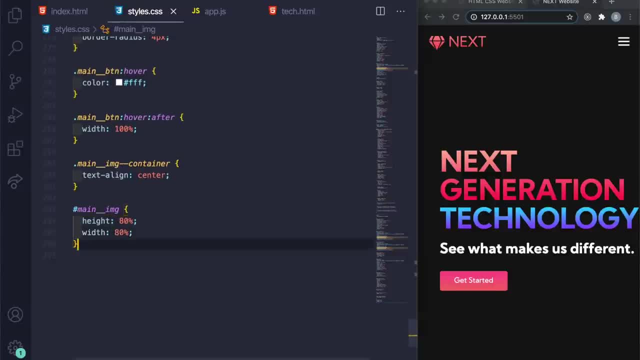 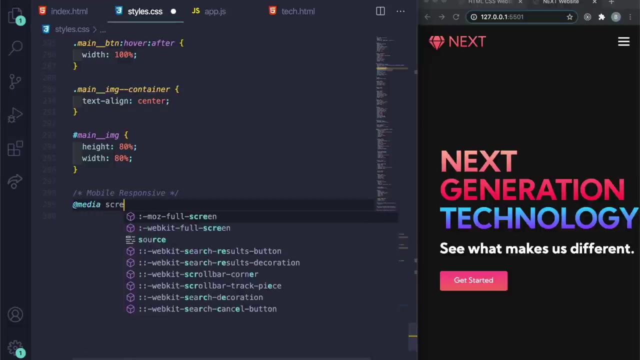 see, nothing happens yet. so here, underneath this, let me just say: this is like mobile responsive, here and now. let's go ahead and let's target the media query, so let's do add media screen and let's do max width to become 768 pixels and let's just target that main underscore, underscore, container and let's do display grid. 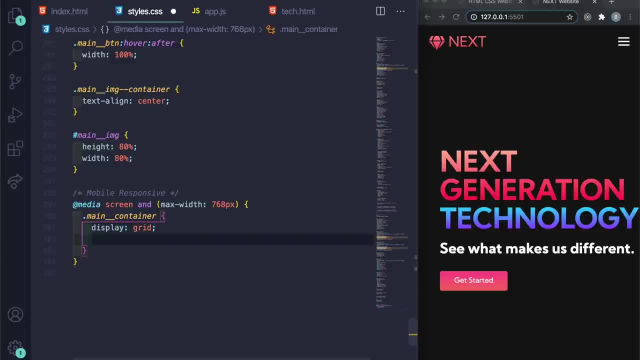 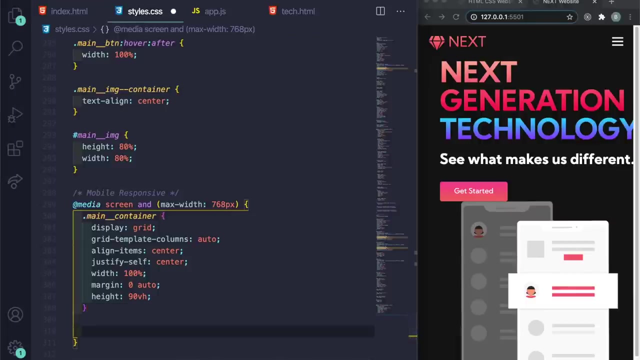 let's do grid templates, columns- i want that to be auto. let's do a line items to be center, justify, self center and let's do with a hundred percent margin, zero auto. and then let's do height to be 90 degree height. so now we got some little media query action going on. so now let's finish. 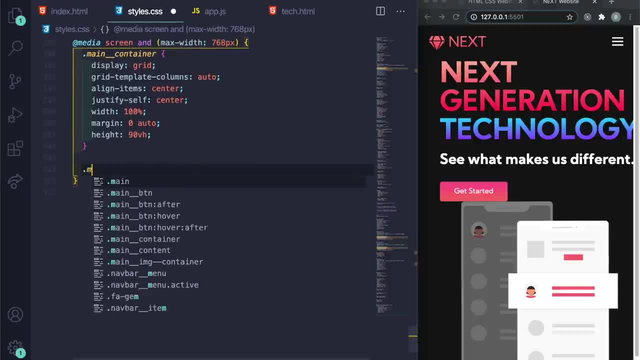 this all, let's do you? let me scroll up. let's do dot main underscore underscore content and let's just do text align to be centered, margin dash bottom to be for rem. and now let's do dot main underscore underscore content: h1 and let's do font size to be 2.5 rem and then margin dash top to become 2 rem. 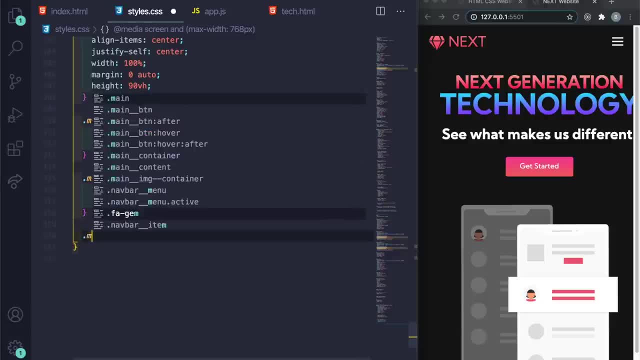 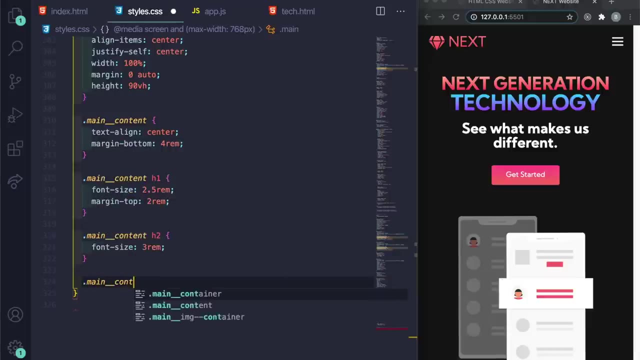 and then let's do dot main underscore underscore content h2 and let's put that as font size to be 3 rem. and then let's do dot main underscore underscore content p and let's simply do margin dash top to become 1 rem and then font size to be 1.5 rem. so let's do that. and then let's do dot main underscore underscore content h2 and let's put that as font size to be 3 rem. and then let's do dot main underscore underscore content p and let's simply do margin dash top to become 1 rem and then font size to be 1.5 rem. 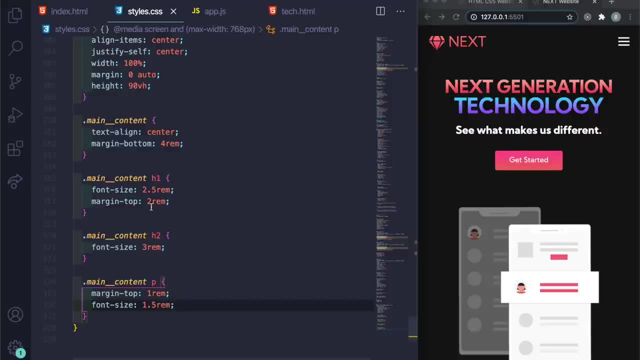 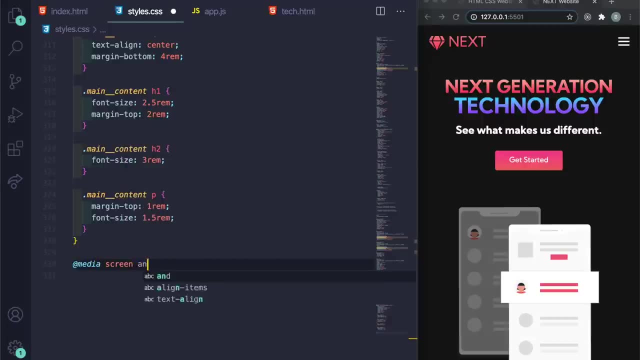 and then font size to be 1.5 rem, and then font size to be 1.5 rem. and now let's go under here and let's do another media query. so let's do add media screen and let's do max width to be 480 pixels. so these are for, like, the smaller screens. 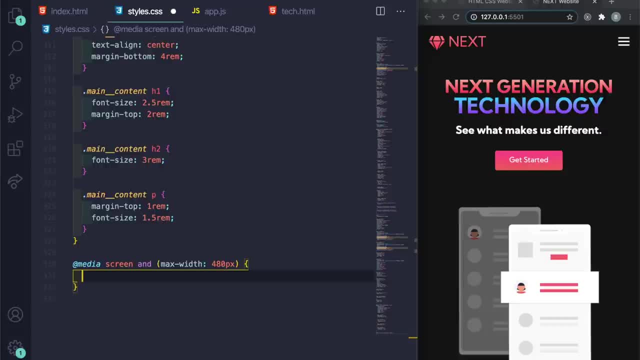 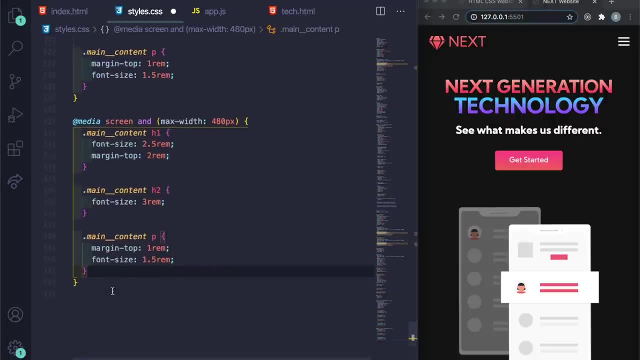 and let's just copy the content: h1, h2 and the p tag, so i don't have to sit here and copy this again. so let's just copy these and paste them. and now we're going to do, we're going to change this to: let's do. 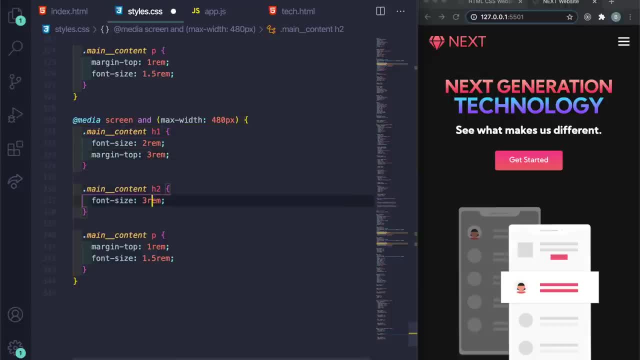 2rem and then 3rem, and then for the h2 let's do 2rem, and then for the p tag let's do um 2rem, font size 1, fiber, and then underneath the p tag let's do dot main 1, underscore btn, and simply let's just do padding to be 12 pixels by 36 pixels and then margin to be 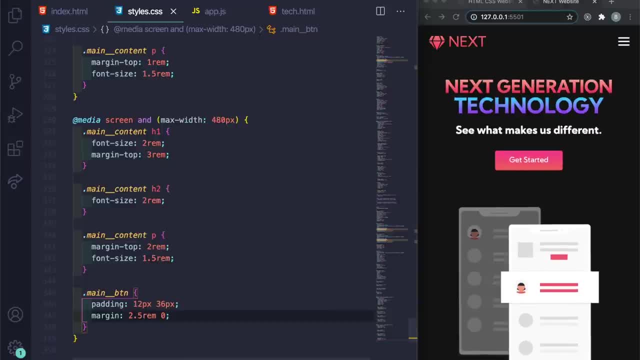 2.5 gram by zero. so let's save that, and we are pretty much set with this hero section right now and we can scroll. got nothing yet, but we can see we've got a mode menu and that's pretty much this section, so let's now go ahead. 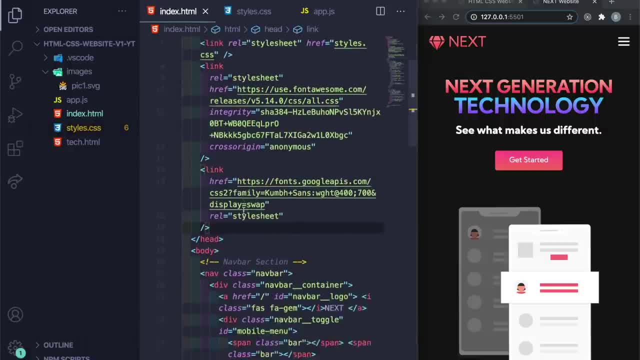 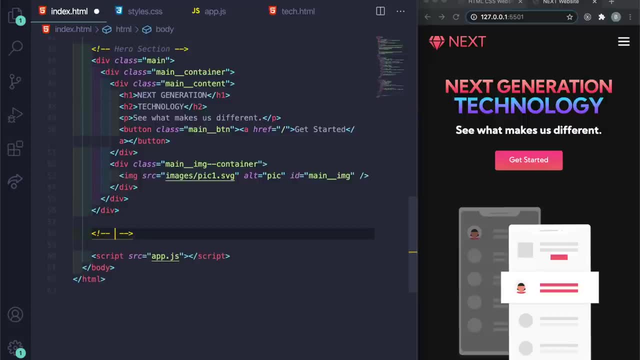 let me command b, go to the nshml and let me actually go ahead and finish and let's add the services section. so, underneath the hero section, let's go here and let's just call this one services section, alright? so now i'm gonna go under here and let's 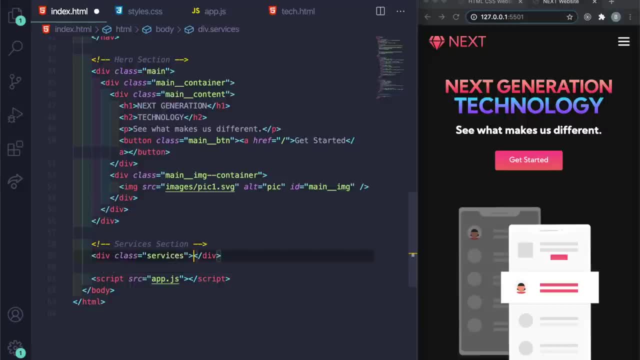 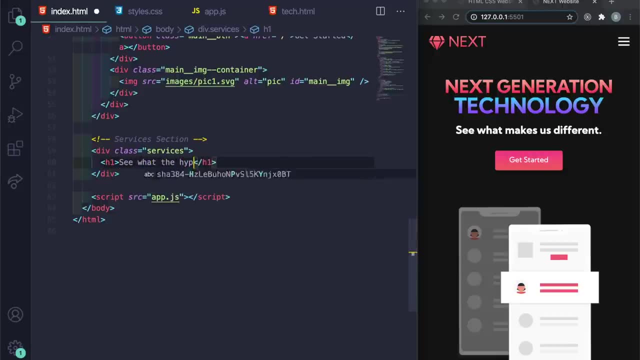 start adding this. i'm going to say dot services press tab, and then in services, let's just do h1 and let's just say: see what the hype is about. and then, outside of this h1, press enter and let's do dot services- underscore, underscore, container. and then in the container i'm going to create, 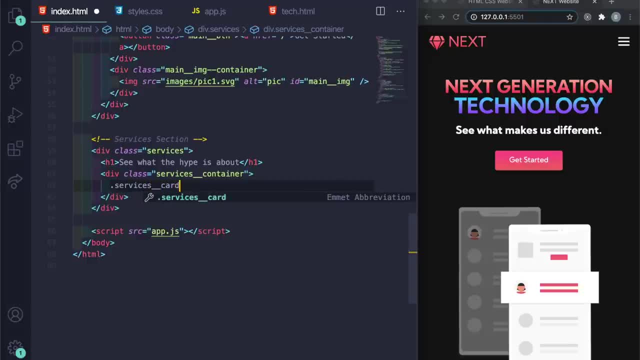 a services car. so let's do services, underscore card, press tab there, and let's just do h2, press tab x. i should take you guys experience, experience, bliss. and then let's do p tag right there, ai powered technology. and then for the button let's just do button, let's just do get started. 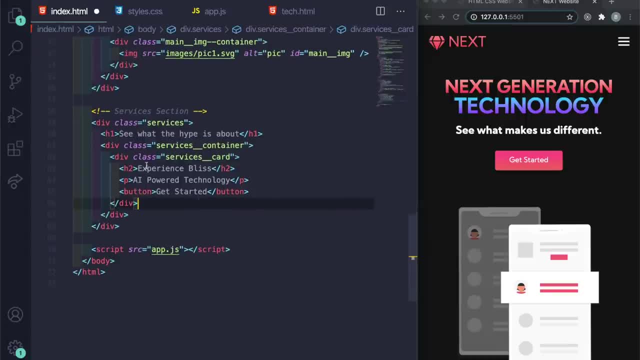 all right. so now, underneath this, so we have essentially a service card. i'm just going to copy and paste this copy paste, and then it's going to change this text here. so let's just do um, let's just say: are you ready? question mark. and then let's just say: 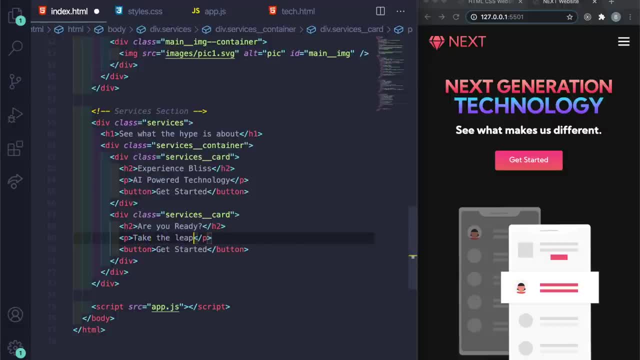 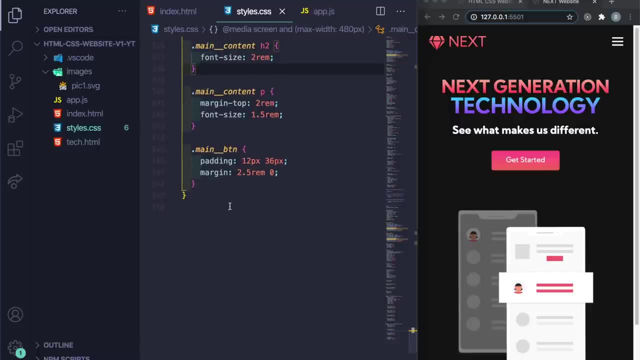 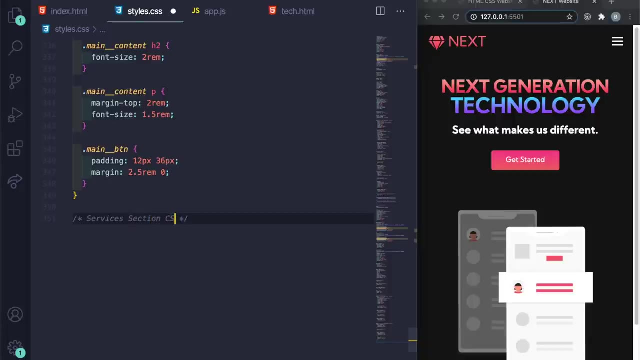 take the leap and then simply get started. so that's pretty much all the index html. so now let's go to the stylescss and under here let's just call this services css, our services section css. so now i'm going to do the services and then simply we're going to say background. 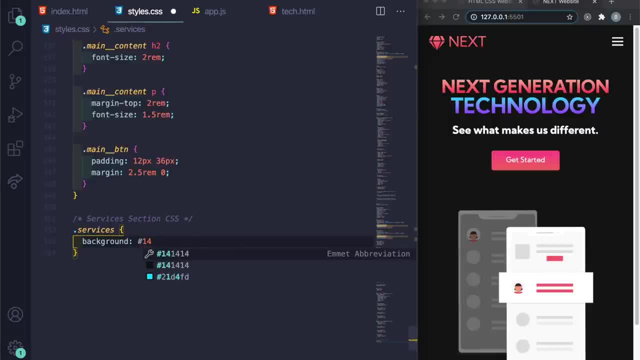 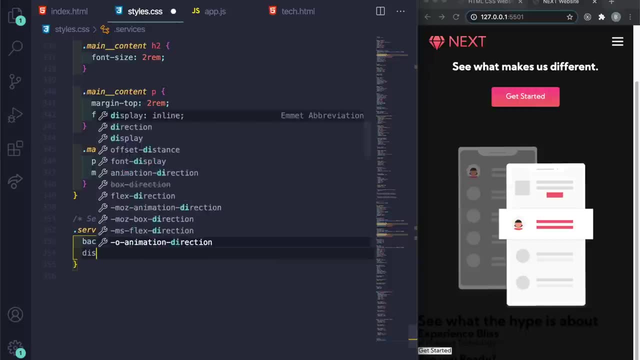 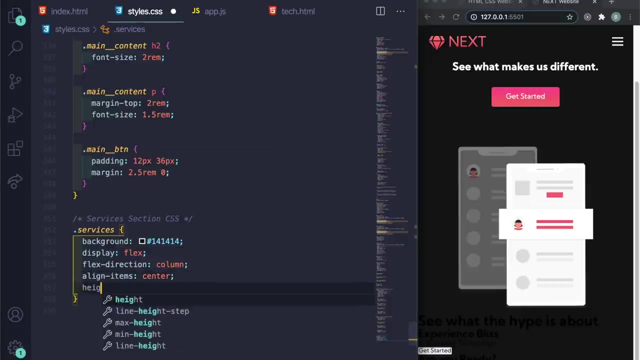 i want the color to be hashtag 1414. save this there, let's see, okay. and then let's do display to be flex, let's do flex direction to be column and then i want the actual items so align, dash items to be center and then the height to be 100. 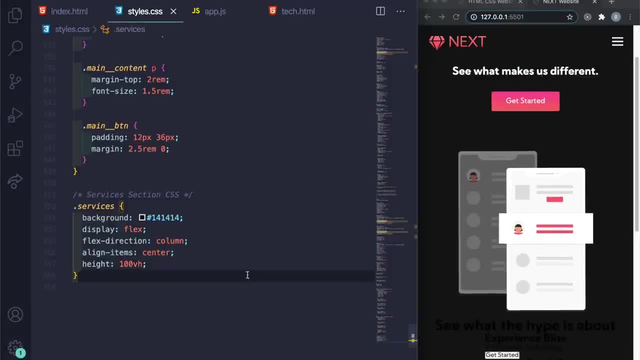 viewport height. and now underneath here, let's do dot services h1 and let's just do- uh, here's going to be a pretty crazy one- let's say background color- background-color- contrast-coloredlн. that's gonna go there. let's go tag go bit after current mech, lemme show you. 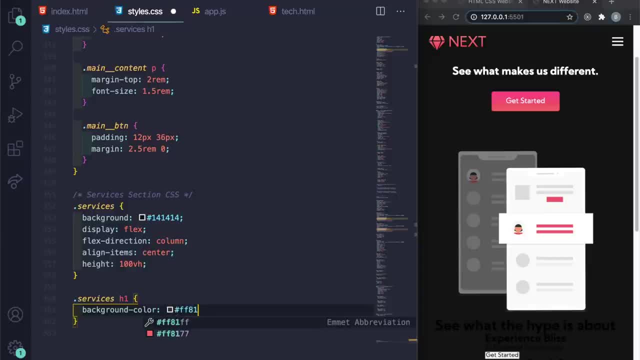 how to get that. just gonna be interesting, business card doesn't come out like a Jakob pattern. and now let's just do flex-edit. I want it to be hashtag FF8177, and then background-image, colon- linear gradient. and then I want to say to write comma and then hashtag FF8177, 0%. and then I'm going to simply let me put this on another line so you can see all this code. 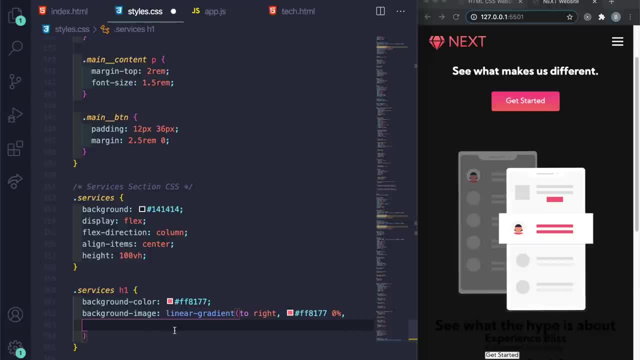 I'm still inside the parentheses and I'm going to do hashtag FF867A- 0%, and then hashtag FF8C7F- 21%, and then comma hashtag F99185,- 52% and then hashtag CF557A. 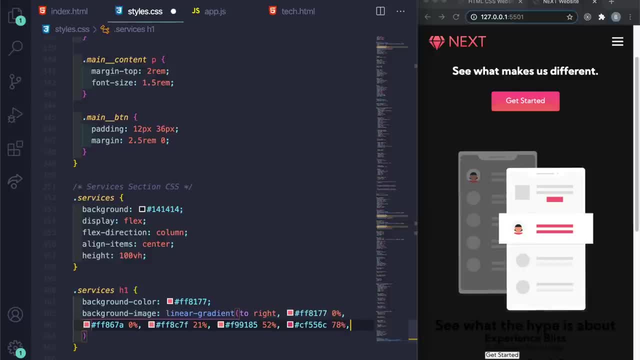 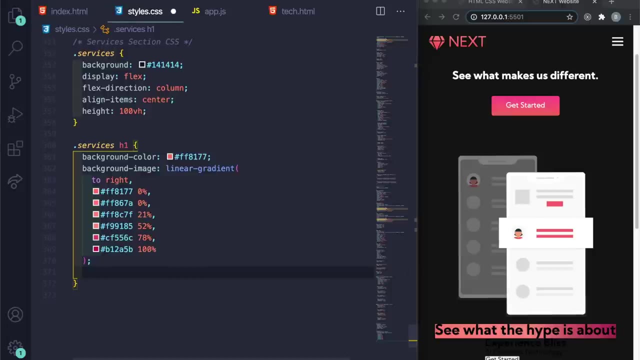 FF86C- 78%. and then last one hashtag: B12A5B with 100%. So I'll save that there and then you can see we got the gradient right there. and now let's go underneath that. Let's do background-size to be 100% and instead of me having to copy and paste this every time, let me finish this off. 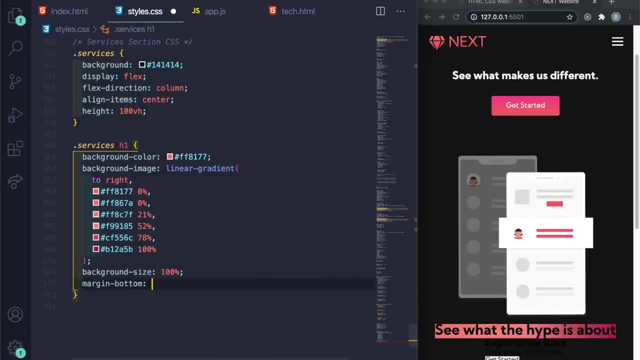 Let's do margin-bottom, So this would be 5rem and then font-size to be 2.5rem. So now I'm going to go back to the top, where we did our original linear gradients. Let me see if I can find one. 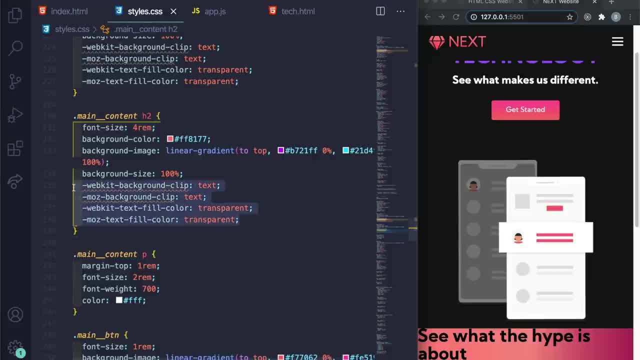 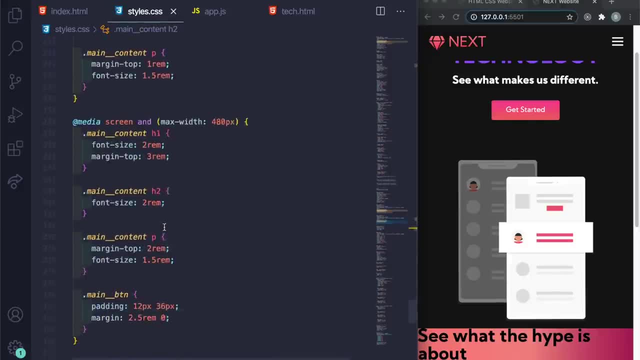 Like right here and I'm just going to copy these last four lines here. So essentially WebKit background text, everything here. Let me just copy these four, go down below and then just simply enter here. All right, 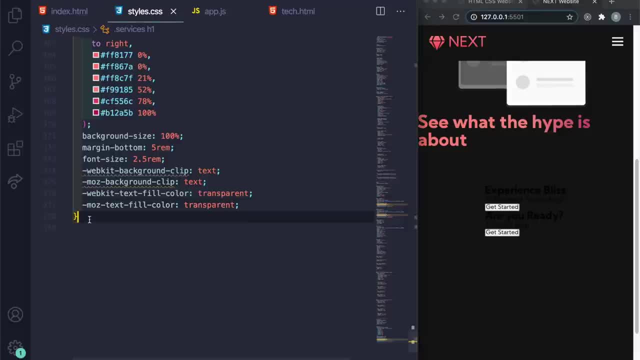 I got the text looking like this. So now let's do services. I'm going to just go underscore container and then in here I'm going to do display to be flex, justify content to be centered, and then the flex wrap is just going to be wrap. 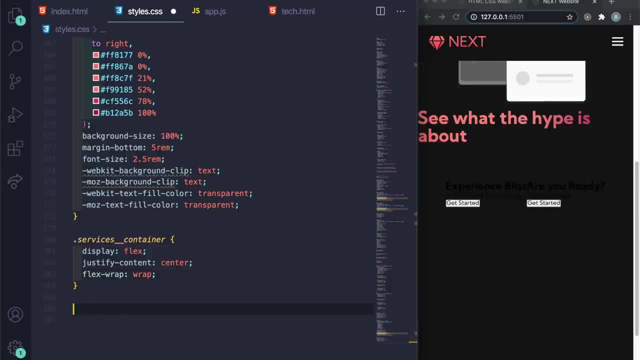 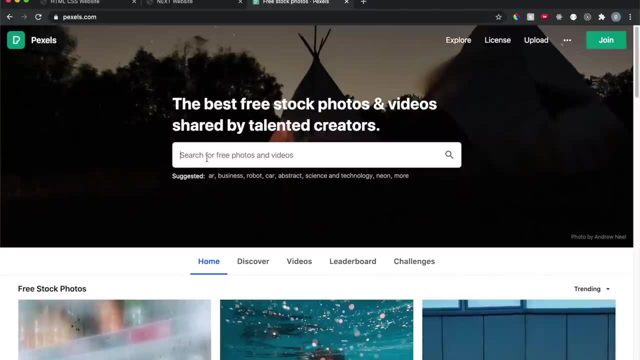 So you can see they wrapped. and now for the card, let's do the. we actually have to get images, So let me show you the site I got these images from. So this is just one of the sites. There's multiple ones you can use, but simply I think I just typed in like VR. 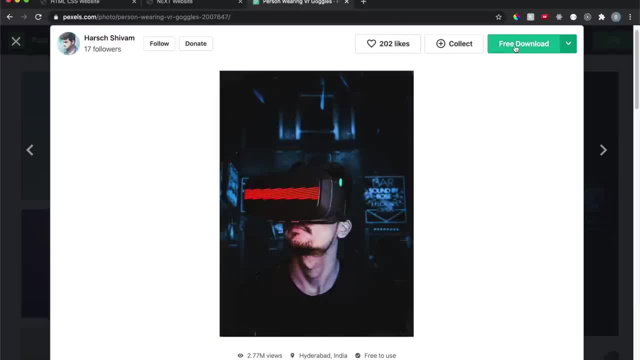 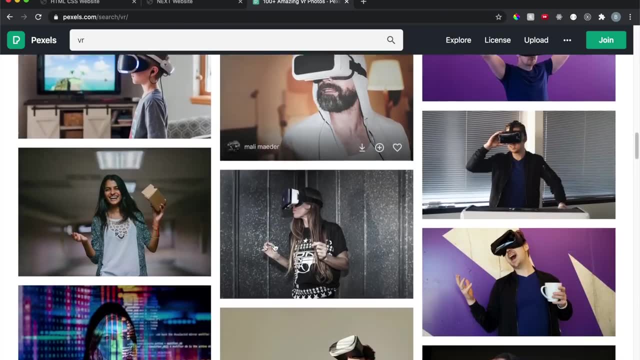 And you can go here, click on this guy right here, download it for free and then simply drag that over to your project, And then I think there's another. let me see if this person- it should be on the front page. 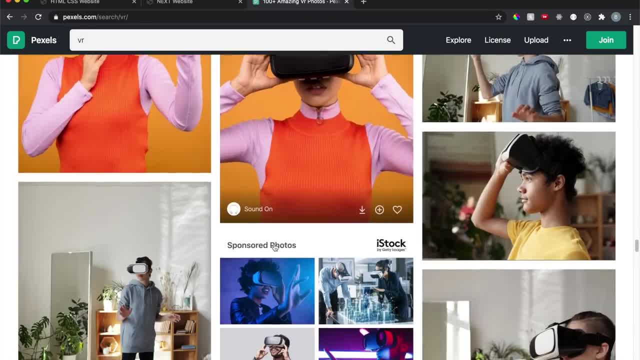 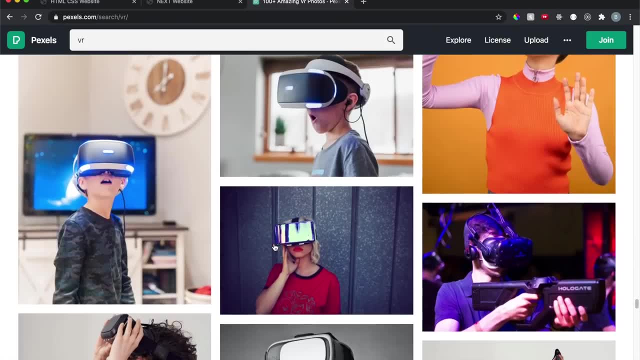 But you get the point. You can literally pick whatever you want, but let me make sure I can find it so that you can actually utilize this. So somewhere over here, let me make sure. yeah, this one right here, Just click on that one and then just re-download here. 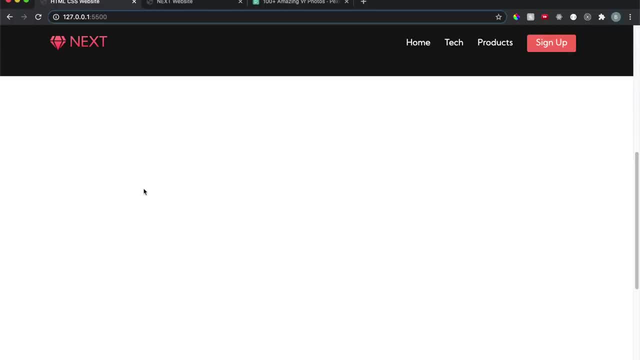 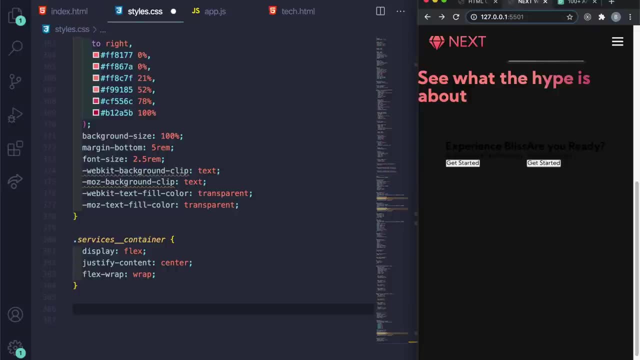 and then you'll have the exact same pictures I used, which were once it was: yeah, these two right there. So let me scroll this back, So download those and then rename them. So I simply got pick, simply pick two and three. 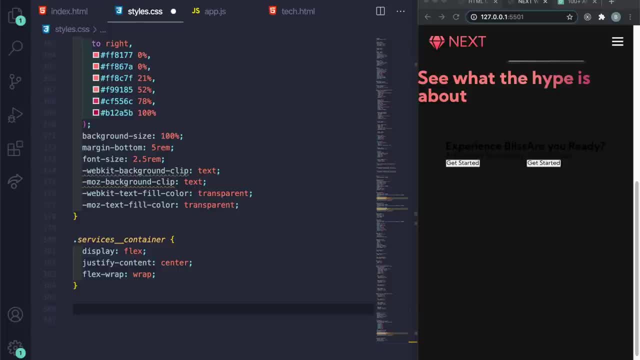 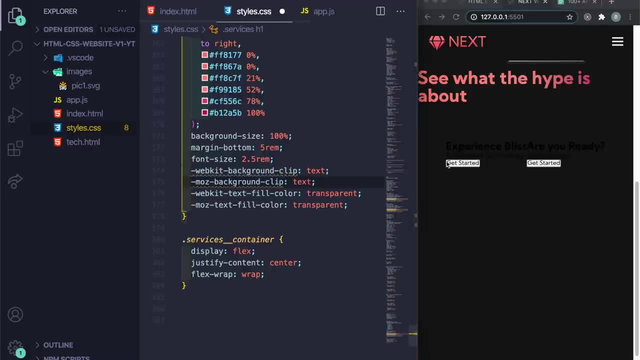 And then I'm actually going to drag in the other picture for a detect. That's not mandatory because I'm just showing this for example purposes, but if you wanted to do it, let me bring back my images folder and then let me just drag these over to the images. 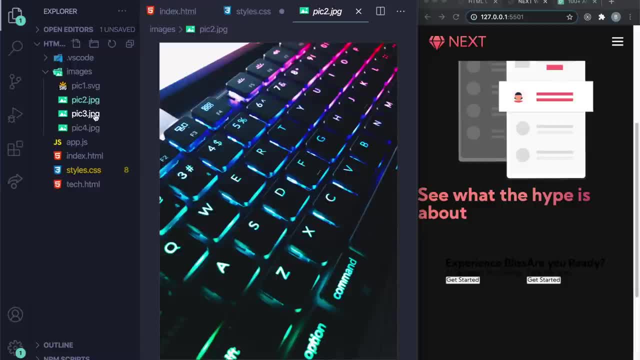 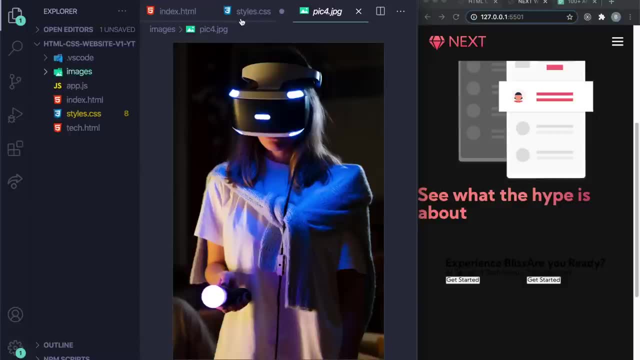 So I simply got another picture So you can download this as a keyboard or typed in. and then we got the pick three, which is the one guy with VR and then the one girl here. So now we need these images because we're going to actually add this into our cards now. 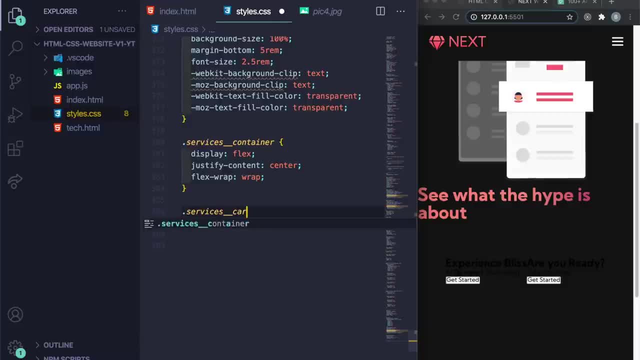 So I'm going to say services__card And then I'm going to say margin one rem. so it's the margin one rem. Let's do a height of 525 pixels, Let's do a width of 400 pixels And then let's do border-radius to be four pixels. 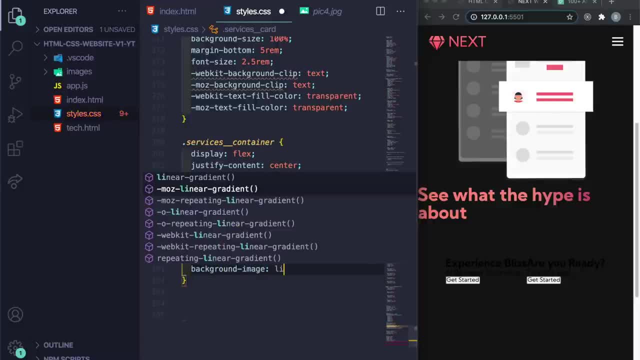 And then let's do background-image, linear gradients to bottom, and let's just do rgba: parentheses: zero, Comma, zero, comma zero, comma zero. And then outside that parentheses, you're going to say zero parentheses, zero percentage. 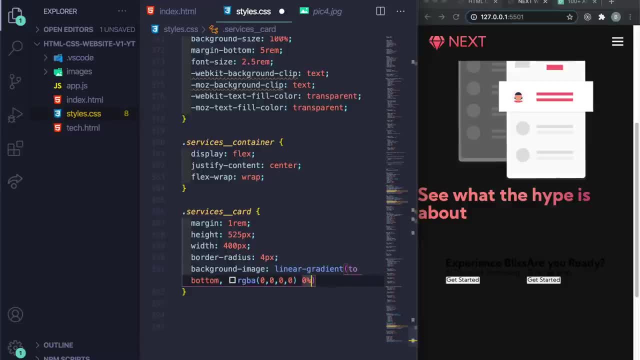 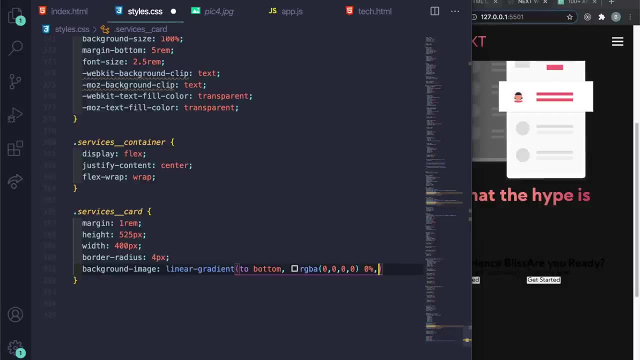 sign. And then we're still inside of this. So let me- maybe you can see what's going on- Drag this out. So then I'm going to say comma, Let's see, yeah, comma here. And then I'm going to say rgba- parentheses- 17,, comma 17,, comma 17,, comma 0.6.. 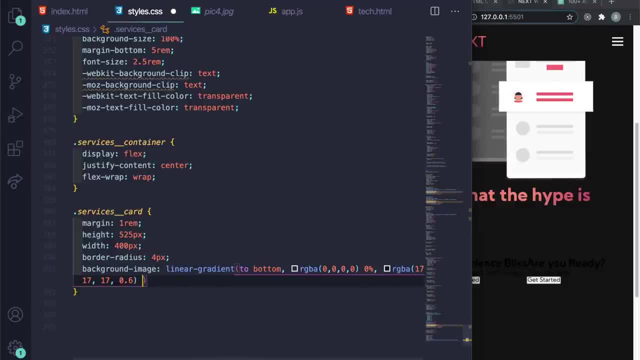 And then I'm going to say rgba, parentheses 17,, comma 17,, comma 17,, comma 0.6.. you're probably like what the heck is this? essentially it's a linear gradient on the background to make it a little darker, because it's when it was too bright, when i had the text that 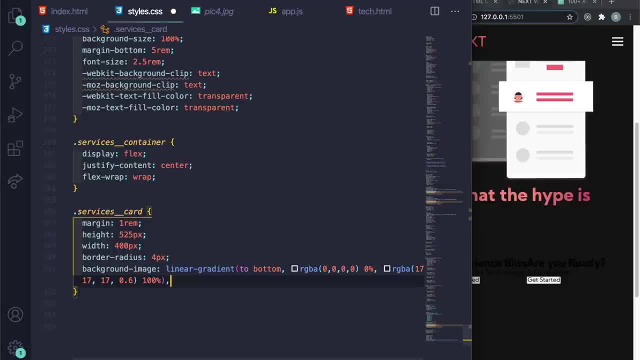 you couldn't even read it. so this is essentially doing that right here, this effect. and then, while we're still actually, let me make sure i have the right um parentheses. yeah, so we're still in the background image, but we went outside the linear gradient, so come after that i'm gonna say url. 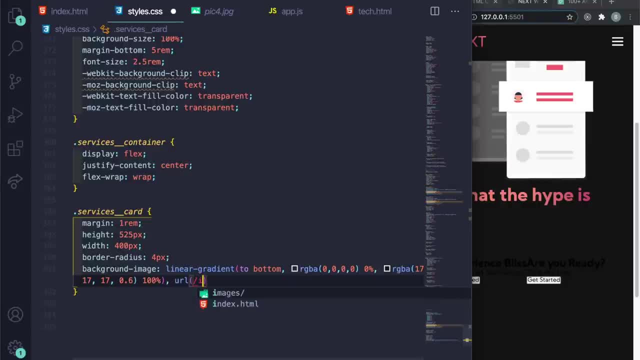 parentheses and we're gonna target the image. so slash images. actually you have to put quotes, so let me make the code: first: slash images, slash pick. i'm gonna use pick, i think three, yeah, dot, jpg and then semicolon after and let's save this and you can see. now we have the images showing up, but they 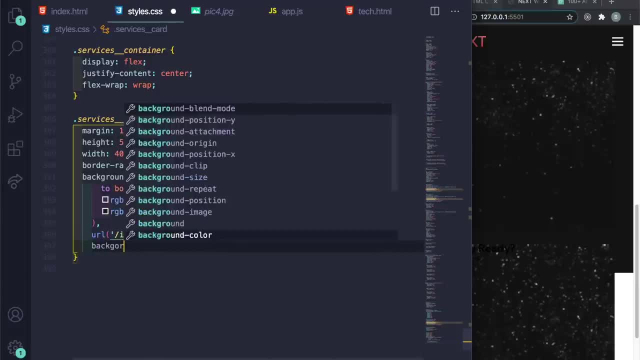 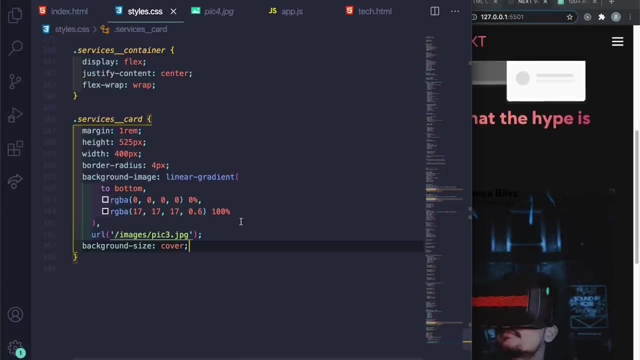 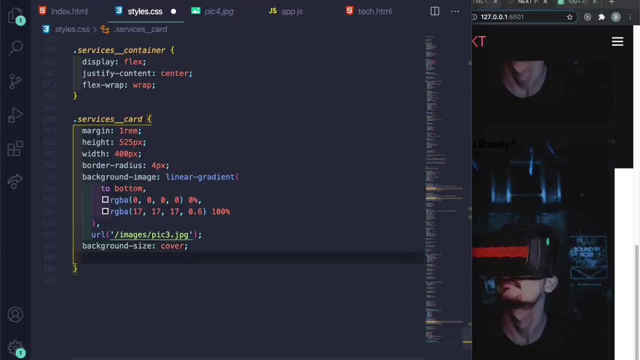 look really crazy. so what we're going to do is we're going to say background, let's do back dash side and i want that to say cover. so now you can see we got our images nice and snug and you're like wondering why is they're both the same because we haven't added the other one. let me just say 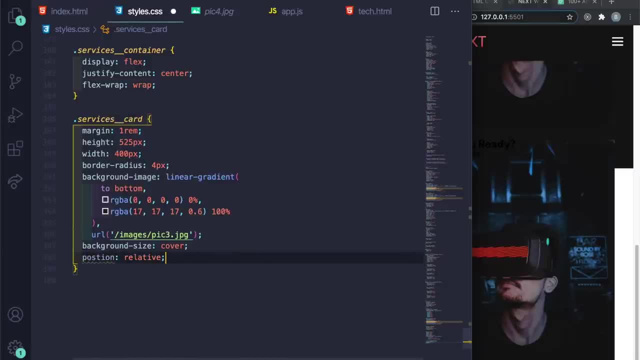 position relative here, because i want to actually- um, i'm going to fix this position relative. i want to make sure i can position the text where i want it and then just say color hashtag: fff. so this is the first services card here. and now what i'm going to do is i'm going to say dot. 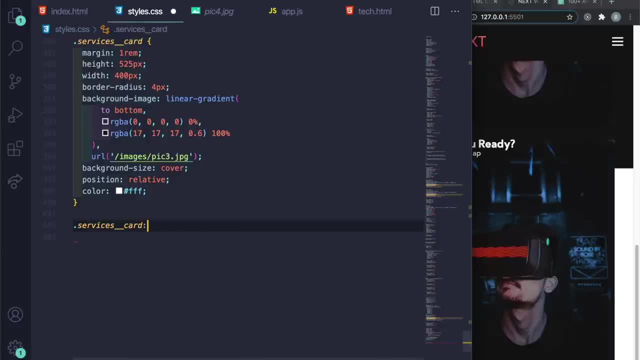 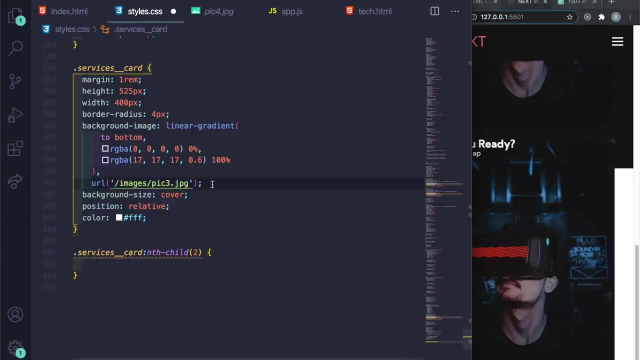 services- underscore- underscore card colon. actually, no, we don't need this, let me just do dot services underscore underscore card colon- nth dash child and i'm gonna target the second one. so obviously this is our second uh card and let me just copy this exact stuff here with this um background image. 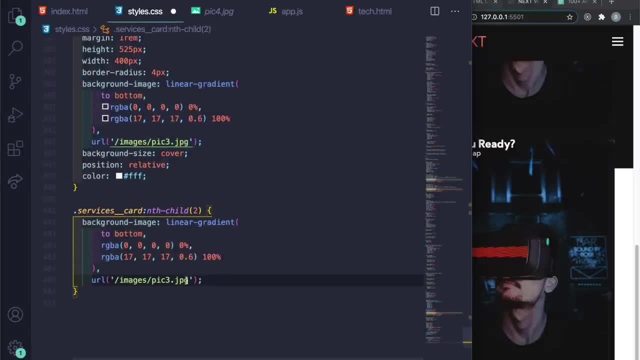 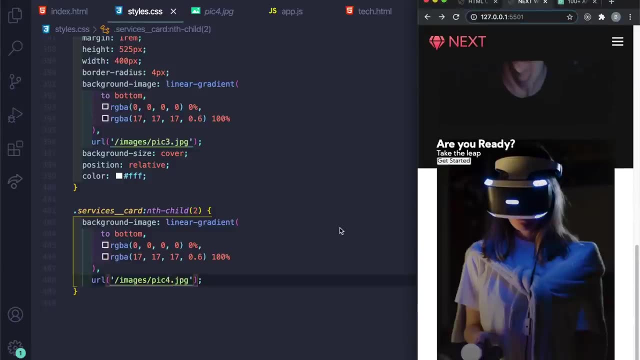 so just copy this one right here, paste it there and just change your picture to. i have mine. it's pick four, but whatever you named your girl, vr, pick is what you name here. and then let's go underneath this, and i was going to say: dot services, h2, position absolute. let's do a top and i want. 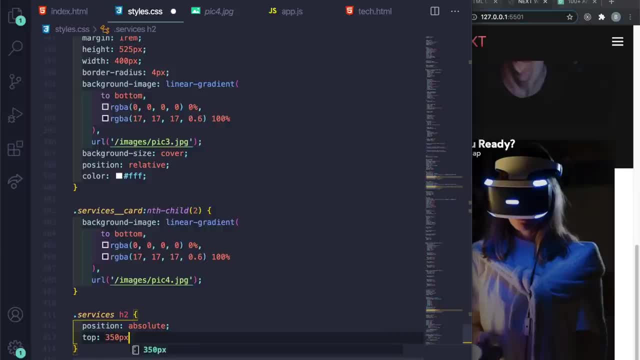 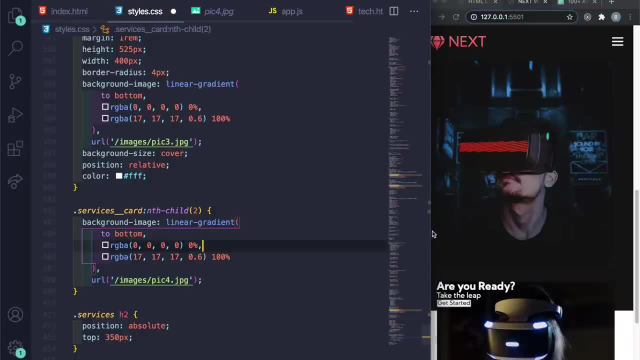 to bring it down. i want to bring down 250 pixels, so if i save, let me show you what's happening. so i saved our this up here to 20. you should save it now and you should also create this altered's死, and if you don't, you can add it down at this point and tap to set it up. 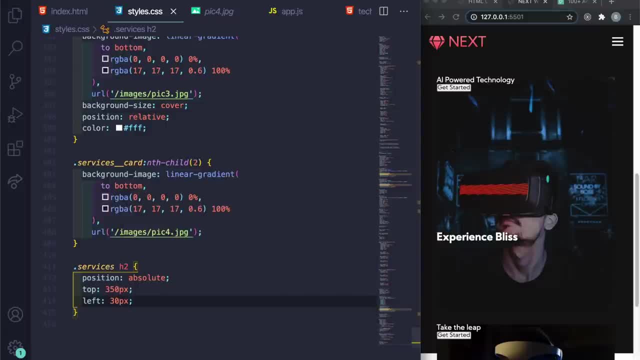 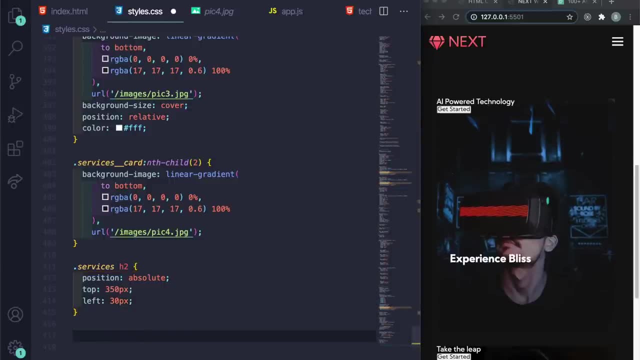 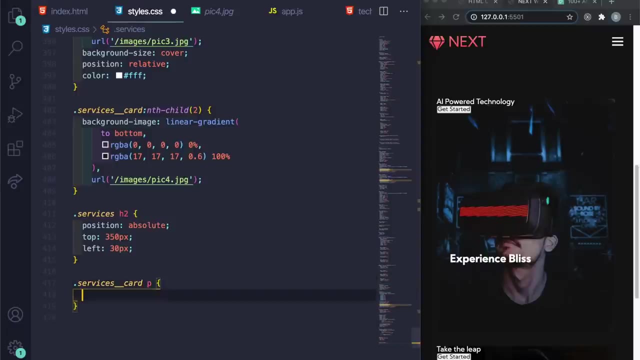 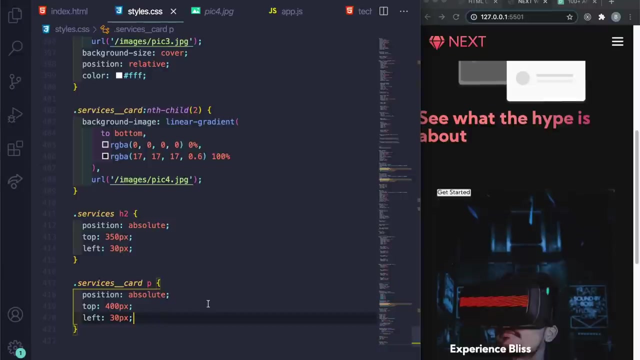 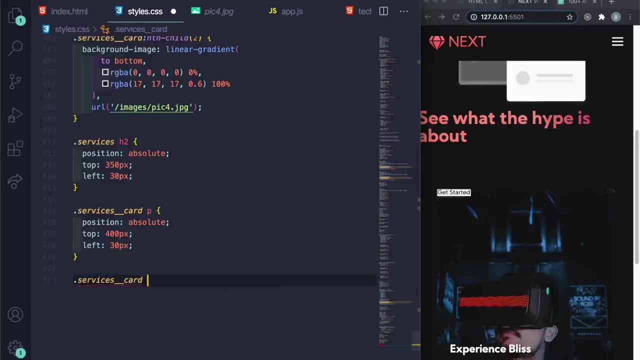 then, um, let's교i do dot services, underscore, underscore card, p tag, and let's just say position absolute again. so, position absolute, let's do top 400 pixels, and then let's do left to be uh, 30 pixels. and now let's do dot services, underscore, underscore card button, and let's target the. 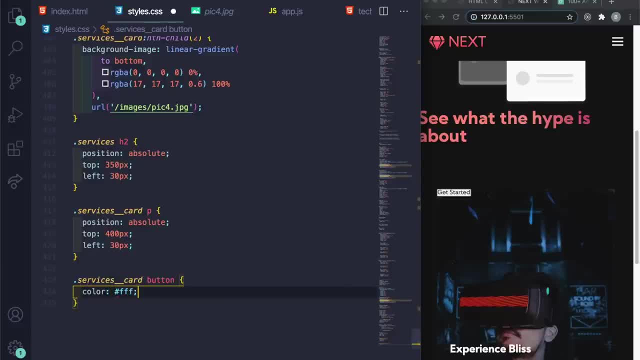 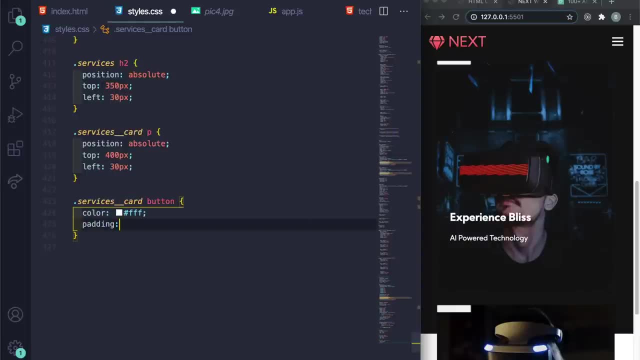 color. let's make it um hashtag: uh, fff. so text is white. and then under here, let's do padding to be 10 pixels by 20 pixels, let's do border to become none, let's do outline to become none and then let's do border dash radius to be four pixels. background is going to be hashtag f. 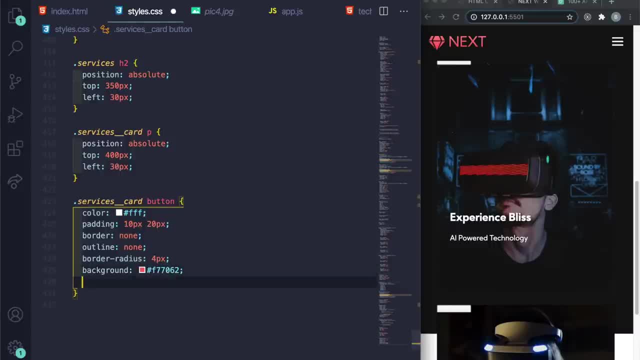 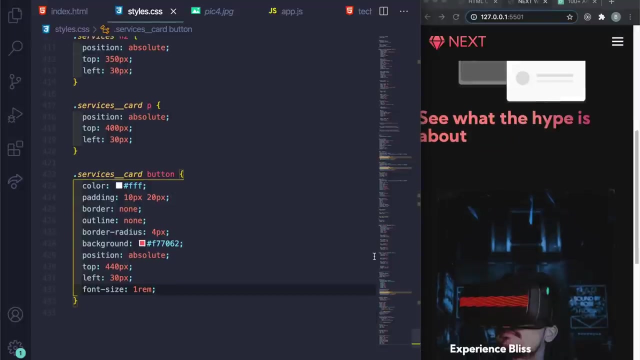 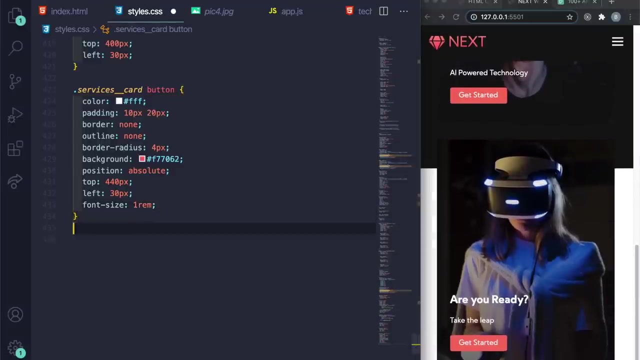 seven, seven, zero, zero, six. two. position is absolute. top is 440 pixels and then left is 30 pixels and then font size is one rep. so now let's check it out. we've got a little button action going on here and the same on this picture or the card there, and then simply let's just do um cursor pointer two. 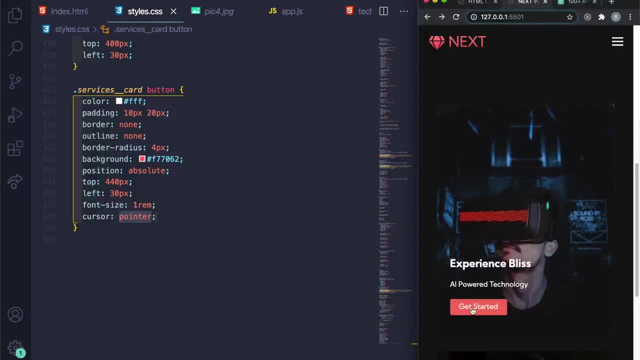 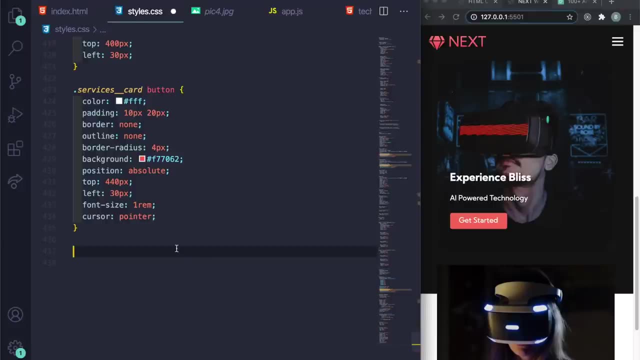 so let's make sure it actually has it there. so perfect, all right, cool. and then now let's just do a little effects when we hover over it, so let's do services on. it's going to score card colon hover and this is going to scale it. so increase the size, so transform. 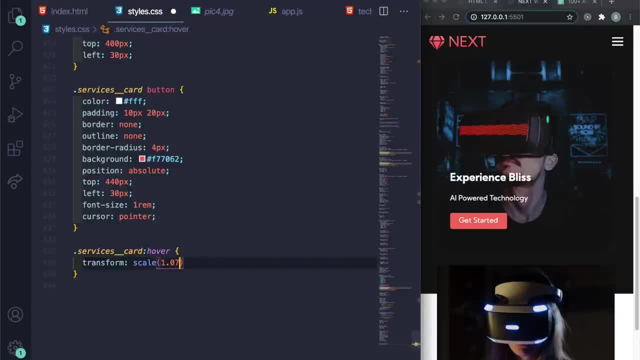 and then i'm going to say scale- parentheses- 1.075. make sure i'm going to go outside here and let's do transition. to be transition, that should be 0.2 s ease dash in. let's do cursor pointer here and now. if you hover over it, you can see. 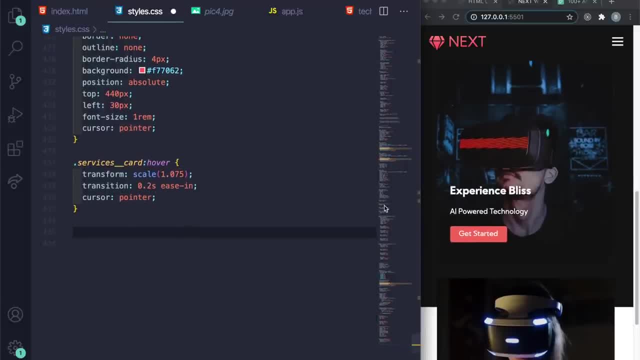 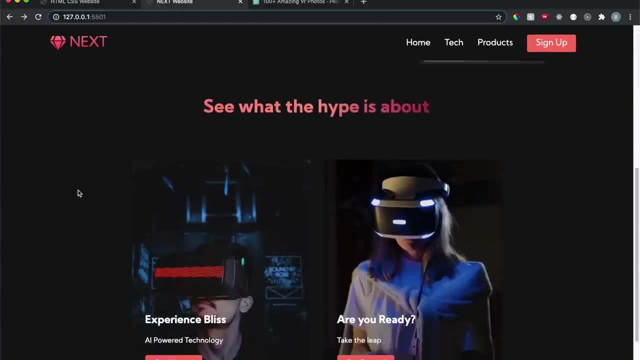 that is increasing in size. and now let's go ahead and just add in the media grease. so right now, if I were to go back, see what we built so far, got this, and then we got this right here with the little hover effect. so now let's go back. 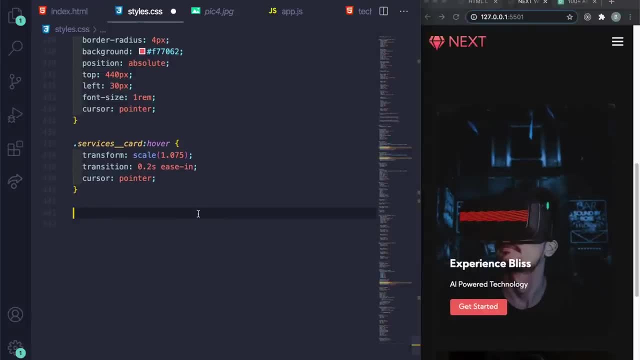 and let's do at make sure at media screen and max dash with to be 960 pixels and let's just do dot services and let's make that a heights of 1600 pixels and let's do dot services of h1 and let's just do font a size to be too. 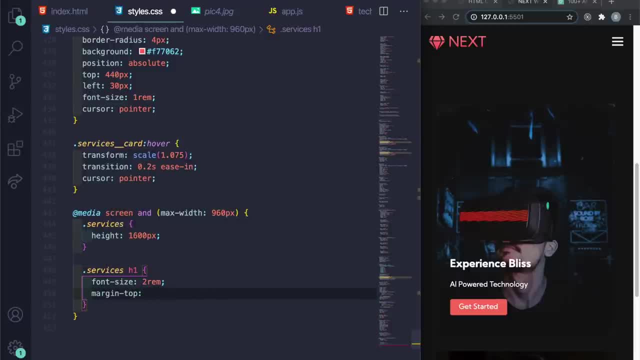 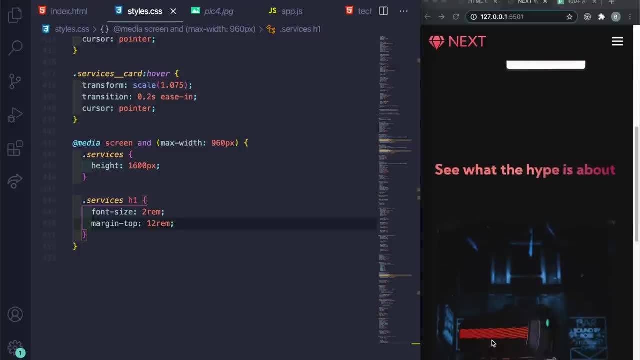 late Ram and then let's do margin dash top to be 12 for him, And I just wanted that because it's like a little close when you shrink it and I want to make sure that I have pipe And then also on the footer when we create that, I want the bottom to have spacing too. 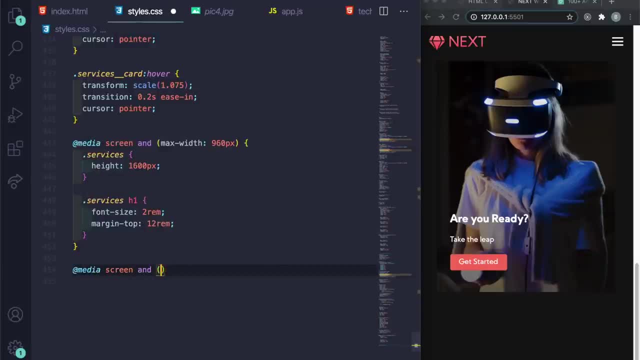 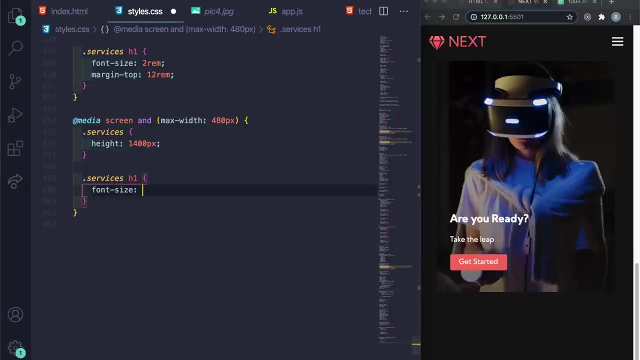 and then let's- last last one, add media screen and max width to be 480 pixels toward the smaller screens, and that should do dot services. let's do a height of 1400 pixels and Then let's do dot services h1 and let's do font that size of 1.2.. Ram and 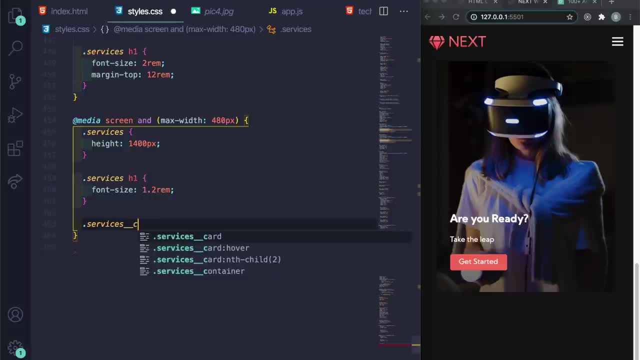 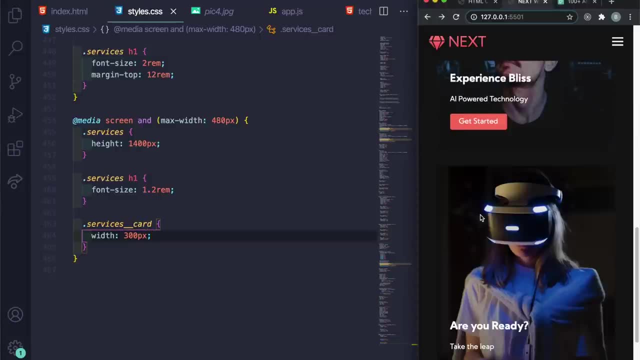 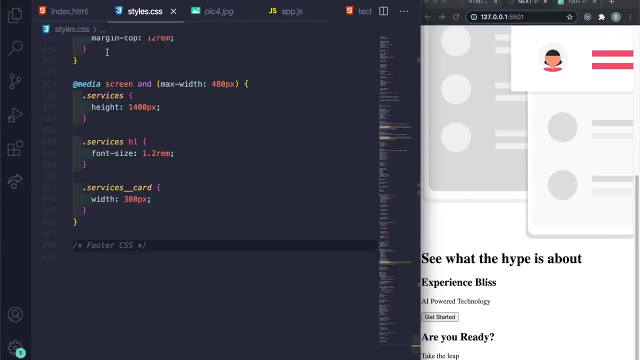 Then let's do dot services, underscore, underscore card, and let's do with of 300 pixels And it looks like we're good here and now let's go ahead And let me add another comment here and it's gonna say: footer CSS. So now let me command B and cool a trick to is um. 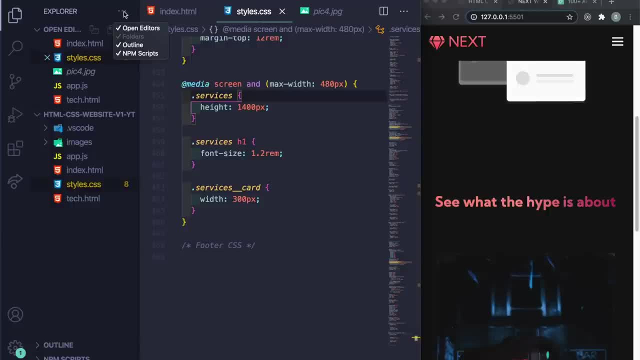 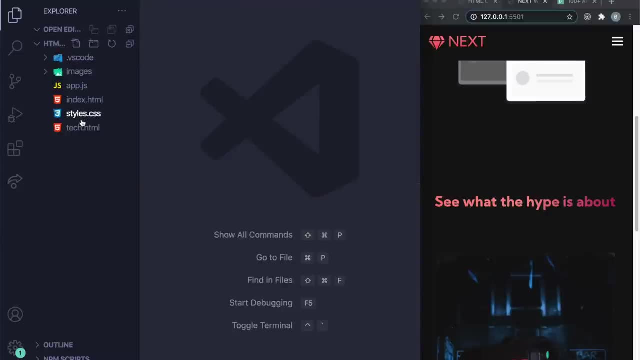 See, I've got all these tabs open if I click on open editors. If you don't have that setting, click on these three dots and just click on it. check it. I can just click the X here and it cleanses out everything. so now I have a fresh slate. 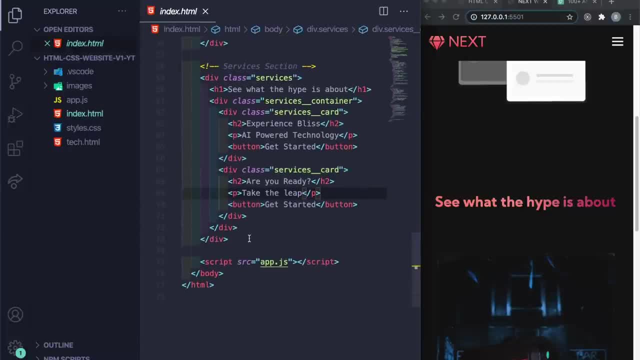 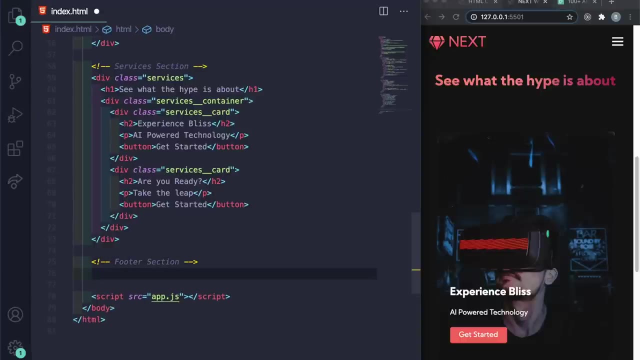 So now go back to in a same HTML, Unless you go ahead and go under here and let's just do a footer section. so now let's just simply go to indexhtml, all right. so let's start adding the code for the footer. so let me close this out and scroll up. so here i'm going to say: dot- footer underscore. 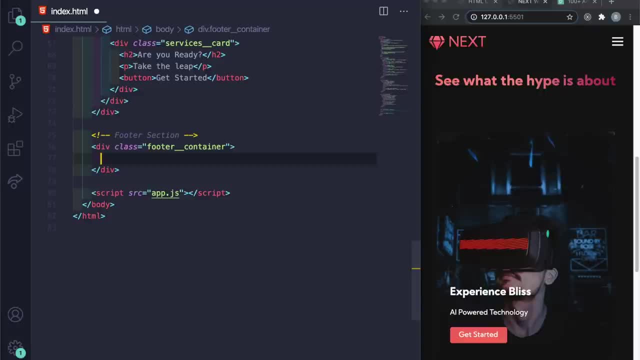 underscore container and then create a div called dot footer, underscore, underscore links, and then inside here i'm going to have dot footer, underscore, underscore link, dash dash wrapper, and then let's do dot footer, underscore, underscore, link, dash dash items, and then in here is where we actually start to add the uh footer stuff. so let's do h2. i'm just gonna say this about: 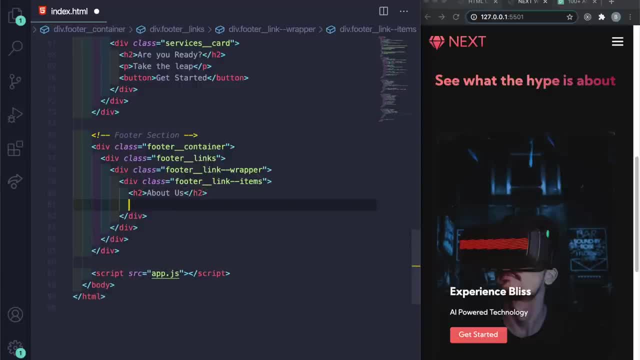 about us, and then in here let's just do an h or an a tag with the just put a slash for here, and then let's just say how it works, and then we can simply just copy and paste this. so let's do one shift again. let's shift alt and down arrow to do what i'm. 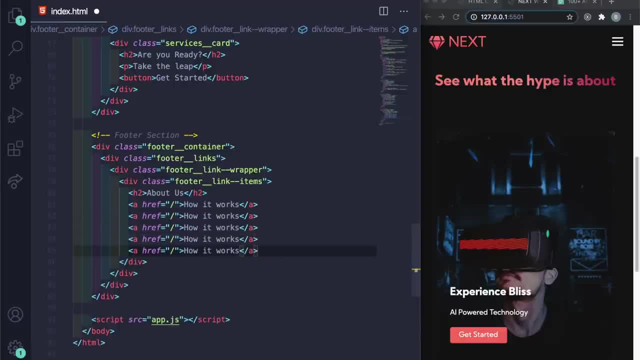 doing here. so two, three and four, so five times total, and then simply let's just go here and let's just say testimonial, let's see testimonials. the next one: let's change this to careers, and then let's do, let's see, let's do investments, and then let's just do term of service. 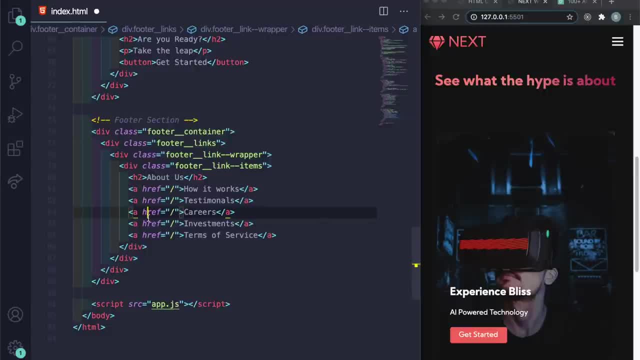 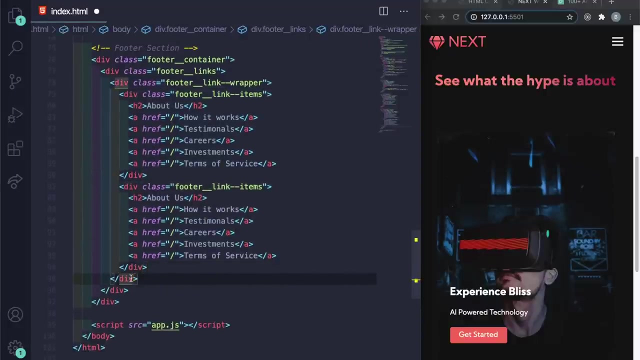 now this, pretty much, is what we need to do for this. so now i'm going to go ahead and take these footer link items with the all the things we just created, command c- and then paste that. so now we both- we have the footer link wrapper and then we have two of these inside of it, and now all we need to do is get the. 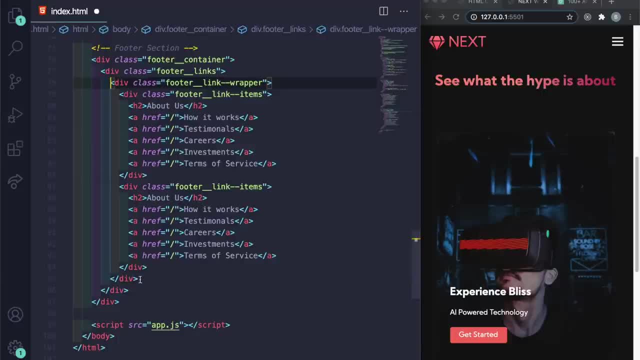 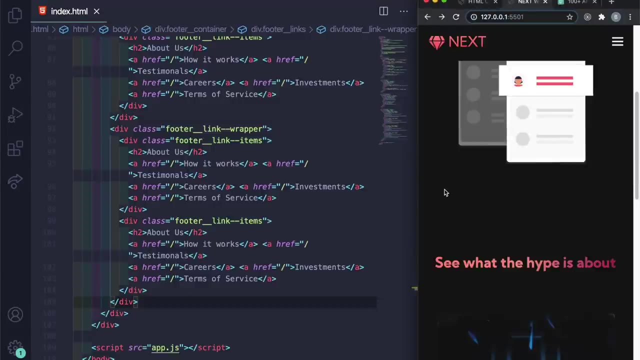 footer link wrapper now and then highlight. so i have a plug extension for this to highlight this, but pretty much get everything wrapped with the footer link wrapper, command c, then go below and then paste that again. so now, if i save it, we should have a footer link wrapper and then paste that, just drag and drop. let's go down here when we go below. 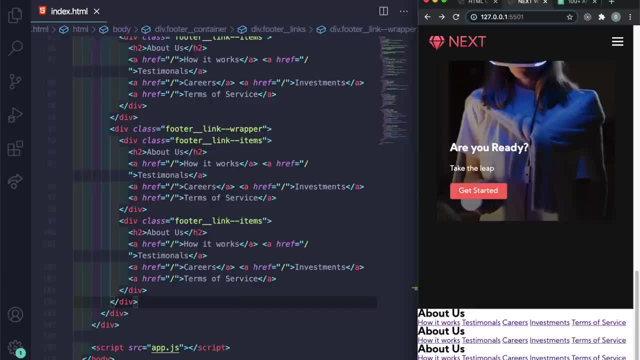 we want across all the flip side. it's this cross here and then use the same gently, push this down and here is the ok. so this is where we want just to hit this left pre exp only button. so we're just going to try to get own city of this. 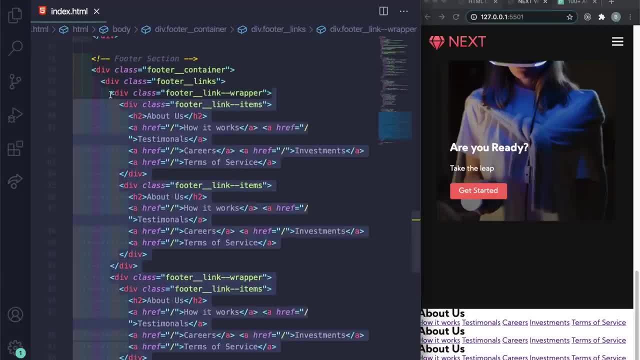 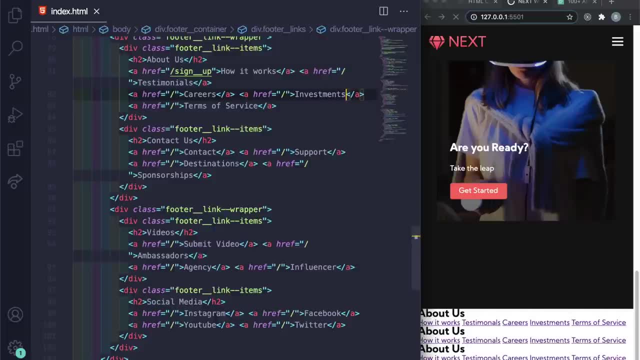 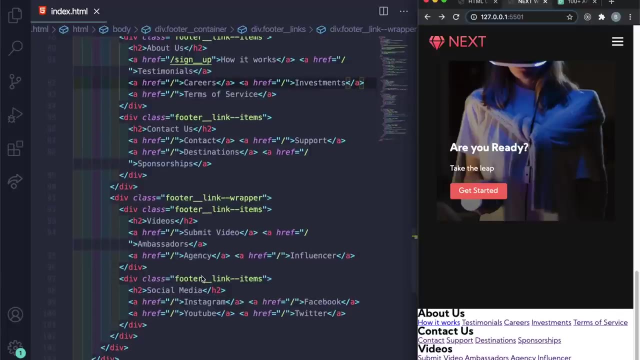 corner here. come on with us, cool, there we go. hey, yeah, finally, but iDIM, it actually fits. i think i misspelled this one- invests, let's see here, save it. and now we have everything different now here. so that's pretty much what i got going here and basically for the 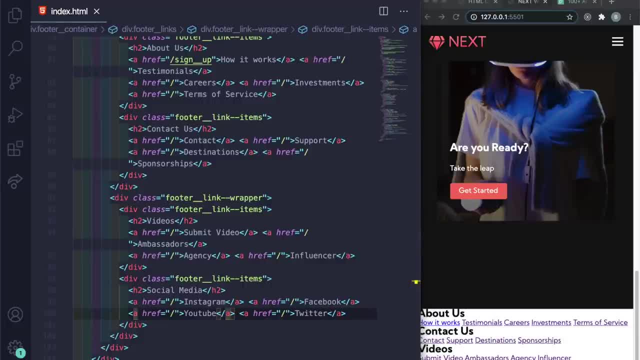 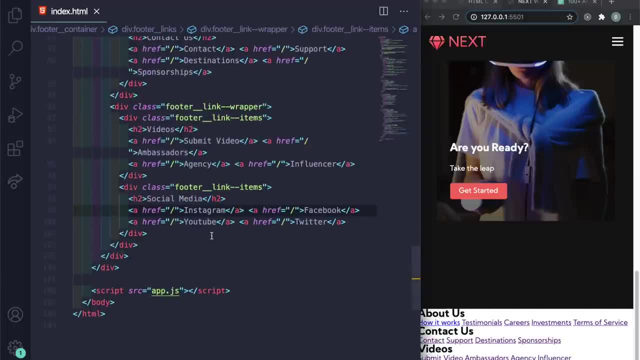 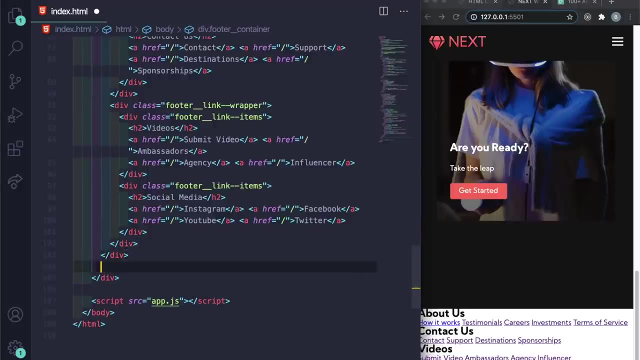 last one. you can change this too, but again, it really doesn't matter, it's just uh, you can name it whatever you want. so now after this: so let's see we have, let's see where is the footer links. so i want to go. so the second to last div: press enter. and now we're going to create these social. 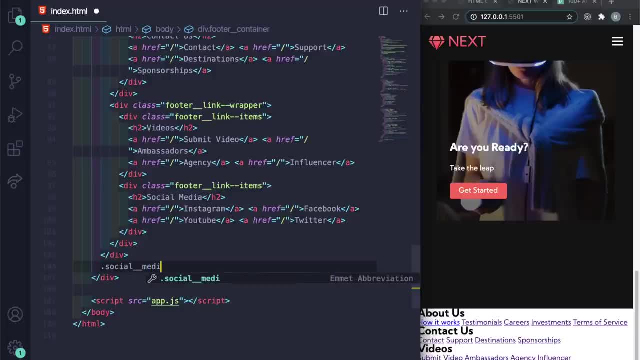 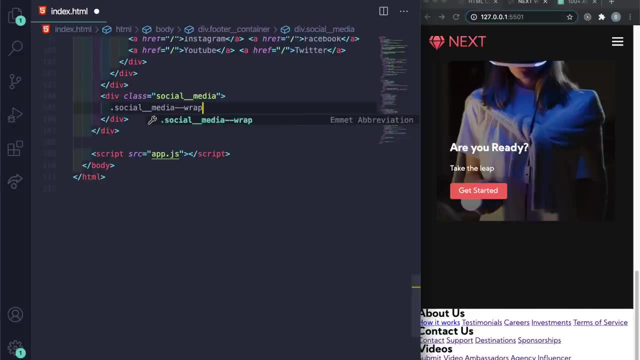 media. so let's do dot social underscore, underscore media press tab. and then let's just do dot social underscore, underscore media dash dash wrap. and then here i'm going to say dot footer- underscore, underscore logo. and then let's do a tag and let's just say hashtag: footer- underscore, underscore logo. 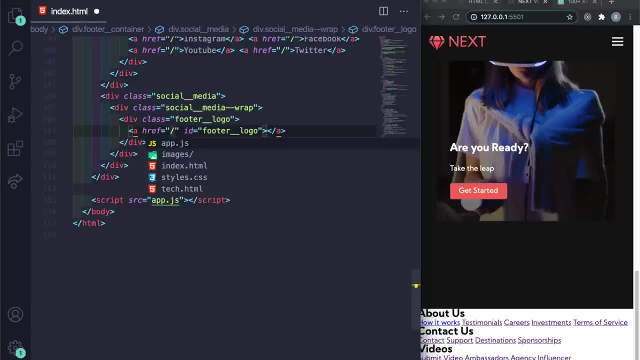 and then here i'm going to have the href- let's just put a slash and then for the a tag, let's just say i dot, fas, dot, fa, dash, gem press tab and then outside of this closing, i tag. and right before the closing a tag, let's just say next: and then let's do underneath this div here: 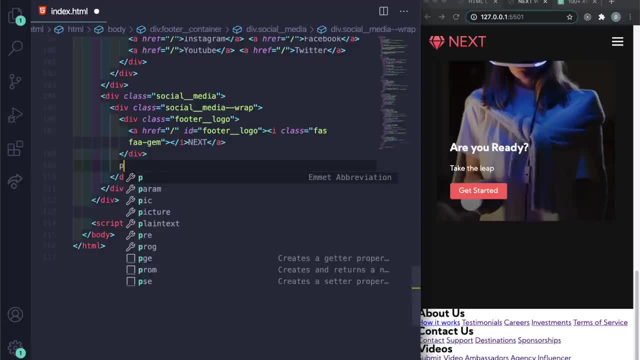 let's go ahead and just type in the p tag with the class of website, underscore, underscore rights, and then in here, let's just do: i have the copyright symbol, but you don't have to just say next, uh, 2020 dot. and let's just say all rights reserve. and i forgot. i forgot the shortcut key. 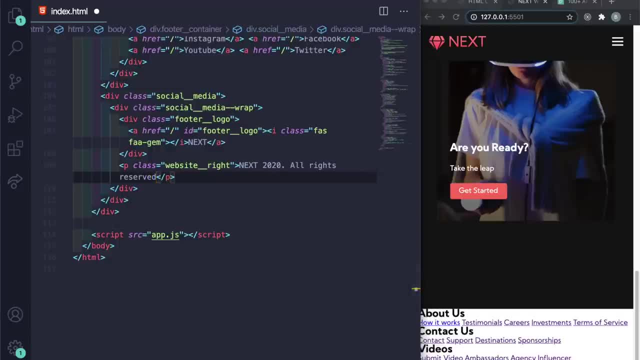 for the copyright symbol. so i'm just going to copy and paste mine, but i'm pretty sure i forgot the one via code. but you can literally just a quick search and should be able to show you. but again, it's not necessary and then let's do uh, underneath this p tag, let's do dot social. 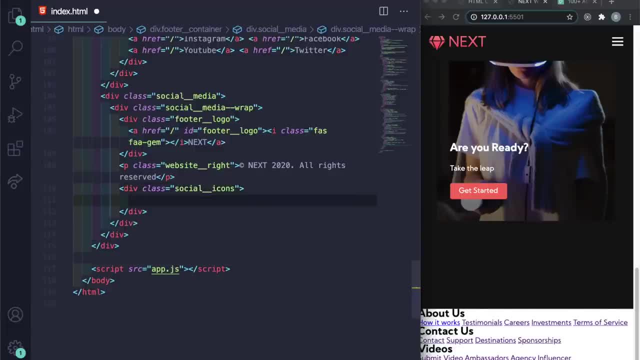 underscore, underscore icons and then in here let's do a dot, social underscore, underscore icon: dash, dash, link href. let me just put a slash and then let me go inside of the a tag and then i just put in this. so inside here let me just say i dot, and let's do fab dot, fa dash. face book press tab and let 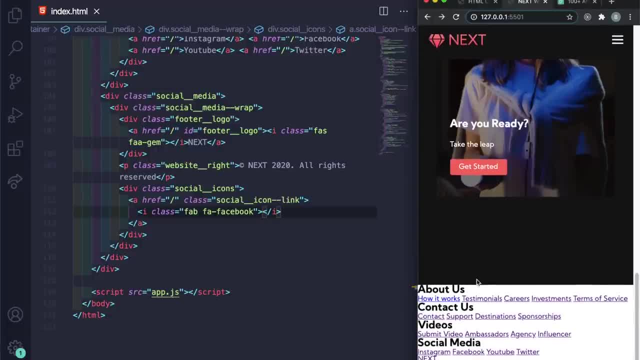 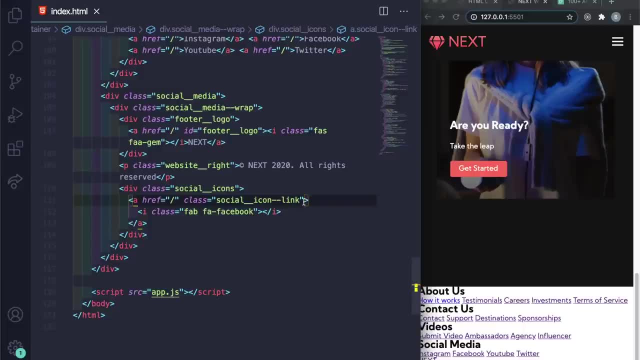 me save this and this should show us a facebook icon, and then let's do a slash and then let's do icon down here, which you can see very tiny, and then in the a tag, let me just finish stuff up and let me just say: um target equals quotes, and then let's just say: underscore blank. so this makes it. 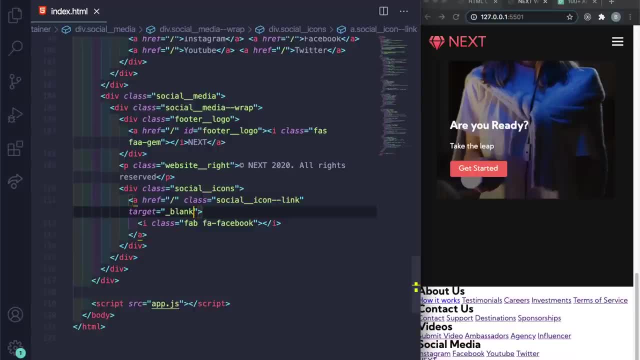 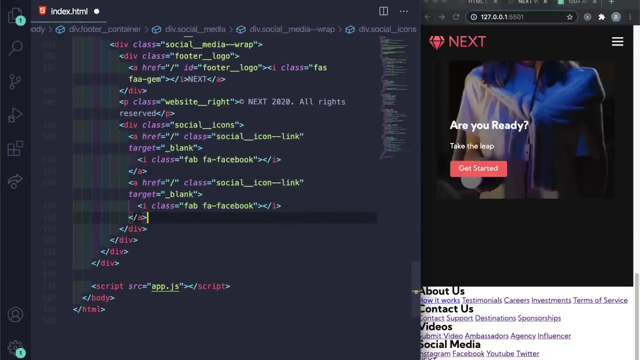 where you can open this in another browser. so let me just save it here and then let me just go ahead and just copy this stuff here. so let's copy this and then simply paste it under. so here i'm just going to say: paste here. so that's essentially instagram, and then let's do another one: enter. 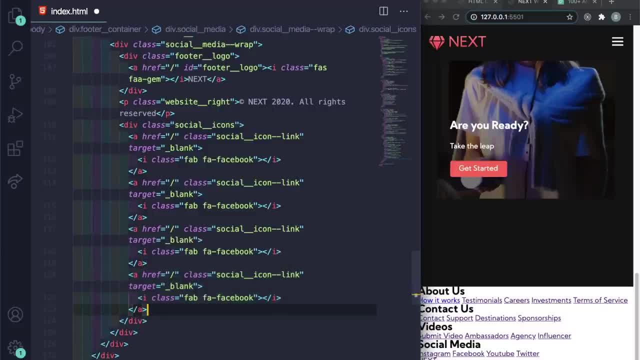 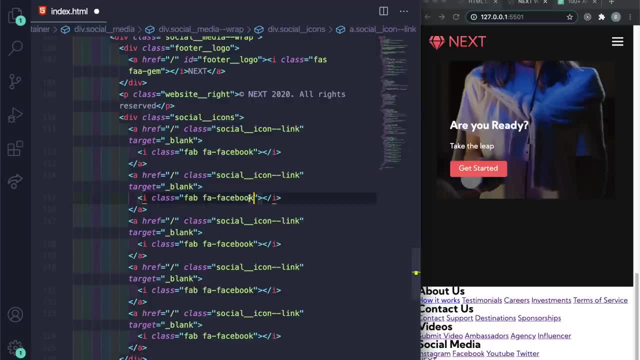 this would be: uh, twitter, enter linkedin and youtube. so now let's go and edit all that stuff. so we have um here. second one is instagram and all the icons. they're the same minus the social main, so you can just change this whatever you want to, so let's just say twitter. 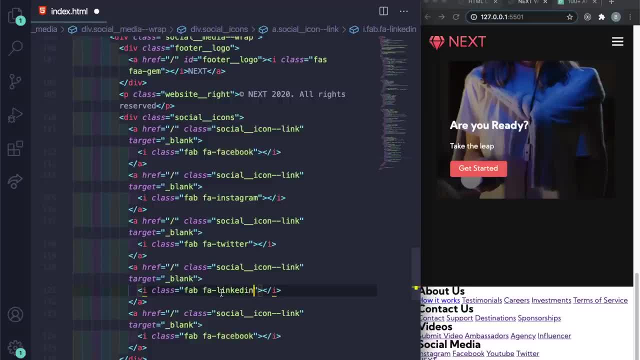 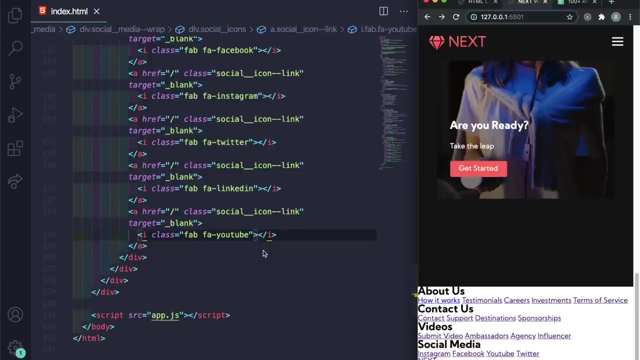 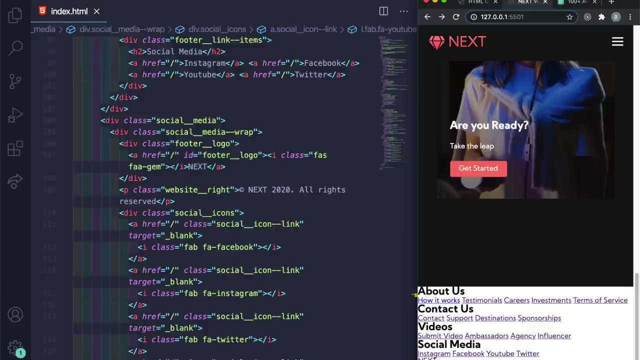 let's do um and and then let's do: uh, let's see youtube, save it there, and i can see we have all the logos there. so that's pretty much the footers um html, and i think let me make sure. yeah, we're fine. okay, so now i'm gonna. 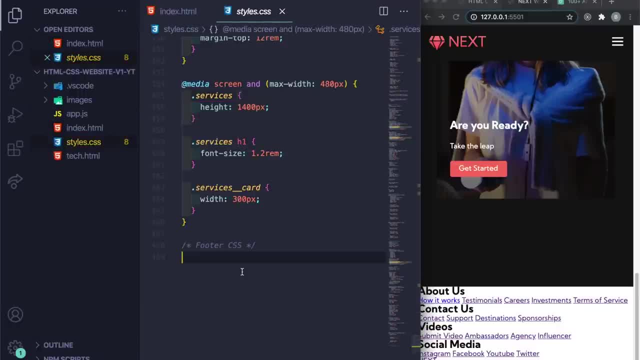 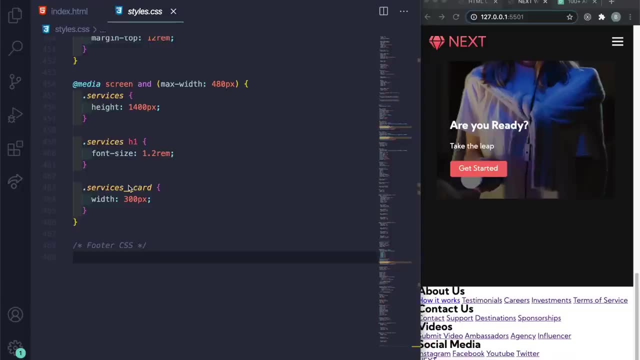 go command b: now let's go edit these styles. so here, close this back out and let's start editing the footer styles, and then we can call it a day. so now let's do dot, footer, underscore, underscore, container. i'm gonna say background dash color to be hashtag one, four, one, four, one, four. let's say: 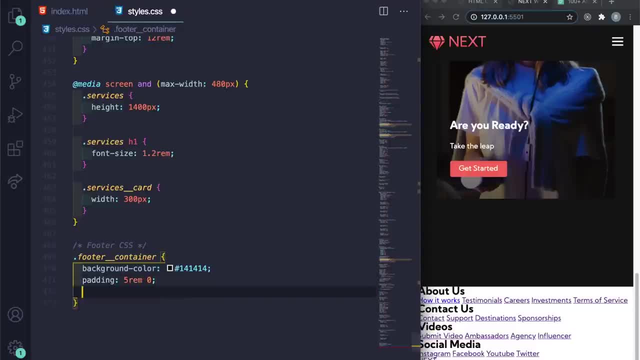 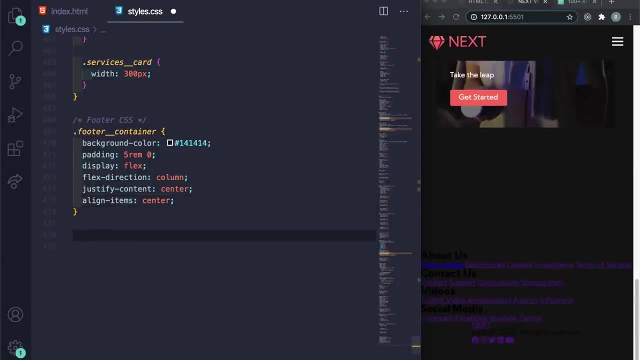 padding to be, let's do five, ram zero. let's do display to be flex, flex direction to be column, uh, let's do justify content to be center and then let's just do all see align items to be center. so let's see, so we got some, some movement going on and now let's target the hashtag footer. 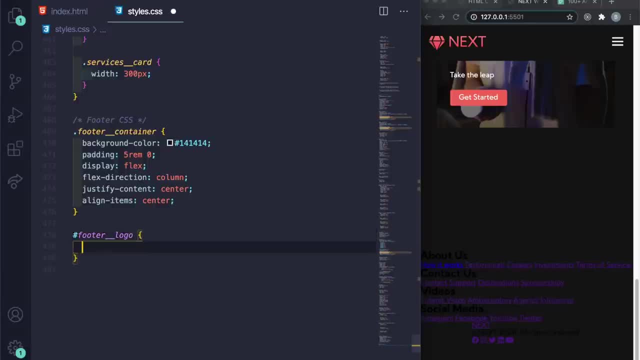 underscore. underscore logo. let's just do color to be as i have, f, display to be flex, align items to be center and then let's just do all see: align items to be center. so let's do point items to be centered, cursor pointer. let's do text decoration to be none and font size to be. 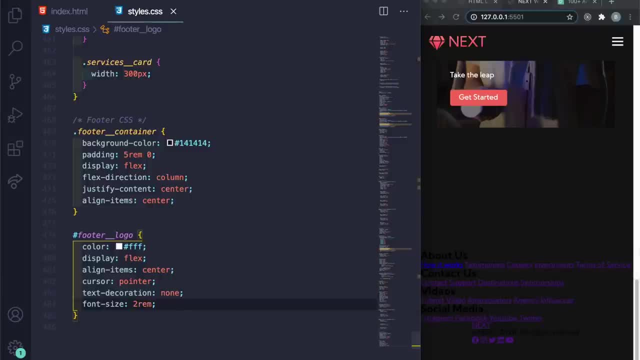 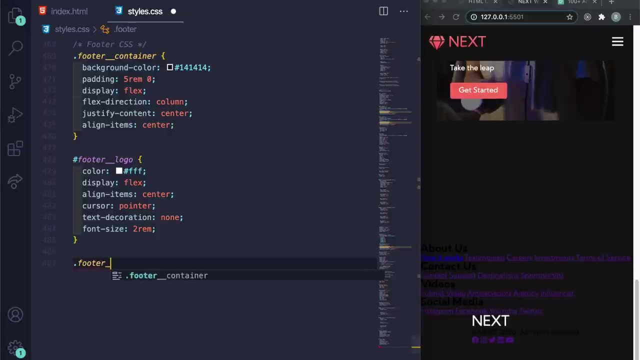 two rev. let me just scroll it up here. and then let's do dot, footer underscore links. let's do a width of a hundred. let's do max width to be a thousand pixels, display to be five hundred. and then let's do a stop here and then let's do techniques, actions to be none and font size to be 100, to be 2rem toast, and then do you score that up here and then let you do footer underscore link. let's do a width of 100%. let's do max width to be 1,000 pixels displayed. i'm just going to continue to go through what i got here. let's open the extension fx. it's just going to give it a moment to start the text window. let's just go through this picture and take note what the does it give for the Primary Touch. I just want to make sure that. 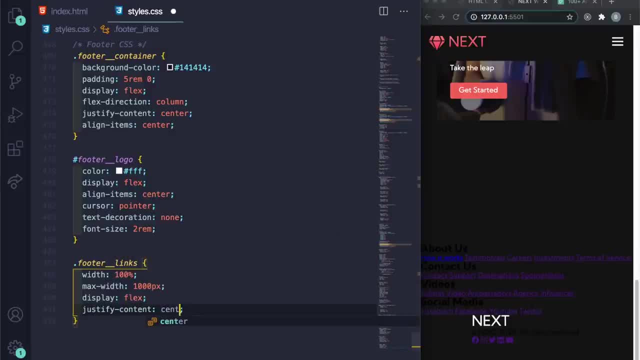 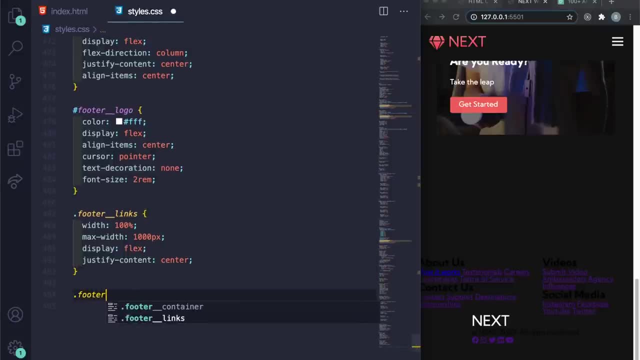 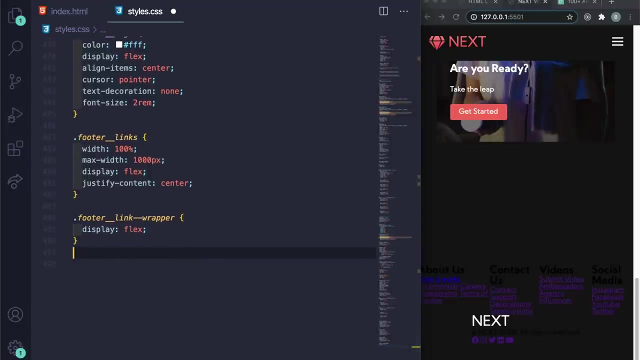 is flex and then justify: content is centered. so we got some stuff happening here, and now let's do dot footer, underscore, underscore, link, dash, dash, wrapper, and let's just say display to be flex, so you can see here. now that brings them over to the side, and now let's just do under here: dot footer. 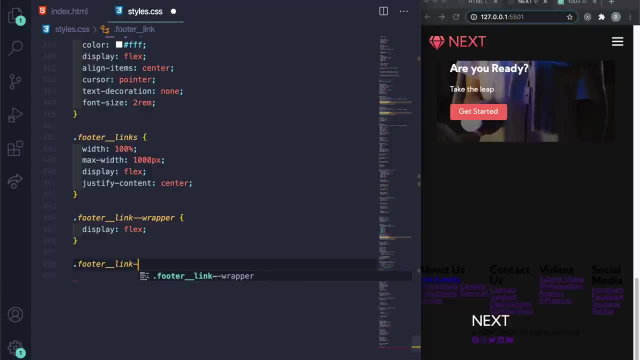 underscore, underscore, link, dash, dash, items, and let's just say display to be flex, then under here let's do flex direction to be column and let's do a line items to be flex starts, and then let's do margin of 16 pixels, let's doctor, do text, a line to be left with to be 160 pixels and box sizing to be border box. save that there. 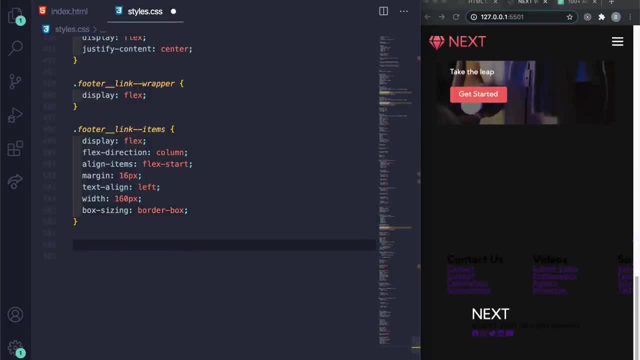 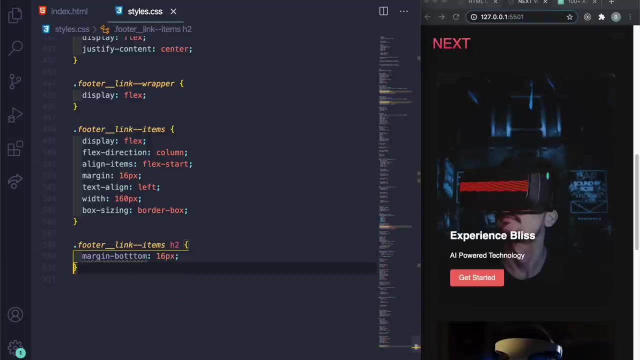 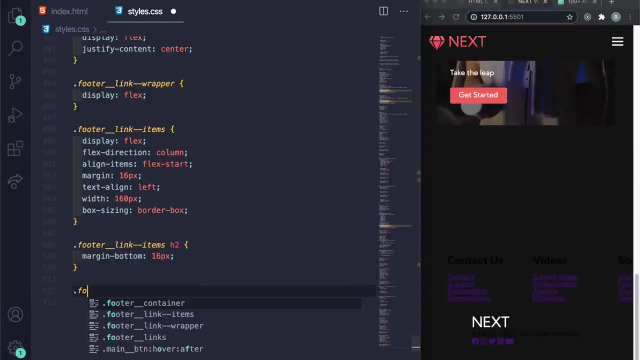 and scroll down. and then let's do dot footer underscore, underscore link dash dash items of h2. let's do margin dash bottom to be 16 pixels- I put two teeth Macy's here, okay. and then let's do dot footer underscore, underscore link dash dash items and greater than h2. and this is gonna. 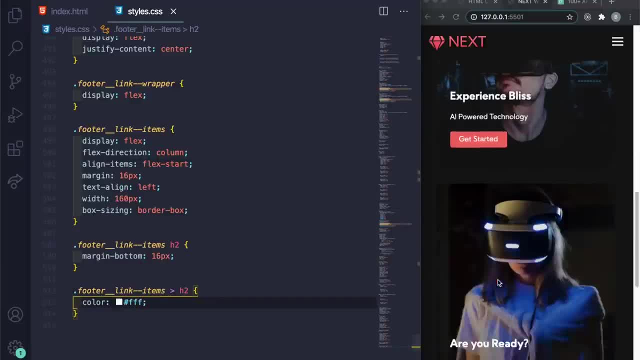 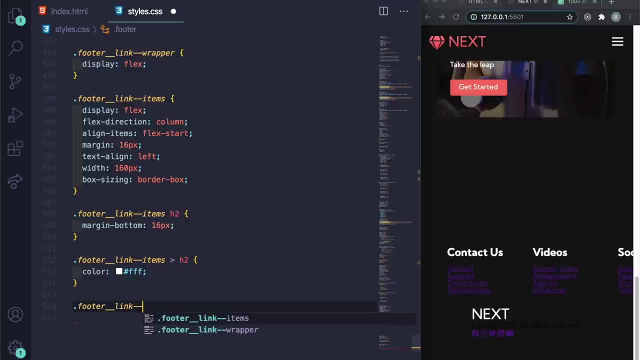 just target the hashtag out of F. so now we're targeting essentially, the h2 is there, and then let's do dot, footer, underscore, underscore, link, dash, dash, items a, and it's gonna say color hashtag, FFF, text deck or ration is going to be none and then margin dash bottom is going to be 0.5 round. let's go. 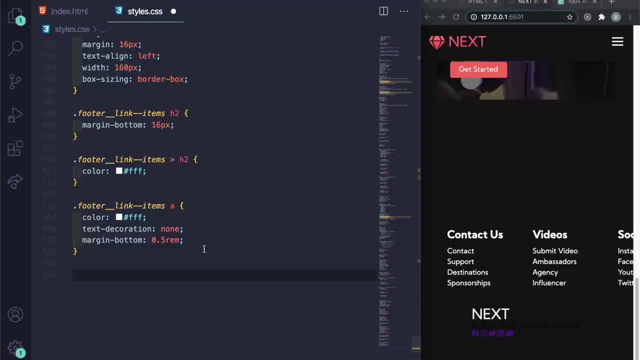 down here. so now I've got some more color action here, and now let's do: on dot footer, underscore, underscore the link, dash, dash items, a colon hover, let's say color equal to hashtag e99, e99, and then transition is going to be 0.3 s ease, dash out. 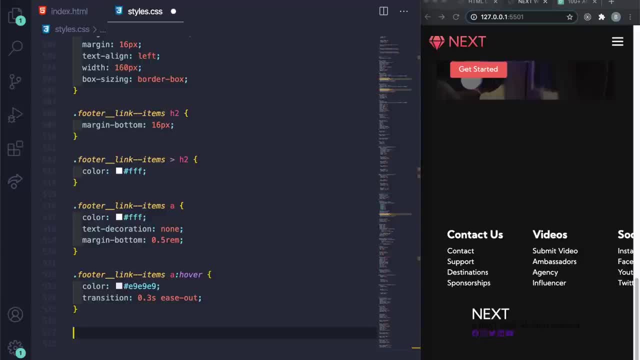 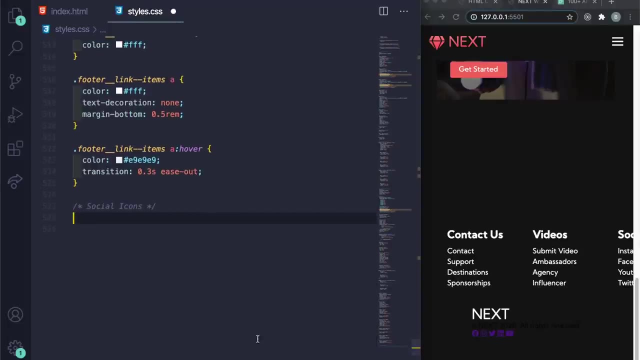 so here and then let's do: um, this is social icon, so essentially the bottom section now. so let's just comment, say social, social icons. then let's go up and let's do the social on a across here fish icon, dash, dash link. I forgot the peered in the front, so still done here. 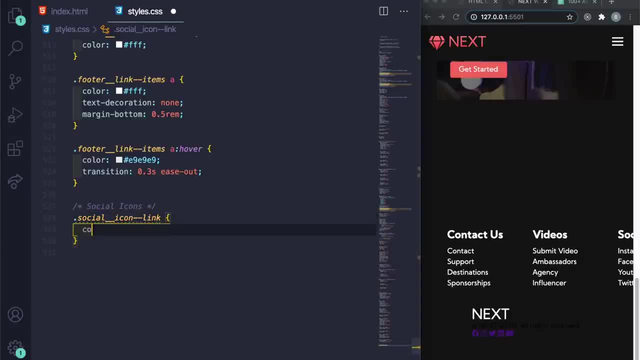 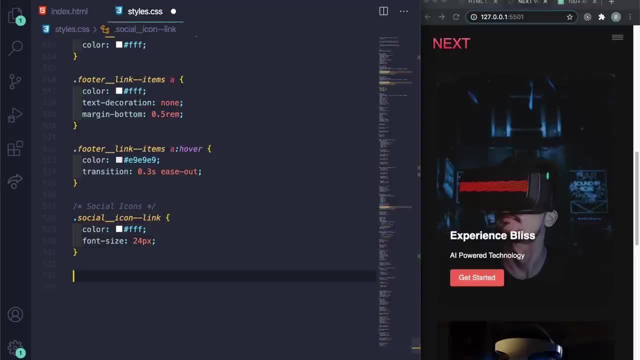 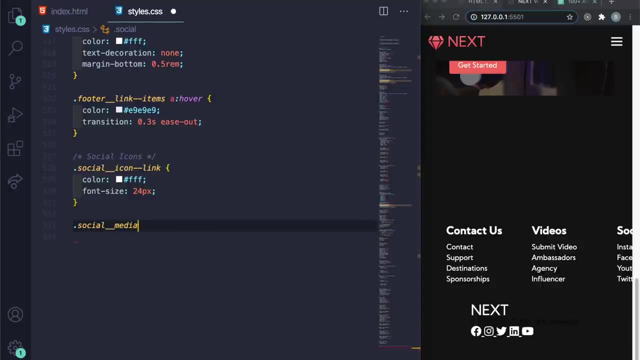 dot. put dot District dot here. let it just a color hashtag: fFF- and then I font size to be 24 pixels down here, and then let's do dot so and you're just saying max dash width to be thousand pixels and then width to be a hundred percent. 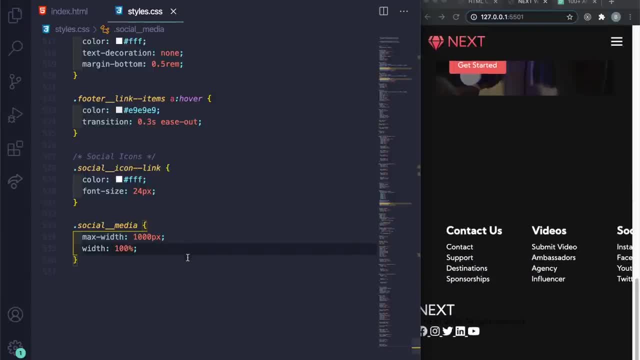 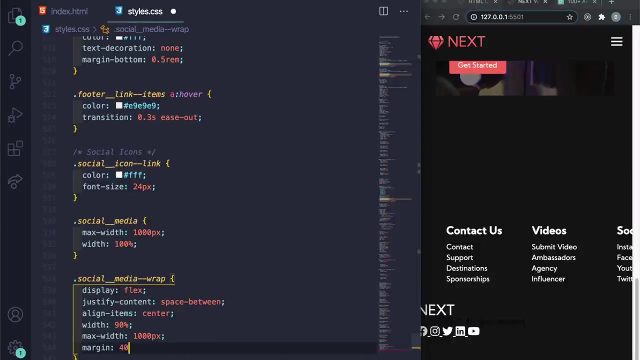 and then under here let's do um dot, social, underscore, media dash, dash wrap. let's say display flex, justify content space between. let's do a line dash can't type right now, to be center with, to be ninety percent, max width is one thousand pixels and let's do margin forty pixels, auto zero on toe, save that. 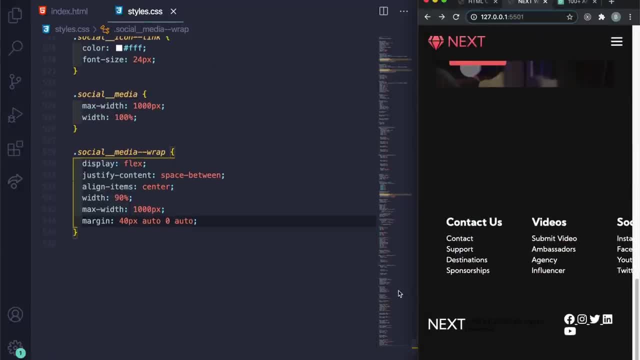 let's see how that looks now. okay, look a little better. and then let's do. let's see you got raps, let's do dot social on underscore: underscore icons. now. display is flex. justify content space between align dash items Center and then with 240 pixels. so we got some space in here. 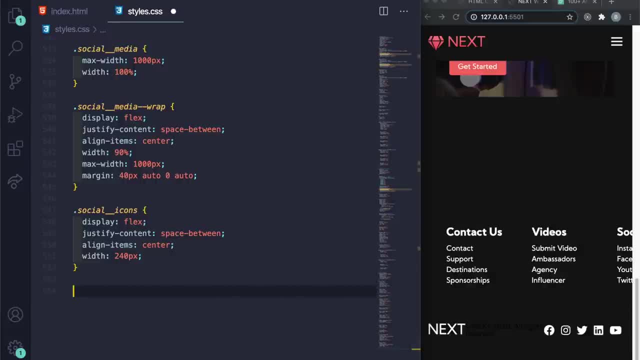 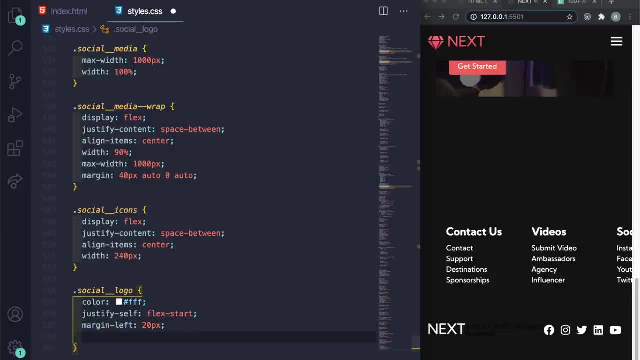 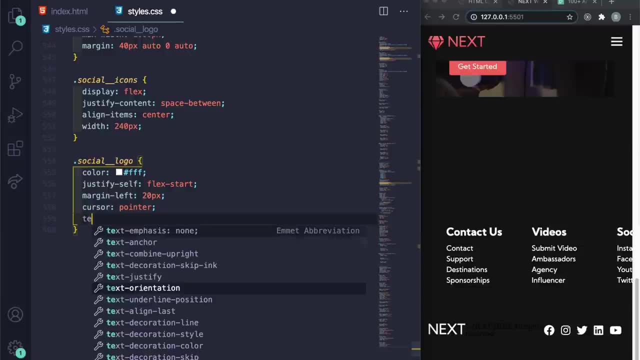 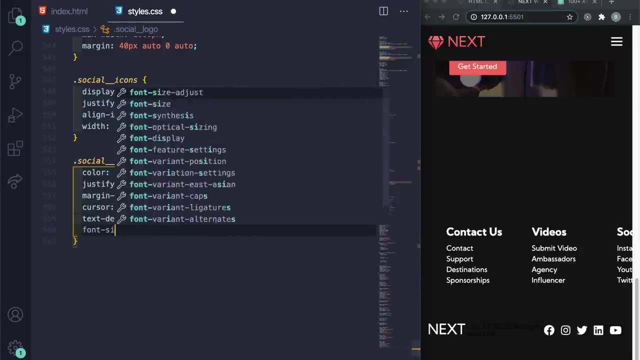 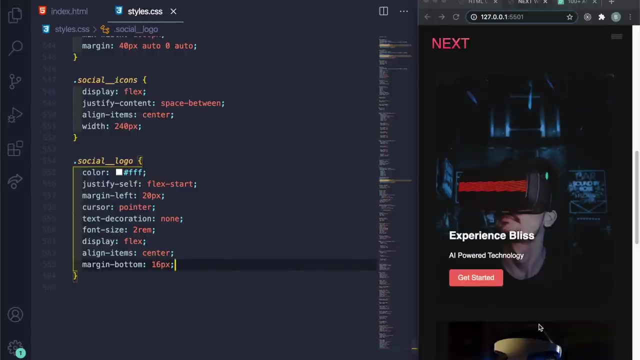 margin dash left to be 20 pixels. cursor pointer and let's do all the text decoration to be none. let's do font size to ram display flex, align items to be center and then margin bottom to be 16 pixels. let's see, we are going on right now. so. 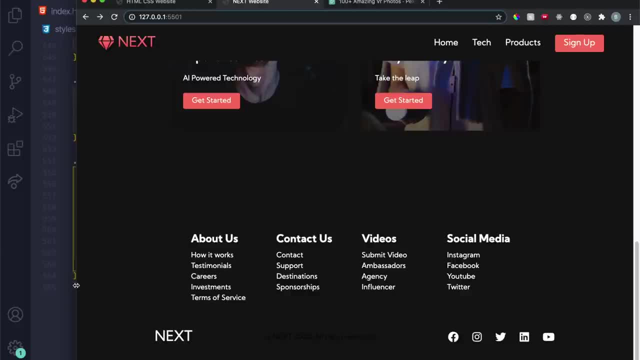 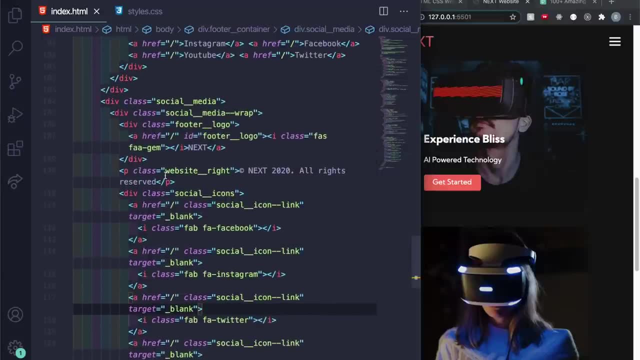 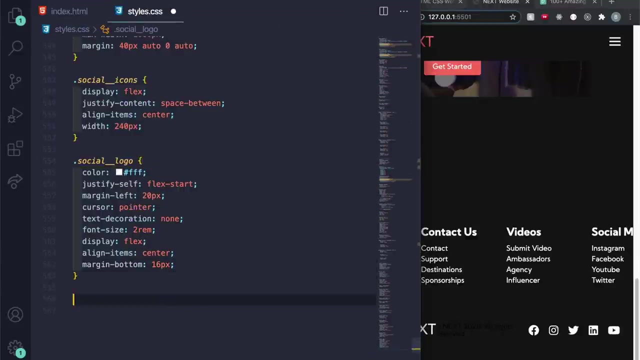 I think I cannot even- you know me chicken- even have the logo in here. sure, that's why misspelled should be the actual, the neck should be FAS dot F, a dash gem. so now we have little diamond. okay, now let's make sense. so now let's. 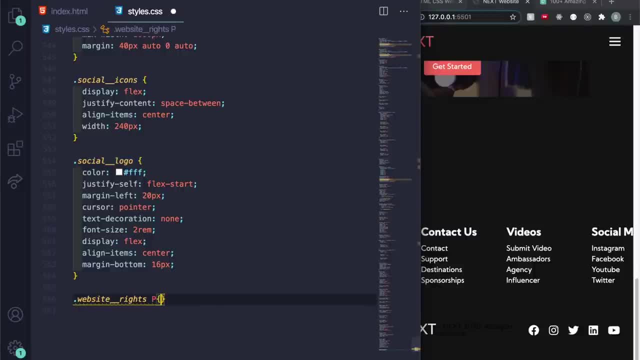 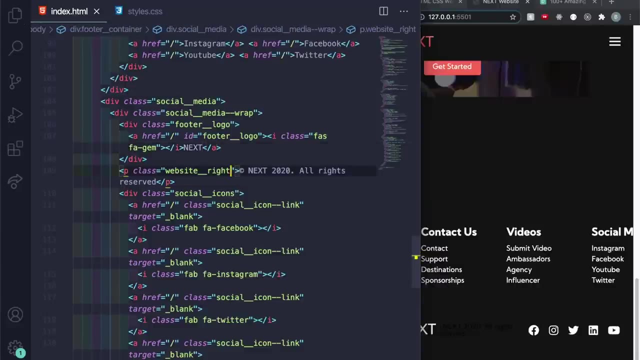 just the last one. that website on. it's gonna throw rights you, and let's just say color hashtag FF. so it's not changing. what the heck? so let's go back right, so this should be website rights. and now we got the color changing. perfect, all right, so now. 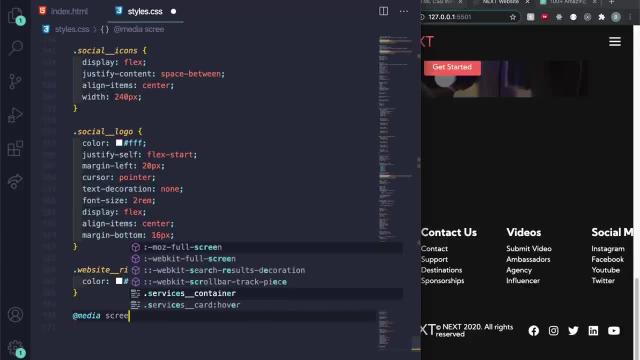 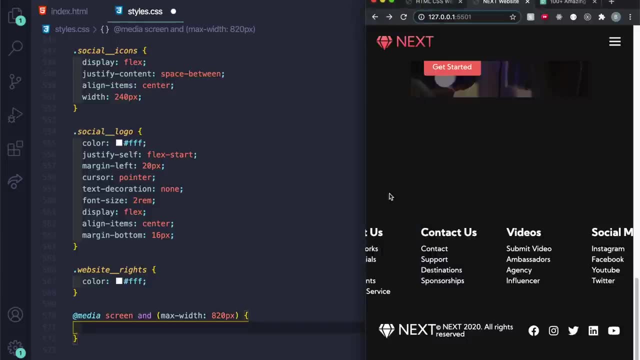 let's do the media creators now. so let's do add media screen and max width of 820 pixels, color race here, and let's just show you what we got so far. it looks like like this, but we need that to be responsive, so let's go ahead and 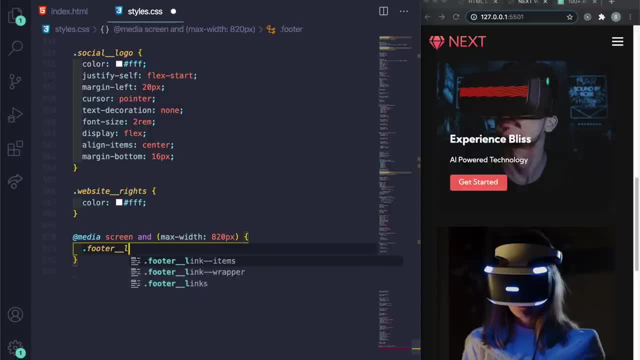 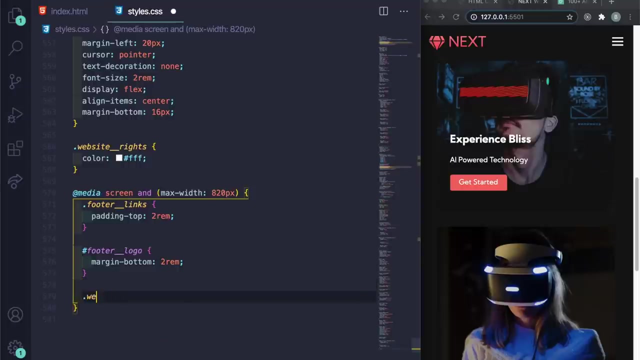 dot footer underscore, underscore links and that should be padding dash top to rem. and let's see dot fushy hashtag footer, underscore, underscore logo, margin dash bottom to be to rem. and then let's do dot websites underscore rights and let's just do margin dash bottom. 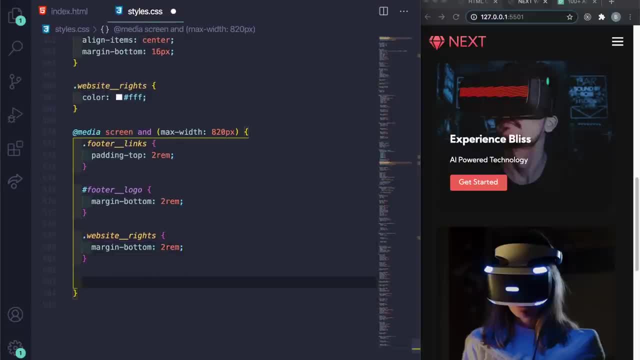 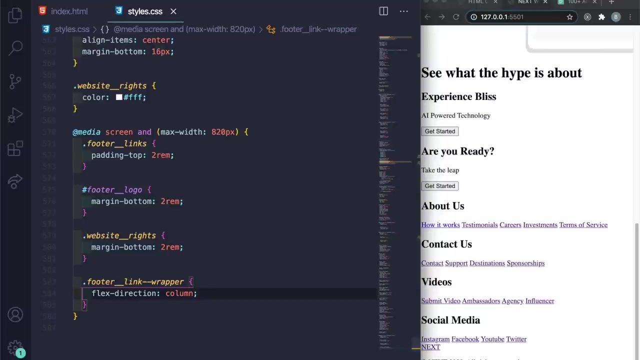 of to round here and let's do dot footer on this- going to score a link, that dash wrapper- and let's do flex dash direction to be column. okay, yeah, I'm tripping out what happened. okay, is it working? okay, cool, and then under this, let's. 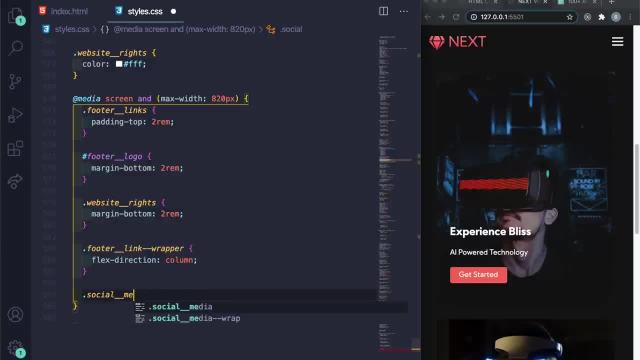 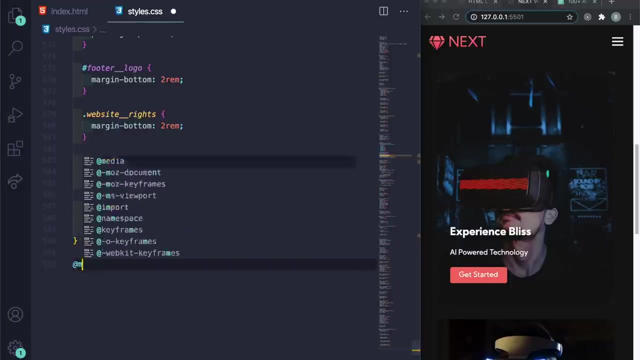 do dot social underscore, underscore, media dash, dash, wrap. and let's do flex dash direction column as well. and then let's go under here and let's simply add this line at media screen and max- I'll see me screen and max dash with 480 pixels- and let's do dot footer underscore, underscore, a link: dash, dash.